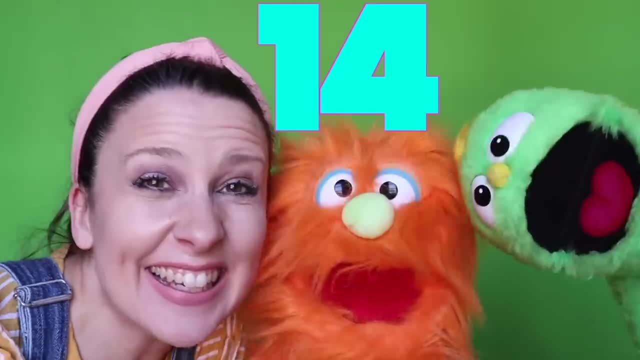 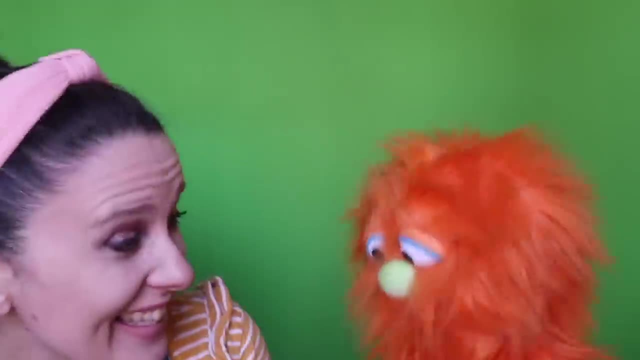 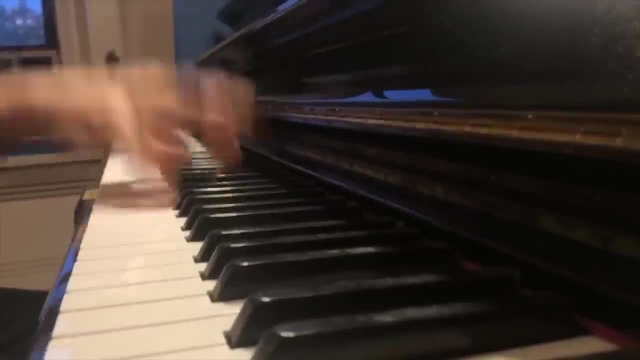 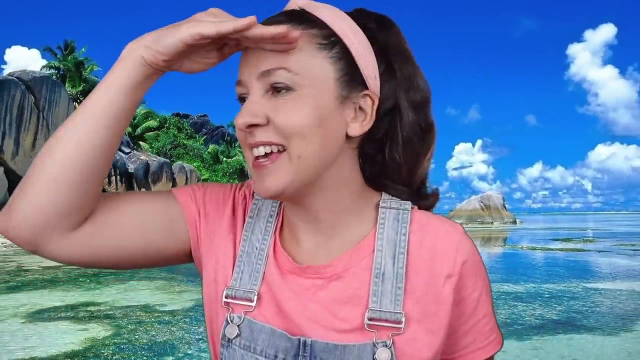 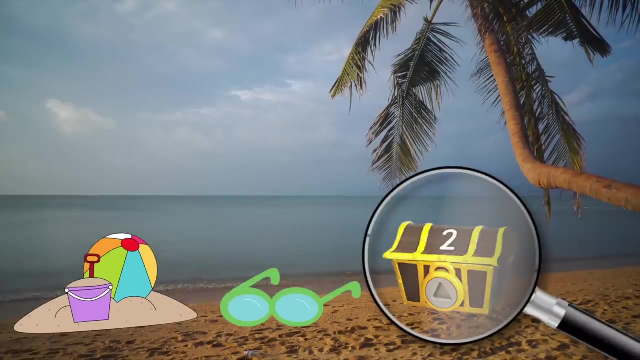 One, two, three, four, five, six, seven, eight, 16,, 17,, 18,, 19, 20.. Okay, let's walk around and look for another treasure. Do you see any more treasure? Oh, wow, I think you found it. 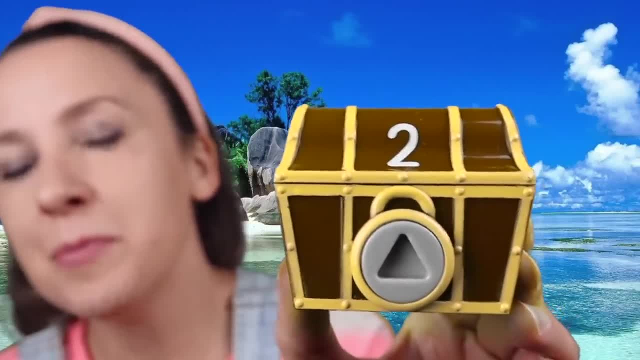 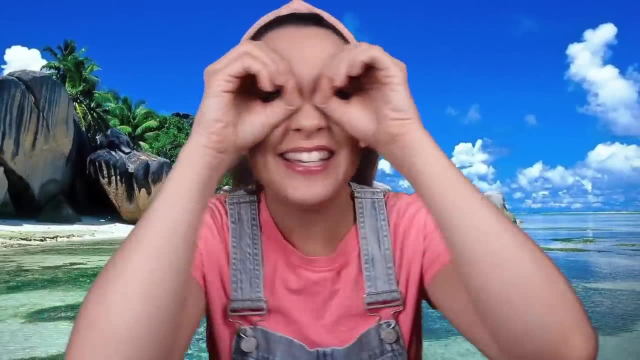 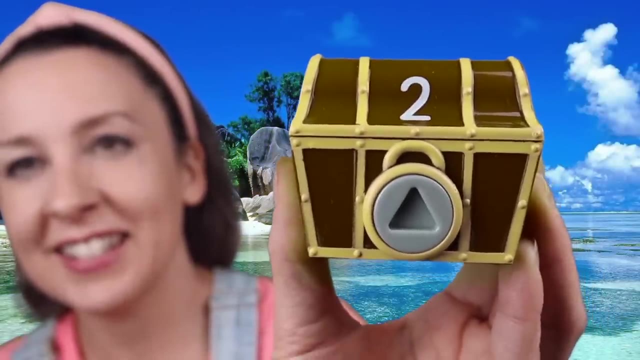 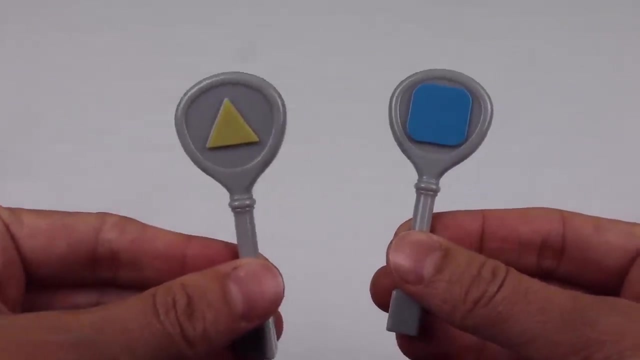 What color do you see on the brown treasure chest? Yeah, I see yellow. What number do you see on the treasure chest? Yeah, it's a two. To open the treasure box, with yellow on it. should we use the key with the yellow triangle or the key with the blue square? 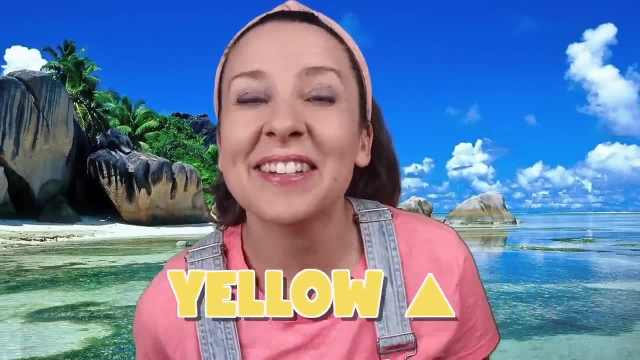 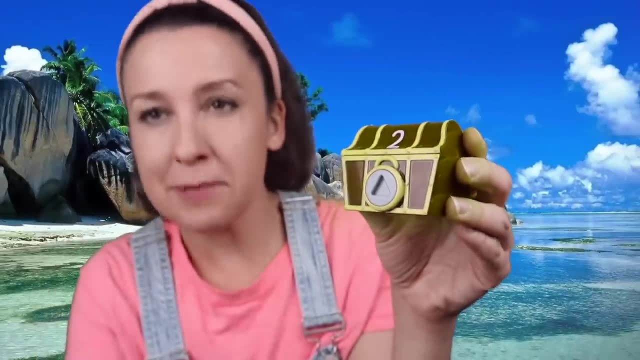 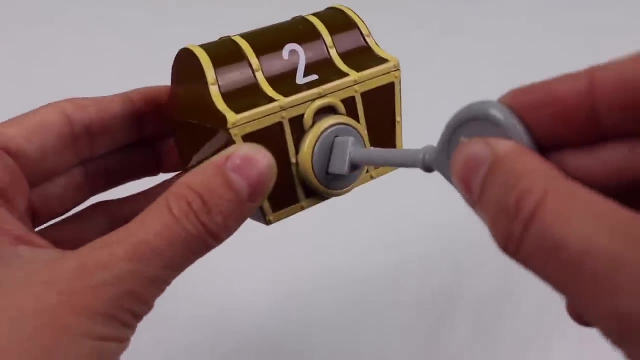 Yeah, let's use the yellow key. If we try the key with the blue, it doesn't work. That's not right. We need it to match, so we use the yellow key. Okay, let's put the key in and turn it. 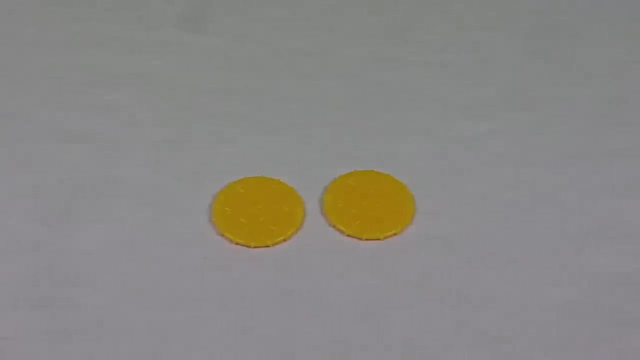 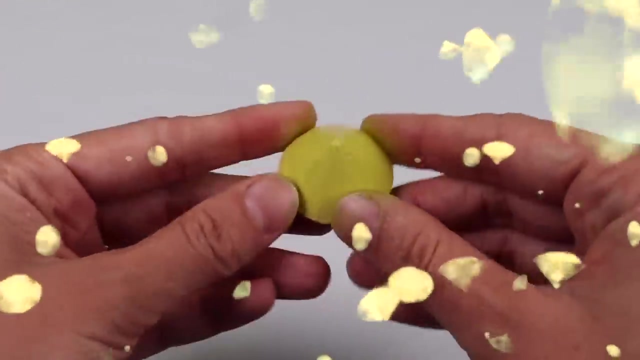 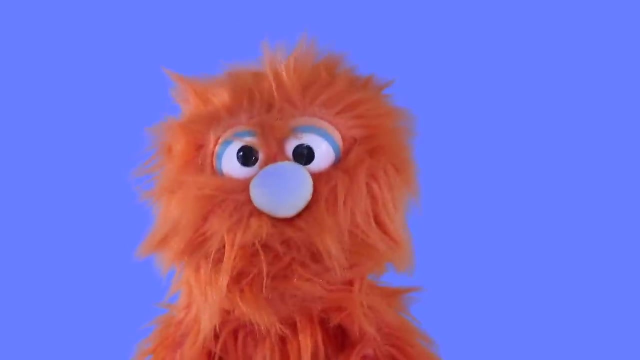 Wow, How many coins. Let's count One, two, Two, Two coins And what's the surprise? Wow, It's a beautiful gem, So pretty. Hi everybody, it's Herbie, Can you count with me? Here we go. One, two, three pickle. 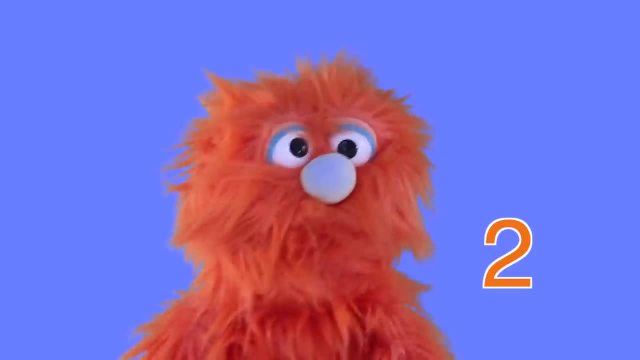 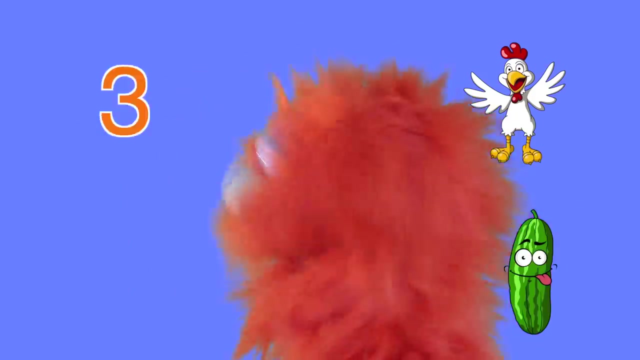 Pickle, That's not good. One, two, three chicken. Chicken, Chicken, No, that's not it. That's not it. One, two, three banana Banana. One, two, three chicken. One, two, three pickle. One, two, three banana. 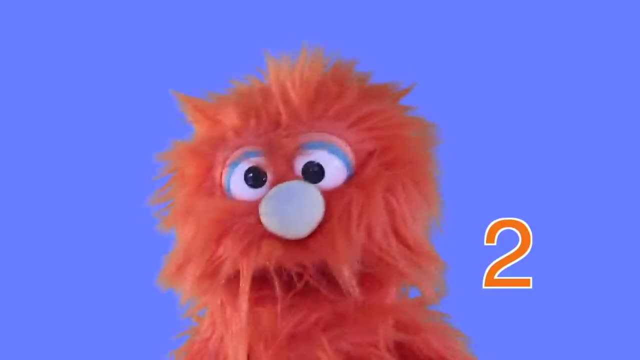 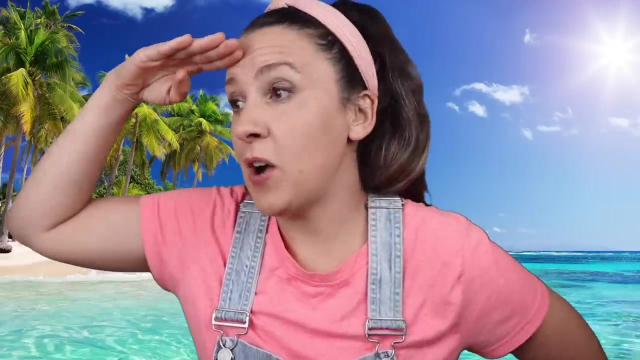 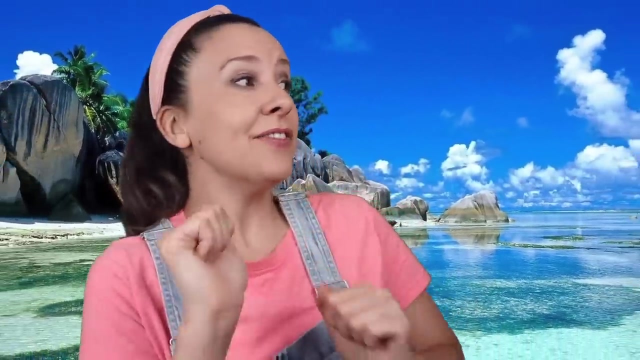 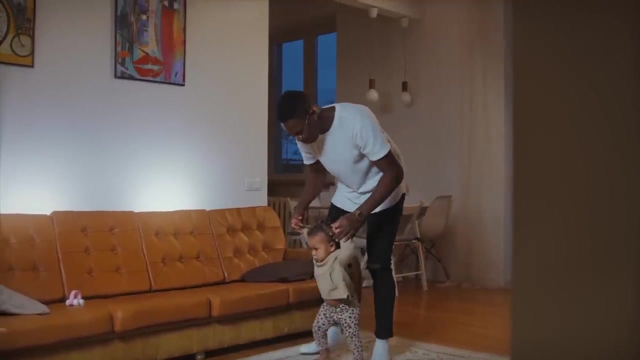 I'll get it this time. One, two banana. Oh, now I forgot three. Let's keep walking around the island and looking for more treasure. Walk around with me and look for treasure. Hmm, let's keep walking, Do you see it? 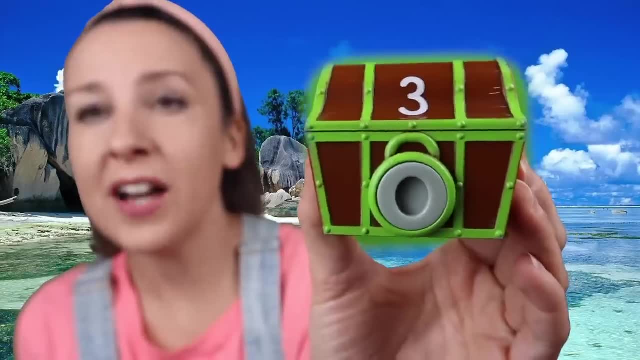 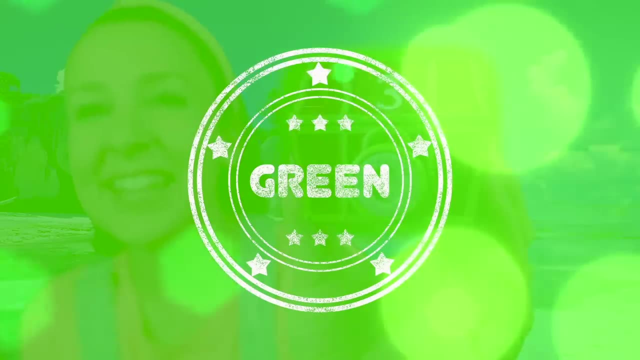 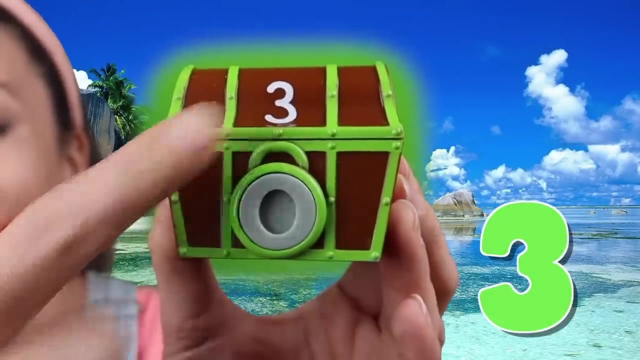 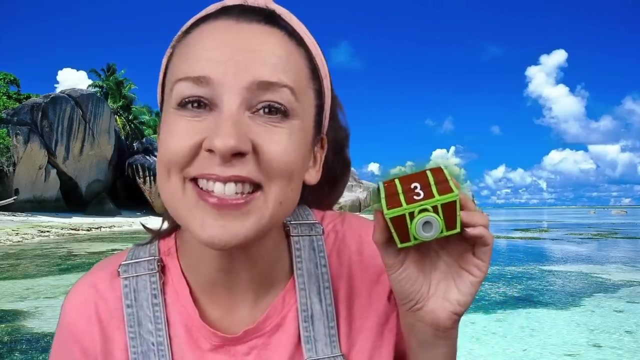 Yeah, I see it too. What color do you see on the brown treasure chest? Yeah, it's green. Wow, What number do you see? Three. Good job, Should we open it? Yes, Yes, please, Let's do it. 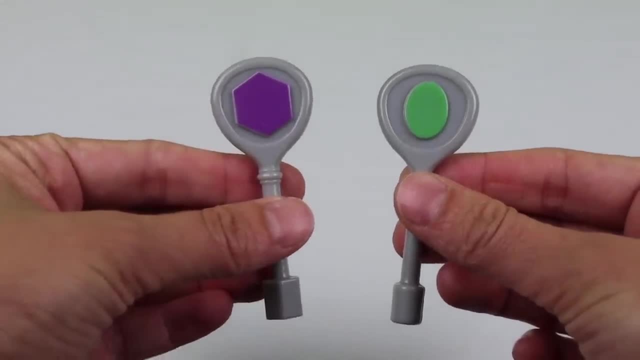 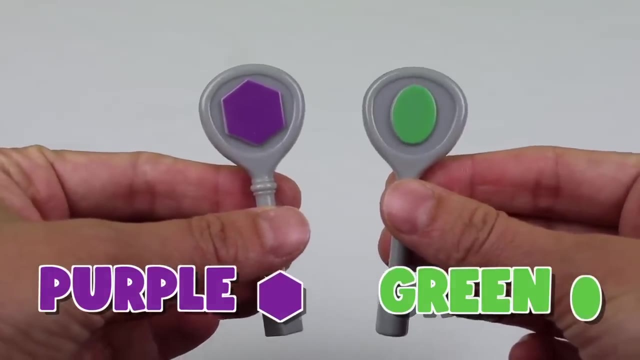 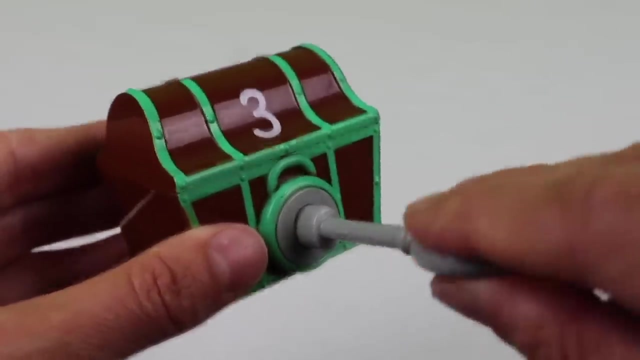 To open the treasure with green on it. should we use the key with the purple hexagon Or the key with the green oval? Yeah, the key with the green oval Say open, please Open, please. Wow. Let's see how many coins. 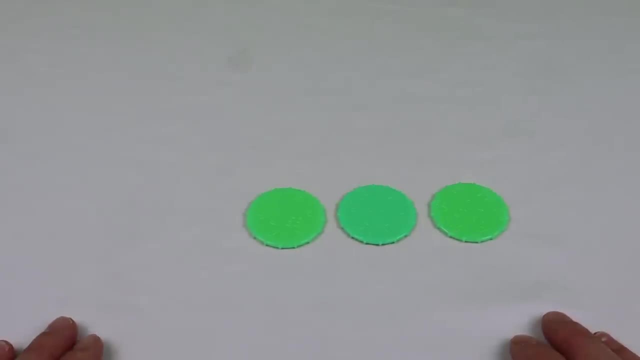 When we count, we don't say the next number until we touch the coin. One, two. oh don't say three until I touch it Three, Three coins. The last number we say is how many coins we have, Three precious coins. 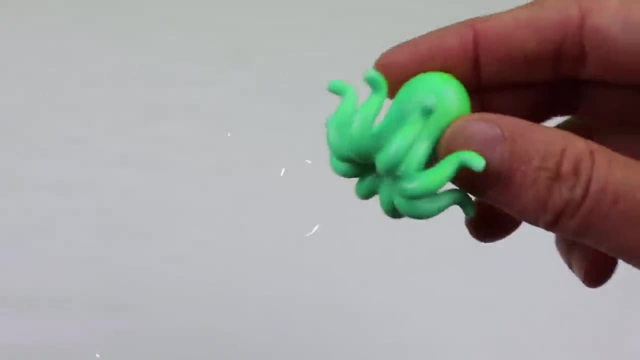 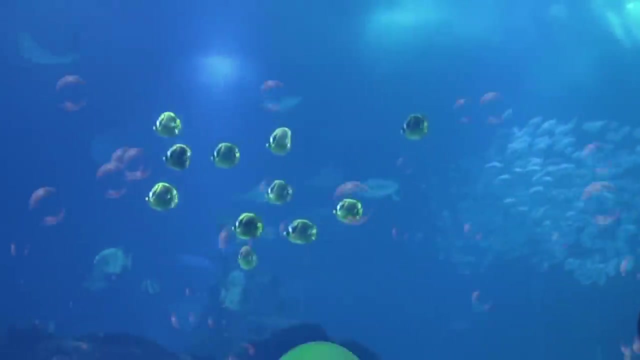 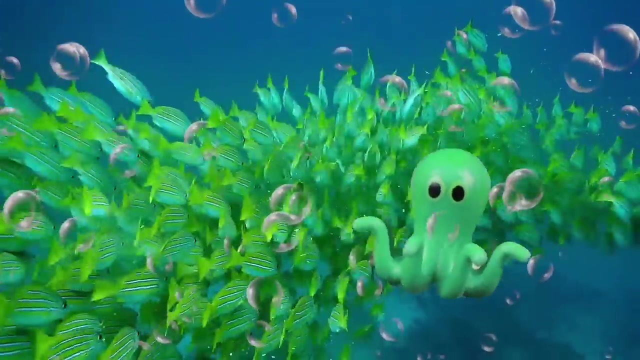 Let's see what the surprise is. Oh, how cute. It's a little green octopus. He's so cute. Hi, octopus, Can you say hi to the octopus? Hi, octopus, Hello, I'm going to swim. 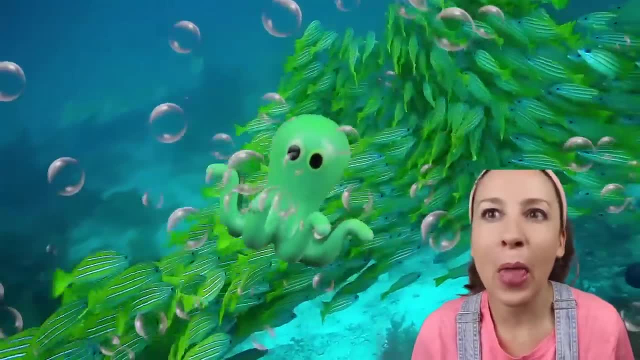 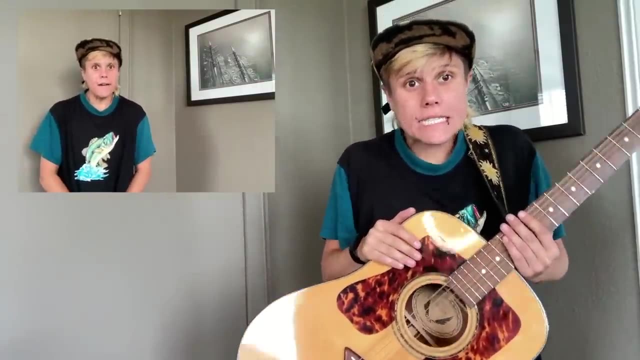 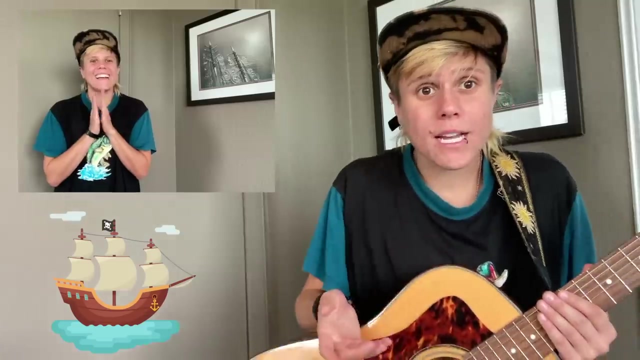 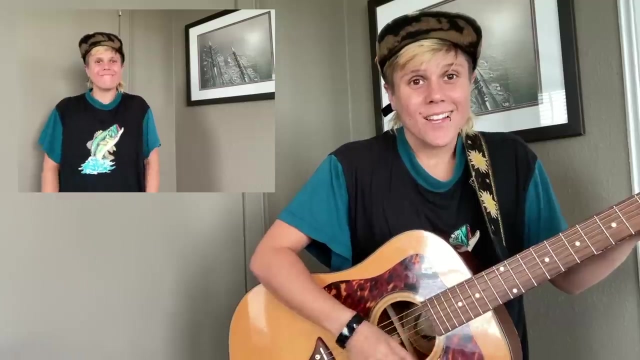 Can you do that? That's so silly. Hey guys, Could you help me sing a song about the deep blue sea? We're going to climb aboard a pirate ship. Maybe we can help the captain steer the boat. Are you ready? Twas a sunny day when I went to play down by the sea. 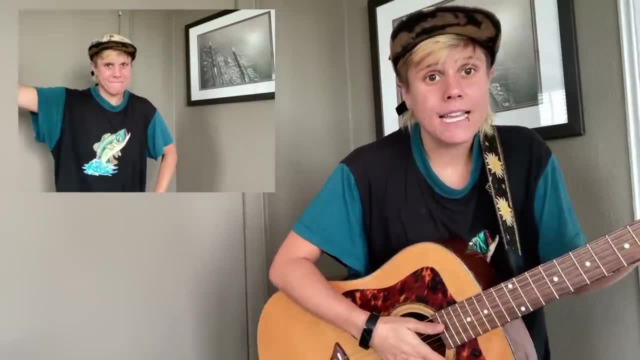 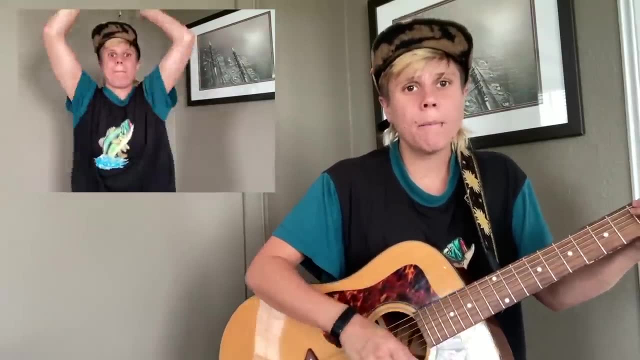 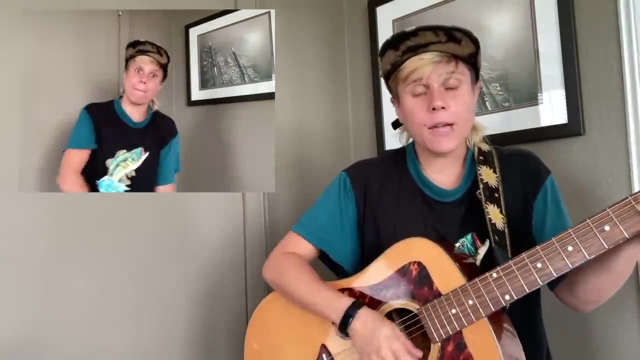 I climbed aboard a pirate ship and the captain said to me: We're going this way, that way forward, Backwards, backwards, up and down, up and down over the deep blue sea. Nice job, It was a windy day when I went to play down by the sea. 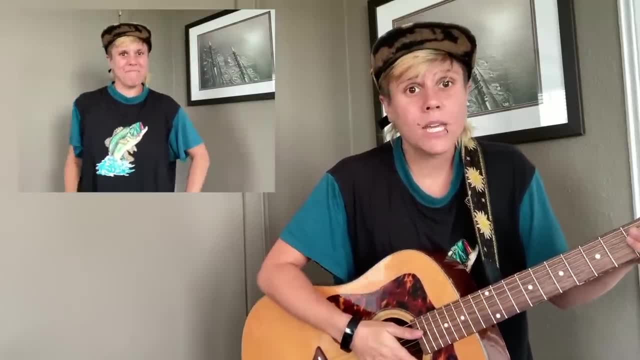 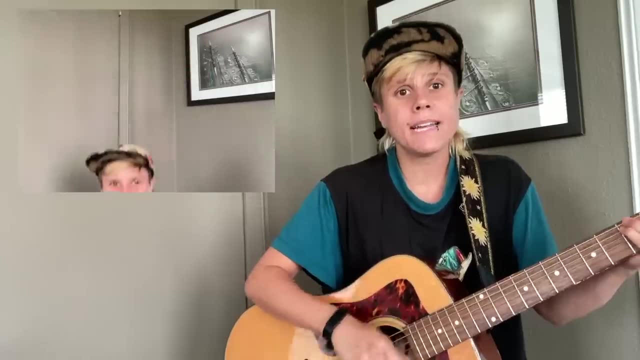 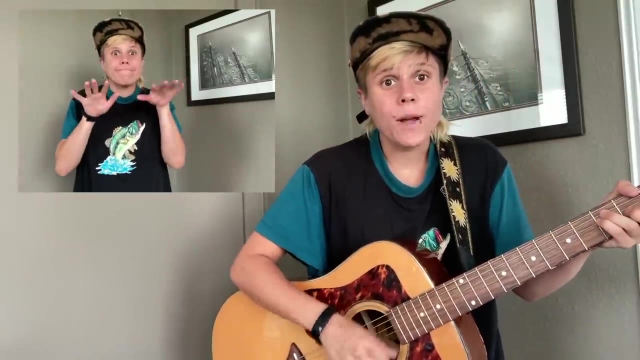 I climbed aboard a pirate ship and the captain said to me: We're going this way, that way forwards, backwards, up and down, up and down over the deep blue sea. It was a rainy day when I went to play down by the sea. 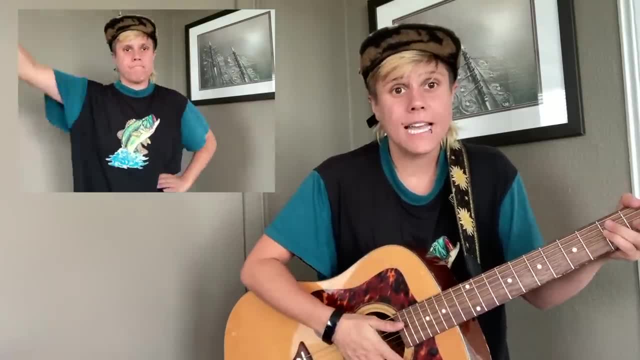 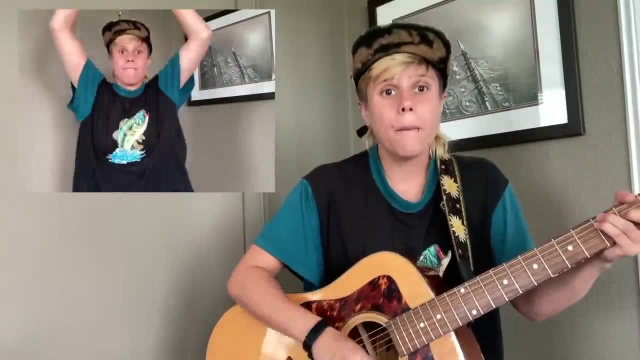 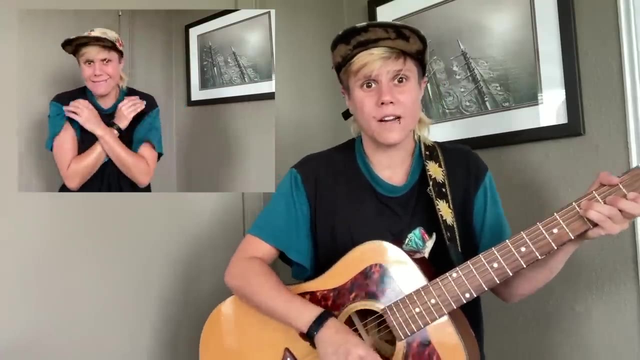 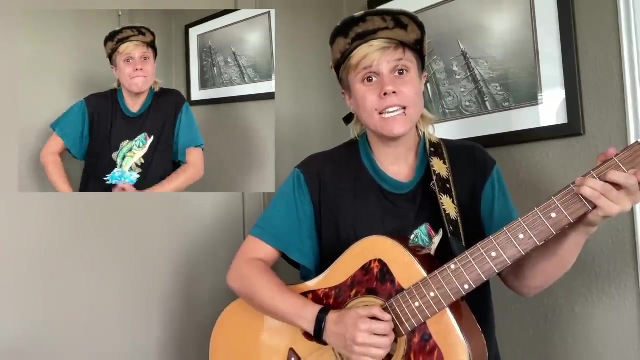 I climbed aboard a pirate ship and the captain said to me: We're going this way, that way forwards, backwards, up and down, up and down over the deep blue sea. It's getting cold out here by the ocean Was a snowy day when I went to play down by the sea. 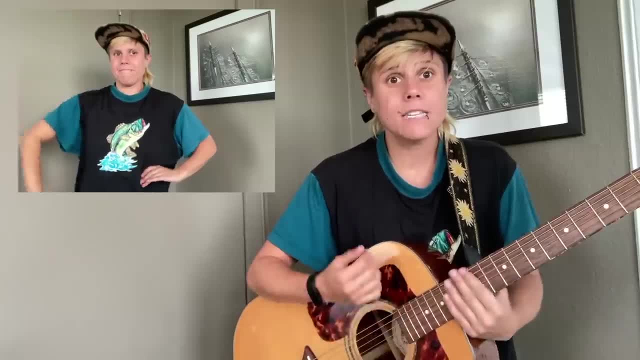 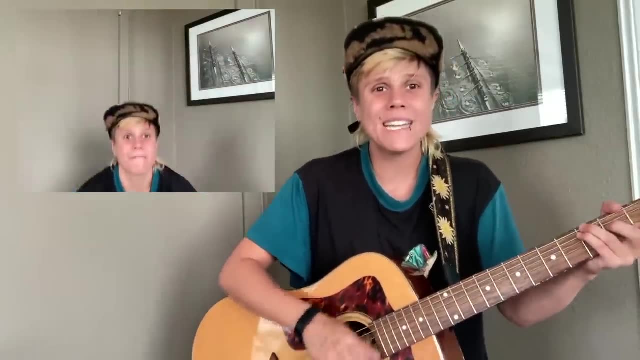 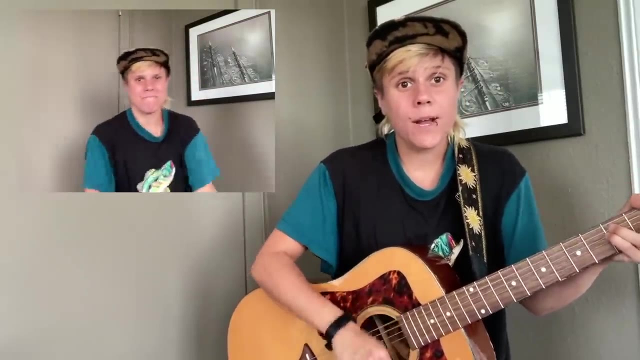 I climbed aboard a pirate ship and the captain said to me: We're going this way, that way forwards, backwards, up and down, up and down. over the deep blue sea Was a stormy day when I went to play down by the sea. 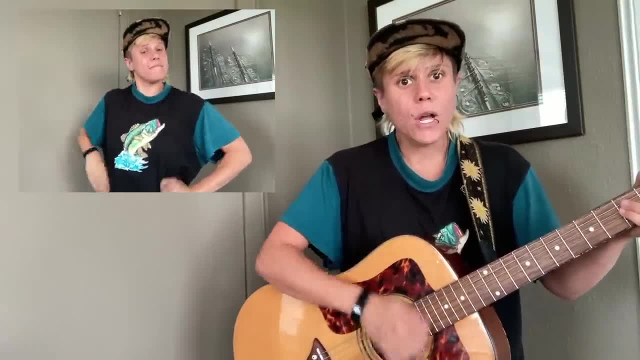 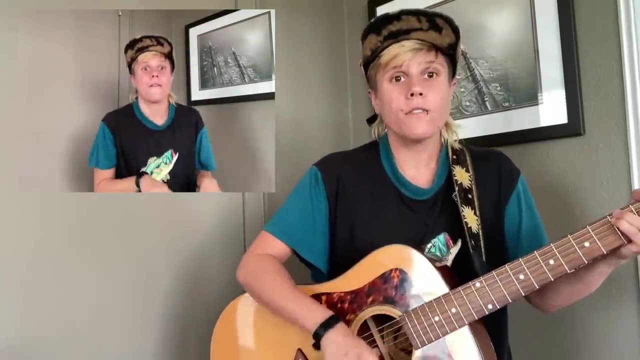 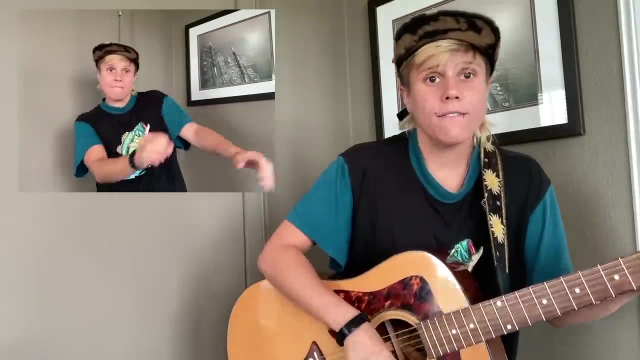 I climbed aboard a pirate ship and the captain said to me: We're going this way, that way forwards, backwards, up and down, up and down over the deep blue sea. We're going this way, that way forwards, backwards, up and down, up and down over the deep blue sea. 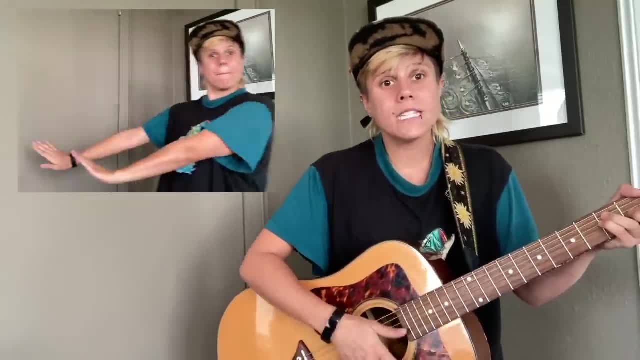 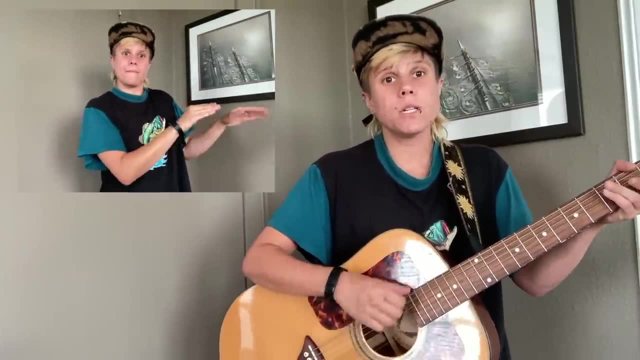 One more time We're going this way, that way forwards, backwards, up and down, up and down over the deep blue sea. One more time We're going this way, that way forwards, backwards, up and down, up and down over the deep blue sea. 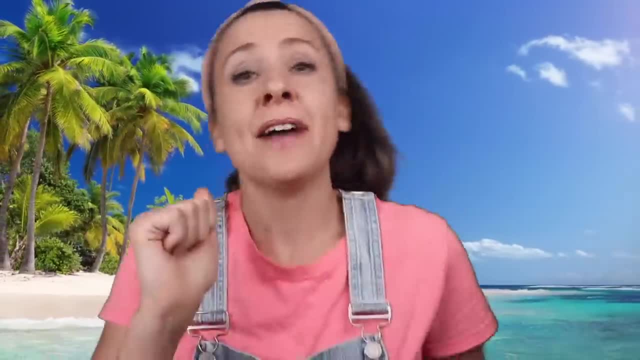 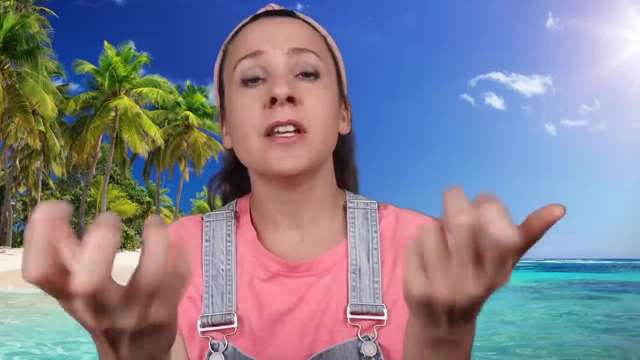 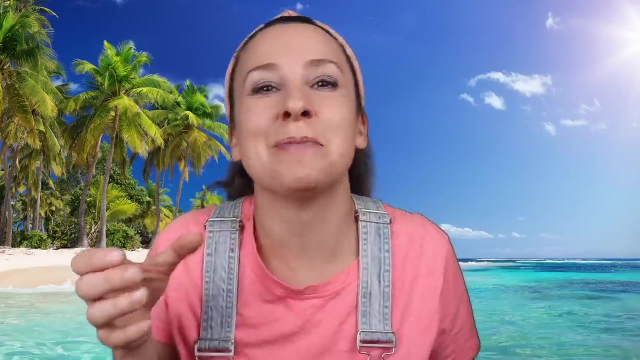 Good job steering the pirate ship. We have to keep walking and finding more treasure. I want a drink. We've been working so hard finding the treasure. It's time for a drink. Let's pretend to drink water. Can you pretend to drink water? 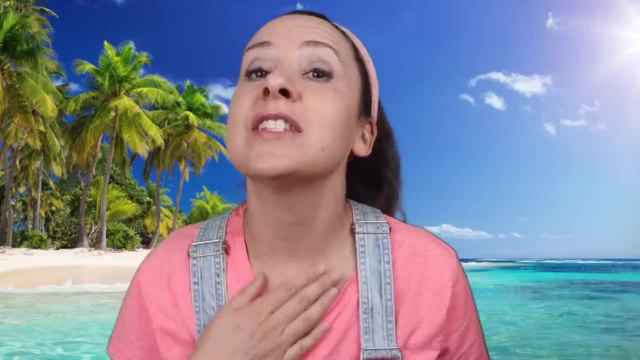 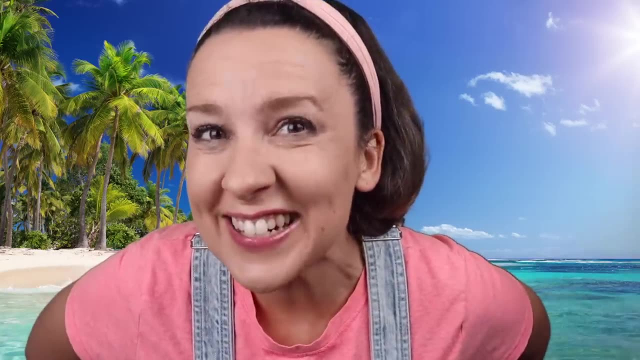 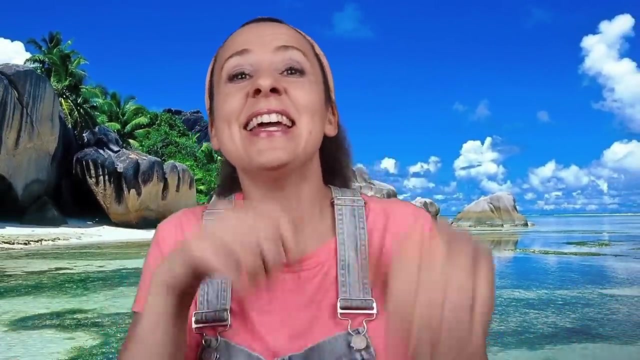 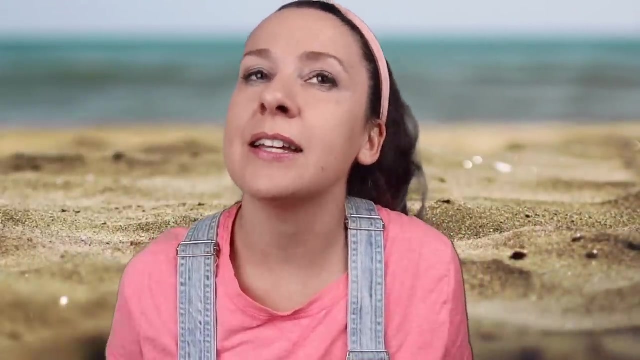 Mmm, so refreshing. I was thirsty, so I had some water. Yay, Let's look for more treasure. Hmm, I can't find any more treasure. Maybe we need to dig, Pretend to dig. Hmm, what could we use to dig? 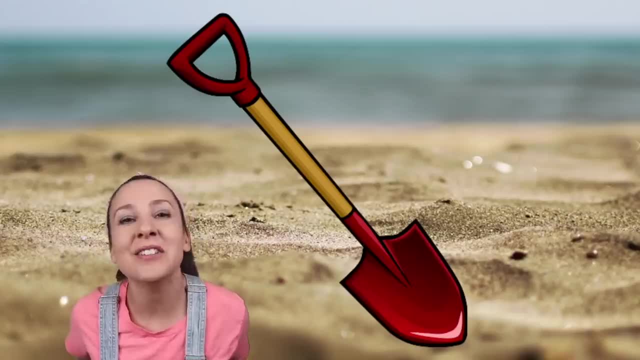 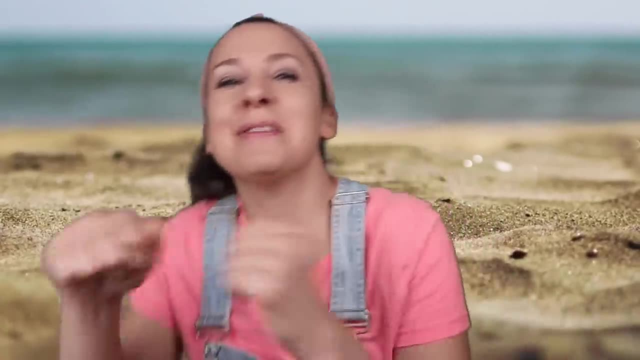 Yes, you got it A shovel. We can use a shovel to dig. Yay, I'm going to pretend I have a shovel. Can you pretend with me? Let's pretend to dig, Digging. We're digging in the sand. 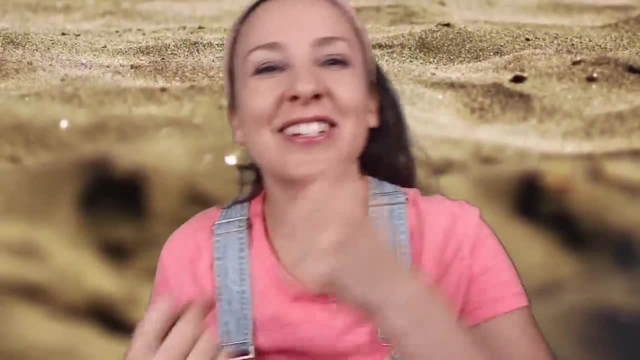 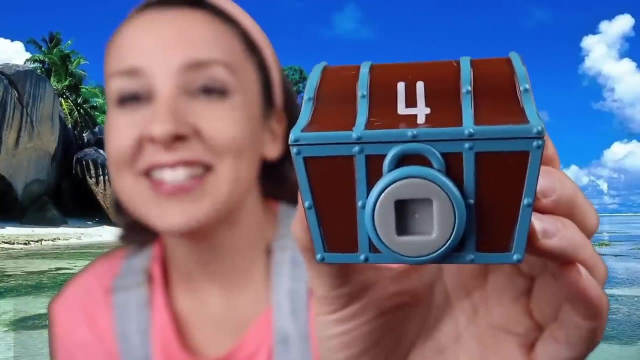 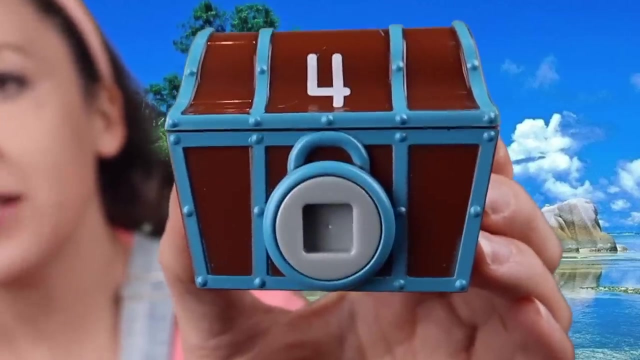 We're digging in the sand. We want to find the treasure, so we're digging in the sand. Yay, Look, We dug in the sand and found a treasure chest. Yay, What color do you see on the brown treasure chest? 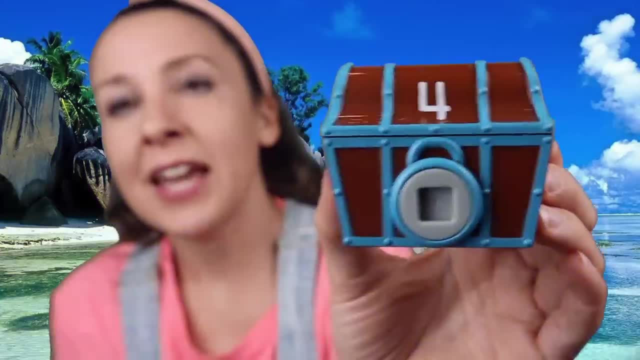 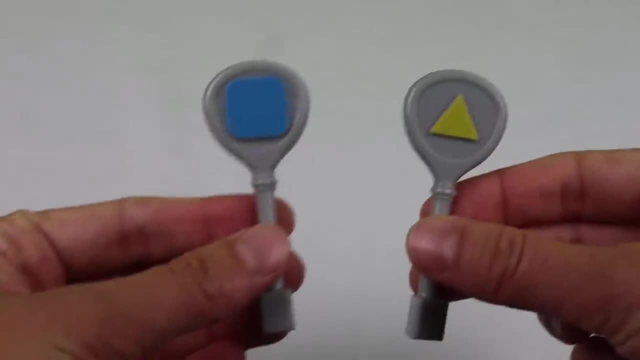 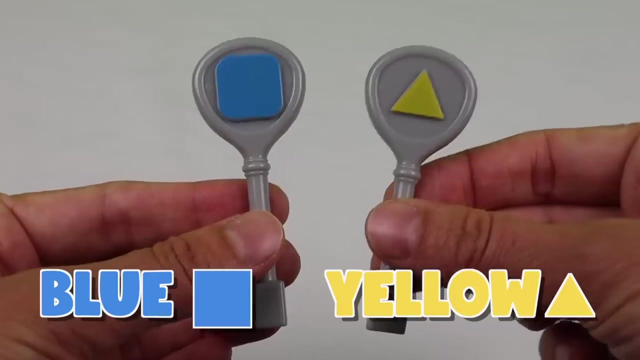 Yeah, it's blue. And what number do you see? Four. Good job To open the treasure chest with the four in it. should we use the key with the blue square or the key with the yellow triangle? Yeah, let's use the key with the blue square. 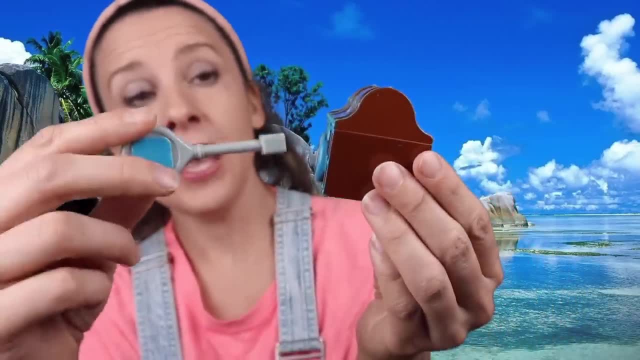 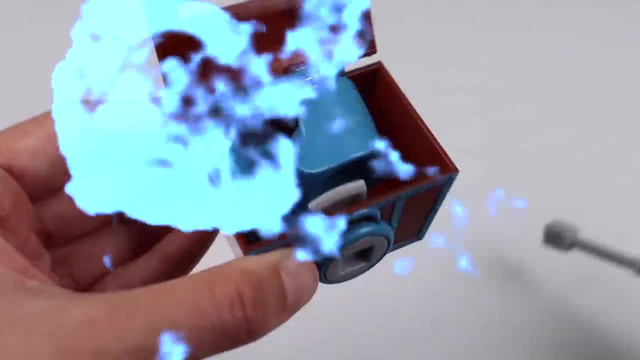 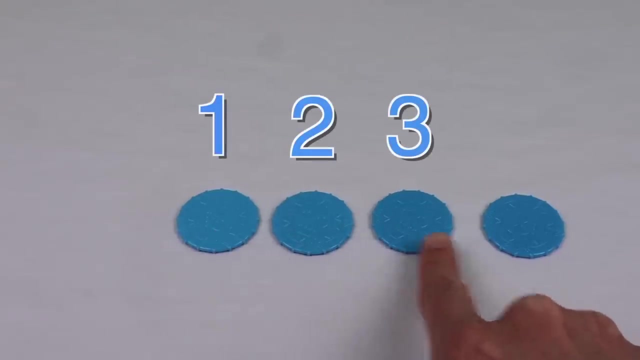 Let's try it. Do you think it's going to work? I do too. Put the key in and turn. Whoa Awesome. Let's see how many coins: One, two, three, four, Four blue coins. Let's see what the surprise is. 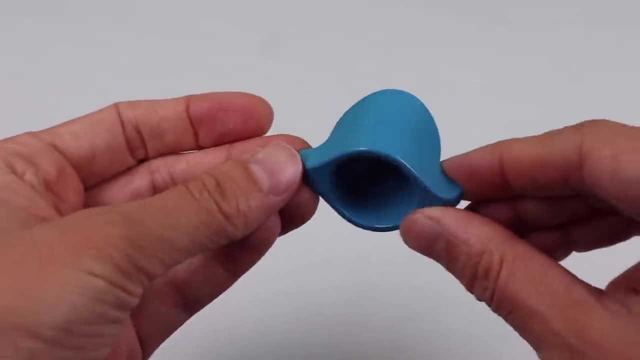 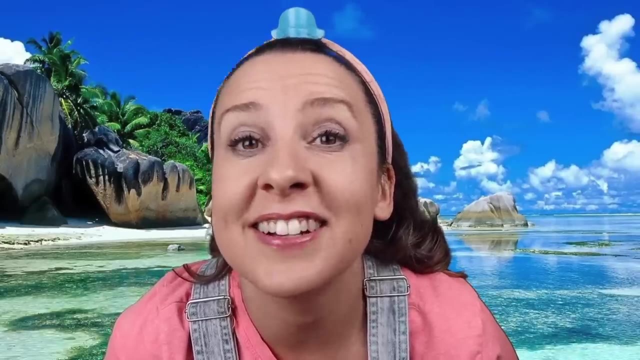 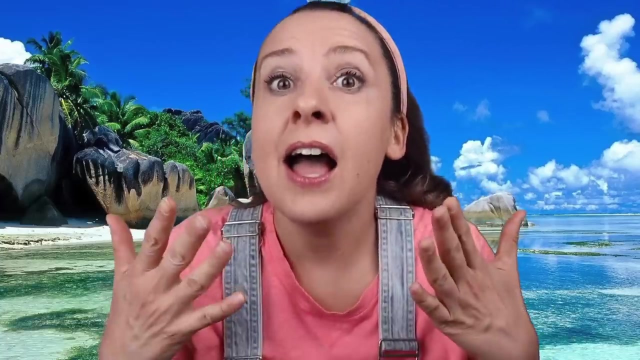 Oh wow, It's a really cool blue hat. Let's see if it fits Miss Rachel. Is it too big or too small for Miss Rachel? Yeah, it's too small. I'm going to sneeze. Ah, ah, achoo. 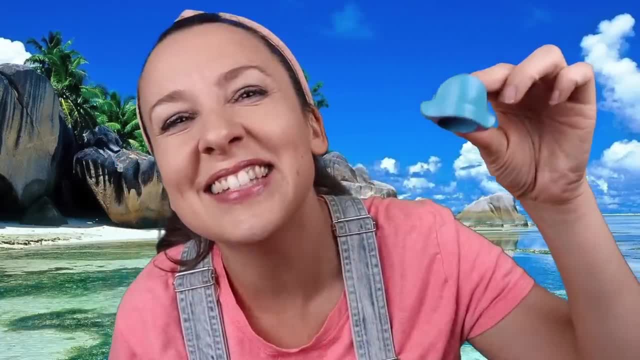 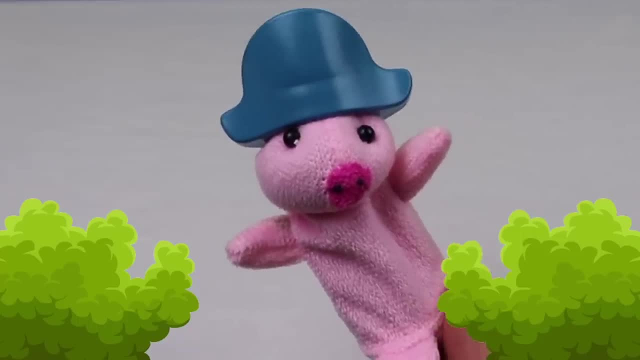 It fell off. That was silly. Hmm, I hope we find someone who can wear the hat. Yay, friends, I found someone who the hat fits. It fits me. Oink, oink. Yeah, it fits this little pig. 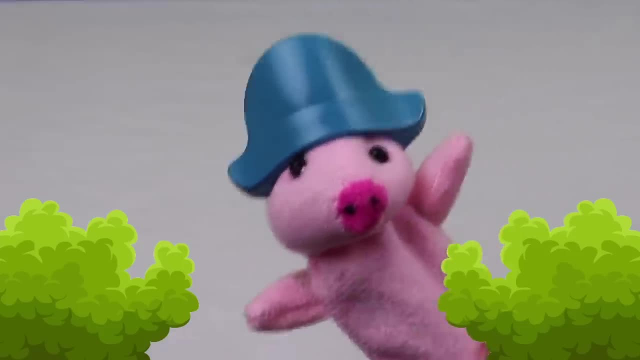 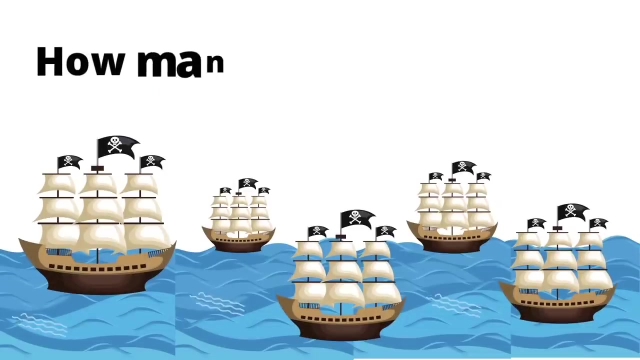 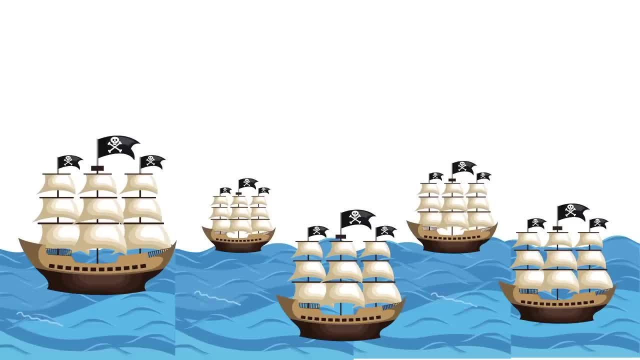 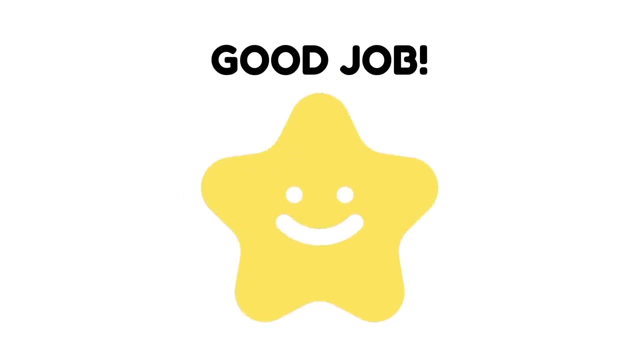 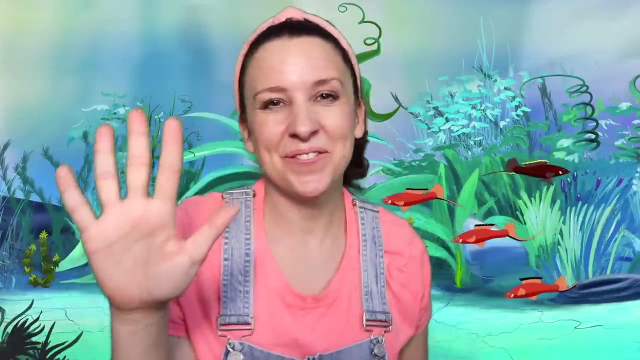 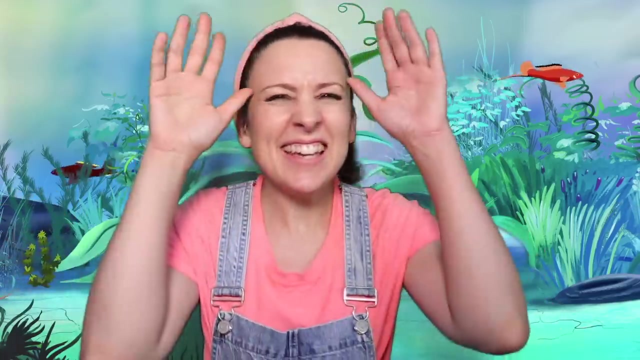 Let's count them: One, two, three, four, five, Five ships- Good job. Can you get out five little fishies? Good job, Five little fishies swimming in the sea Teasing- Mr Sharky can't catch me. 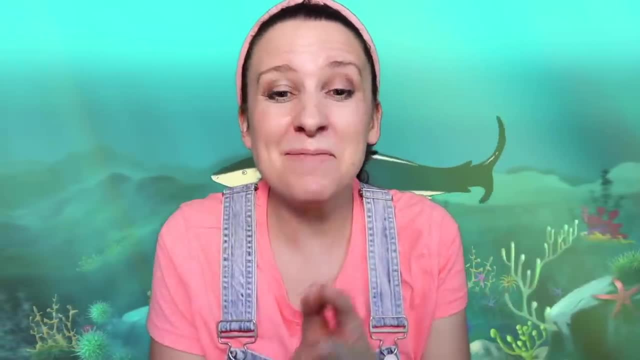 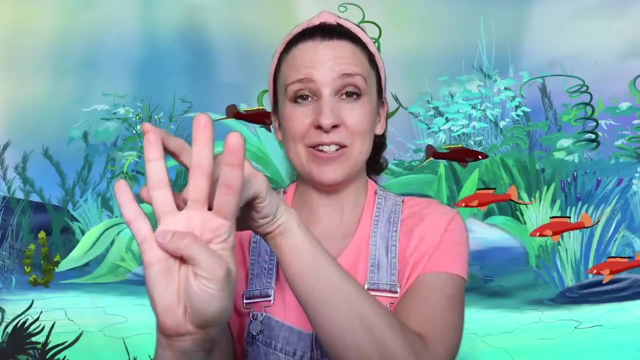 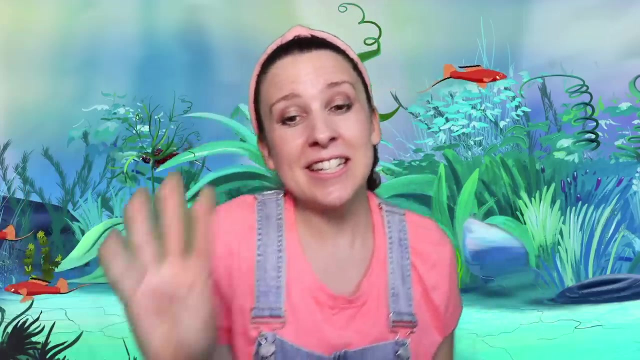 Along comes Mr Sharky, quiet as can be, And snapped that fishy right out of the sea. How many are left? One, two, three, four, Good counting Four little fishies swimming in the sea Teasing. Mr Sharky can't catch me. 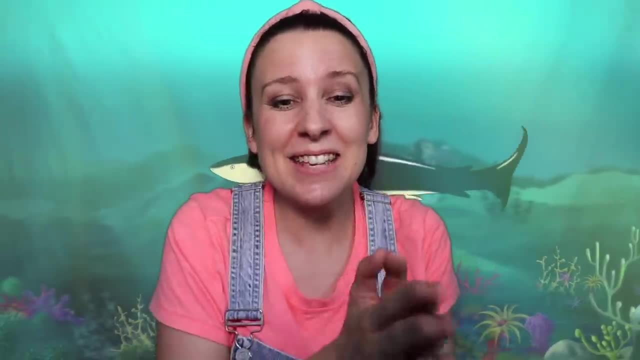 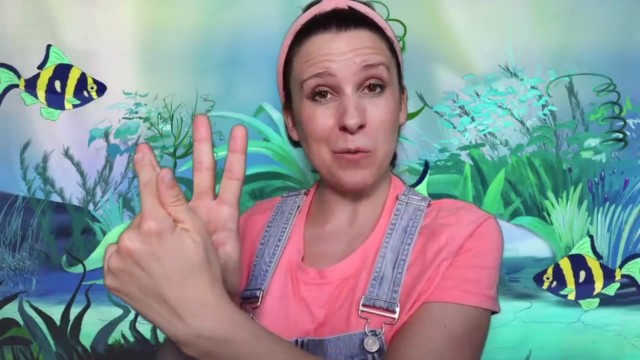 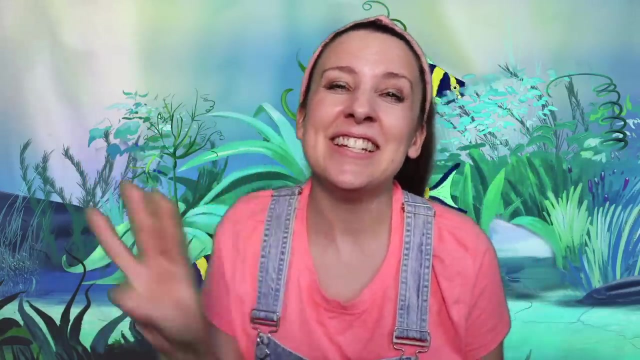 Along comes Mr Sharky, quiet as can be, And snapped that fishy right out of the sea. How many are left? Count with me One, two, three, Three. Good job, Three little fishies swimming in the sea. 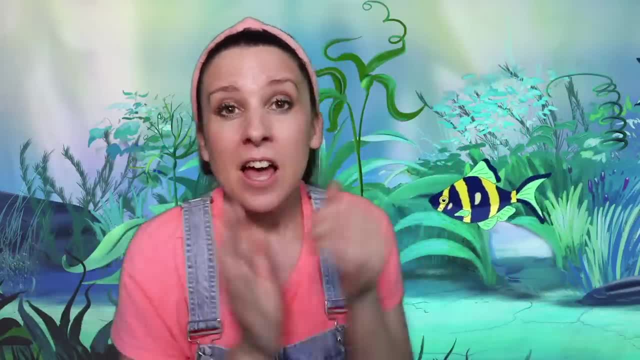 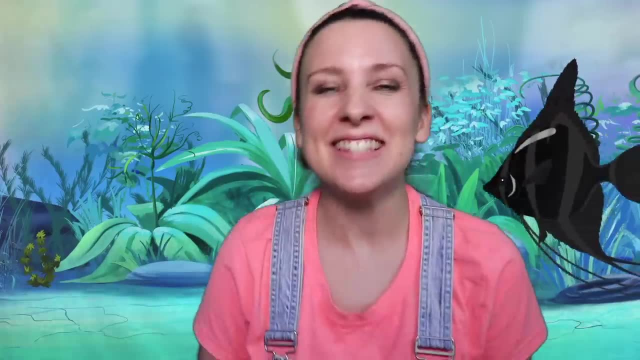 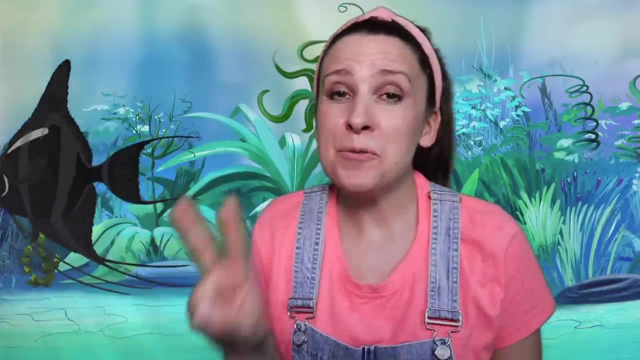 Teasing, Mr Sharky can't catch me. Along comes Mr Sharky, quiet as can be, And snaps the fishy right out of the sea. Good singing. How many are left? One, two, Two little fishies swimming in the sea. 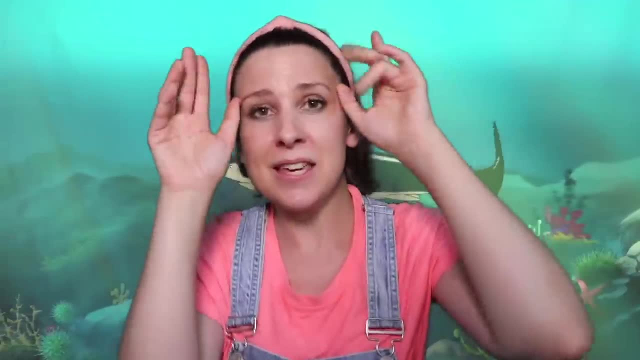 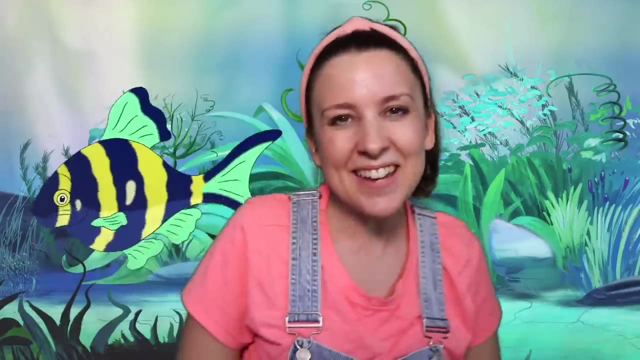 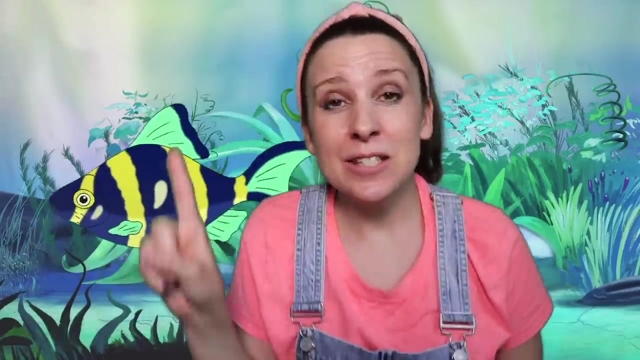 Teasing, Mr Sharky can't catch me. Along comes Mr Sharky, quiet as can be, And snaps the fishy right out of the sea. How many are left? Just one One little fishies swimming in the sea. 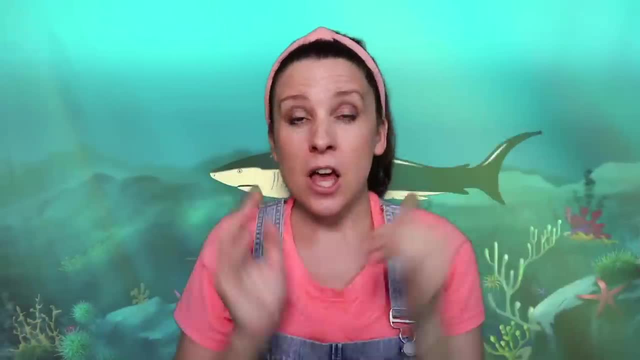 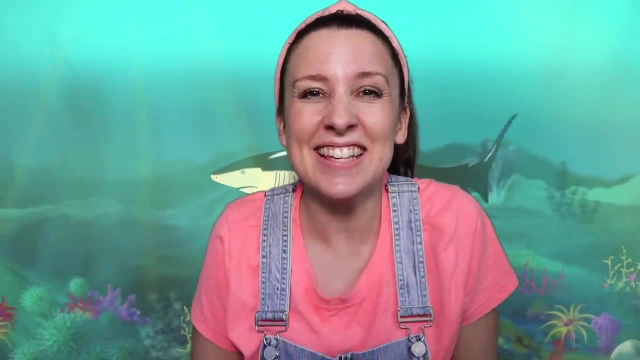 Teasing, Mr Sharky can't catch me. Along comes Mr Sharky, quiet as can be, And snaps the fishy right out of the sea. And snaps the fishy right out of the sea. That was so good. 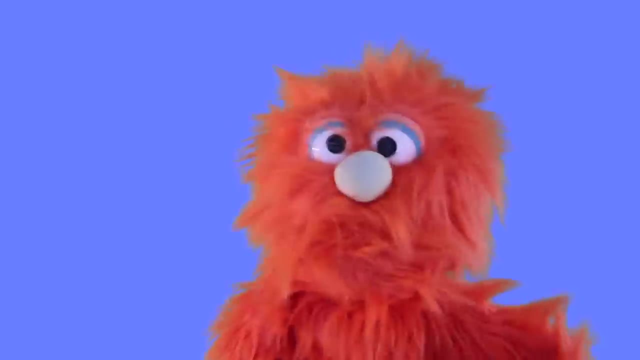 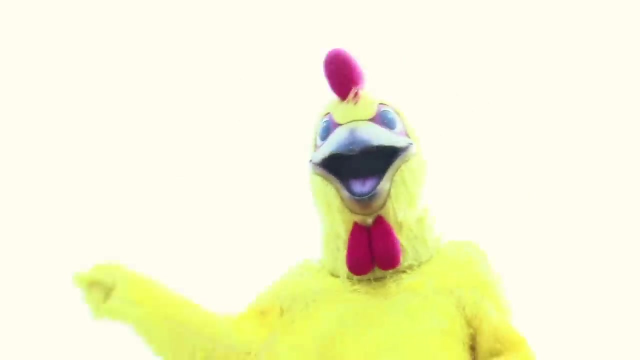 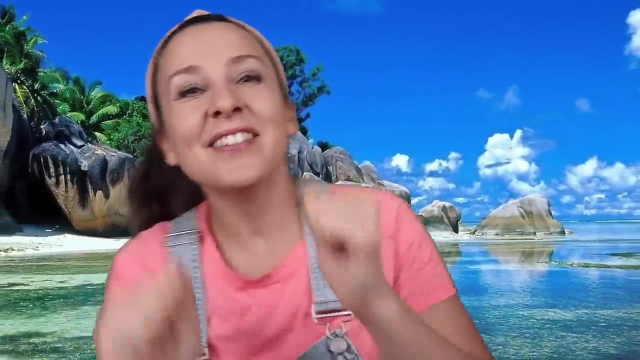 Great job, friends. Okay, we're going to get it this time. One, two, three chicken. Can you march around while we look for treasure? We're marching all around. We're marching all around. We're looking for a treasure, so we're marching all around. 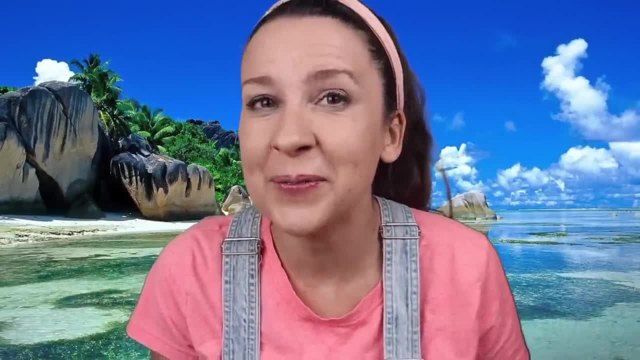 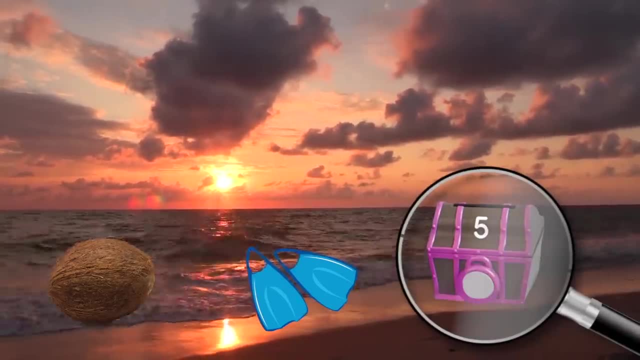 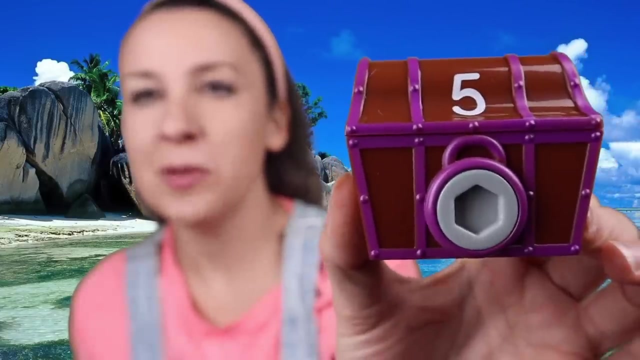 Yay, Yay, I'm so proud of you. Do you see any more treasure? Oh, wow, I think you found it. What color do you see on the brown treasure chest? Yeah, that color is purple. And what number? 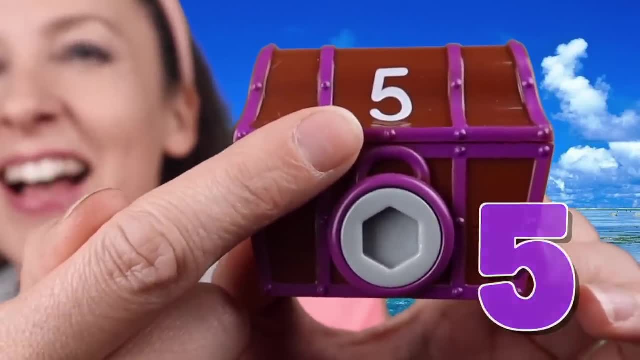 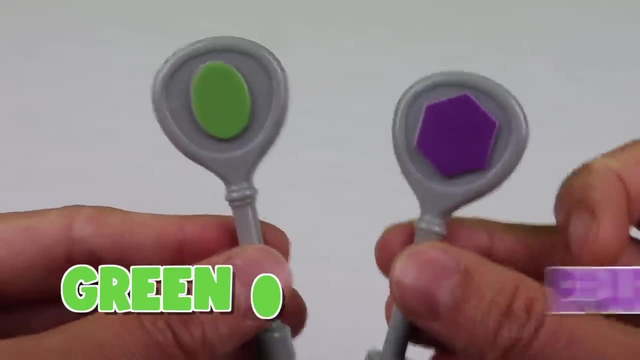 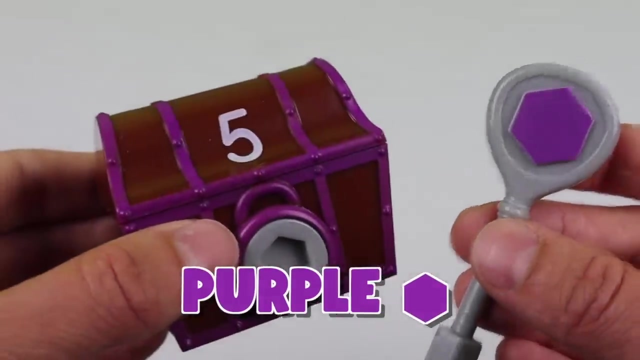 Yeah, that's five. Good job To open the treasure chest with purple on it. should we use the key with the green oval or the key with the purple hexagon? Yeah, the key with the purple hexagon, Because the treasure chest has purple on it and a hexagon. 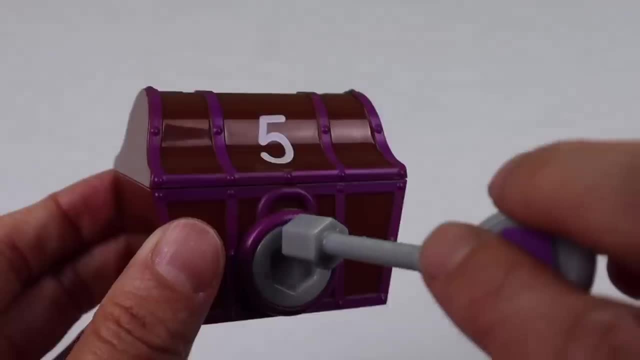 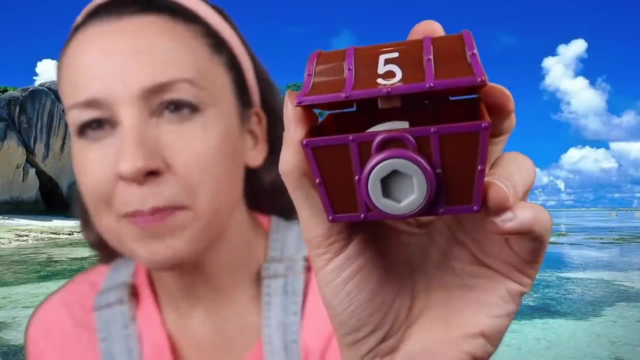 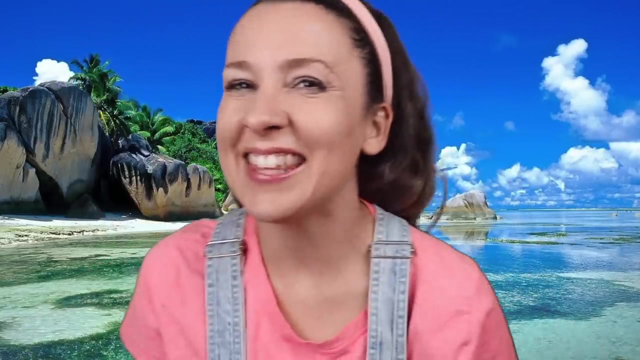 Okay, get out your key, Say open please, And we'll turn the key. Yay, Let's count the coins. How many purple coins do you think we're going to find if there's a five on the treasure chest? I think five too. 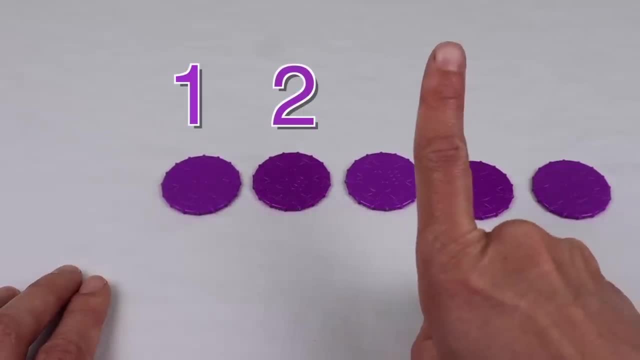 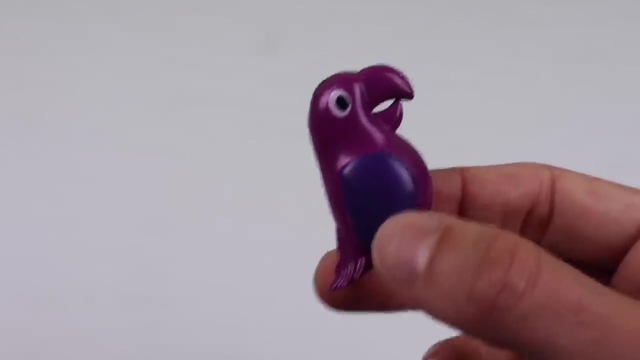 One, two, don't say three, yet three, four, five. We did it, We counted to five. That's so awesome. Let's see what the surprise is. Wow, It's a cute purple parrot. Hello, Thank you for finding me. 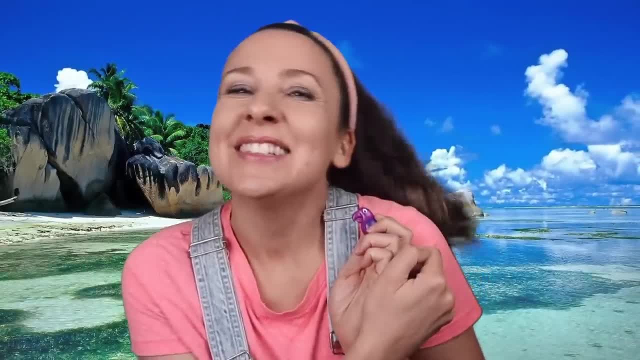 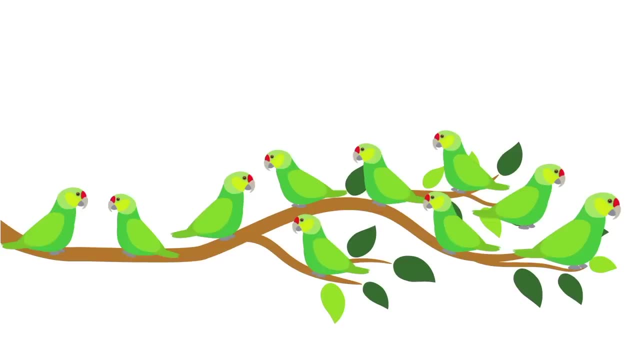 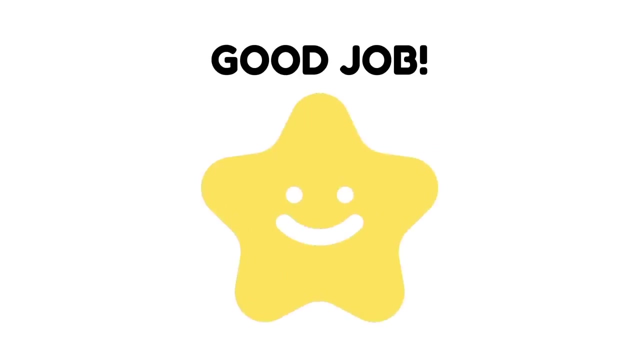 Oh, the parrot's giving you a kiss, So sweet. How many parrots are there? Let's count them: One, two, three, four, five, six, seven, eight, nine, ten, Ten parrots, Good job. 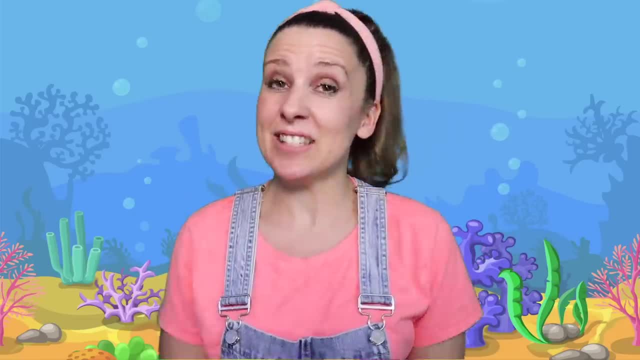 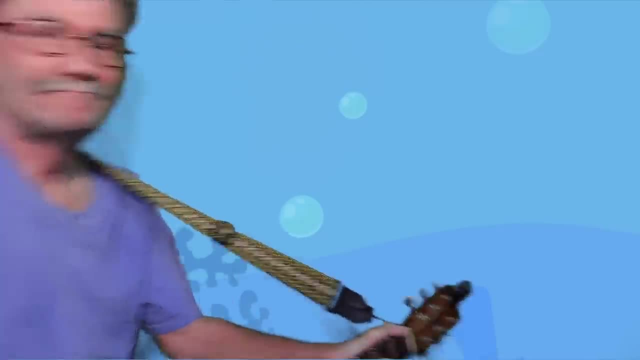 Let's pretend to be ocean animals together. It's going to be so much fun. Papa Tim's here again to help us with the guitar. Hi kids. First let's pretend to be fish. The fish in the sea go, swim, swim, swim. 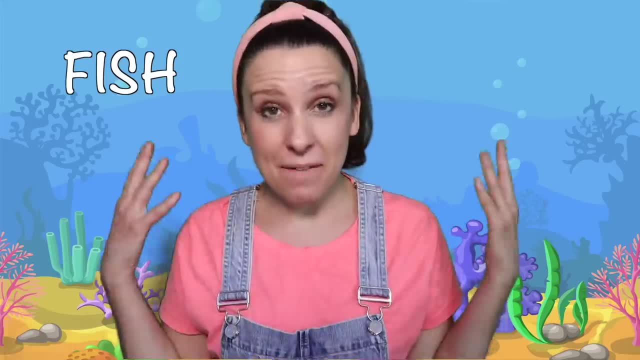 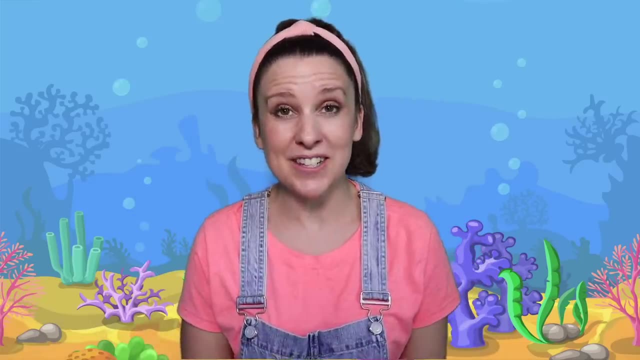 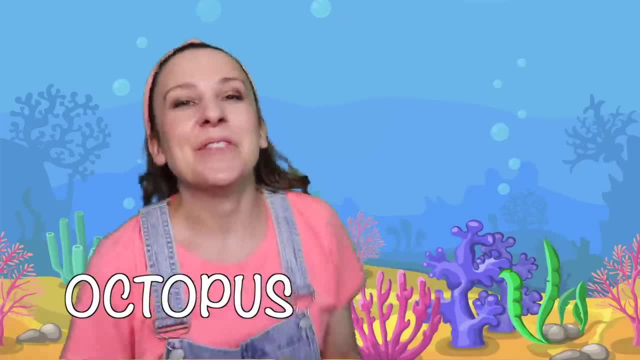 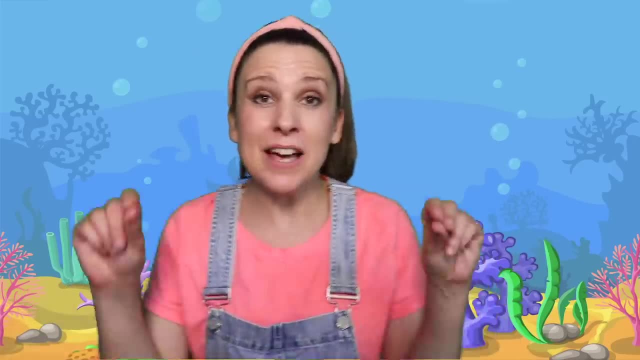 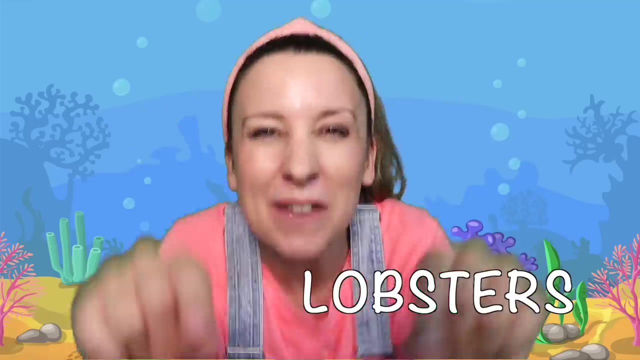 Wiggle, wiggle, freeze, Wiggle, wiggle, freeze. The octopus in the sea go wiggle, wiggle, freeze All day long. Now let's be a lobster. Can you pinch like a lobster? The lobsters in the sea go pinch, pinch, pinch. 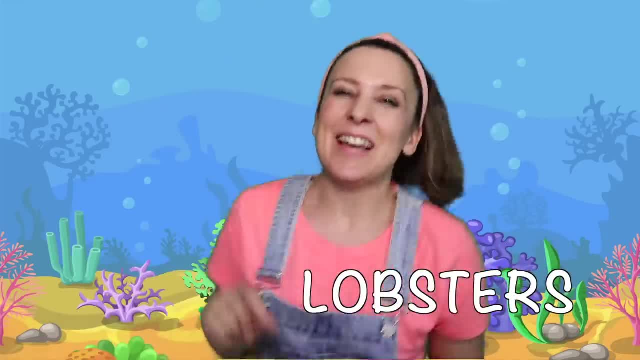 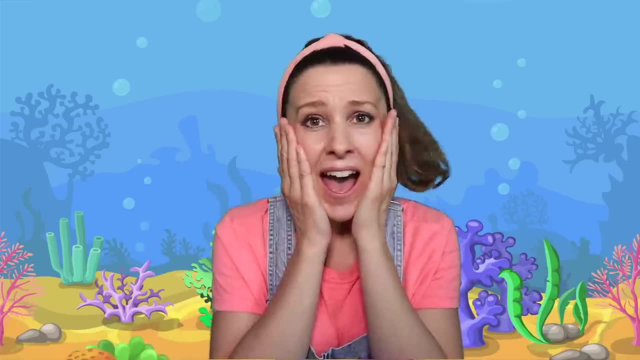 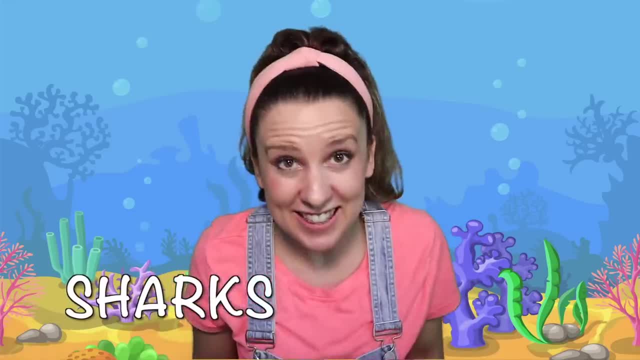 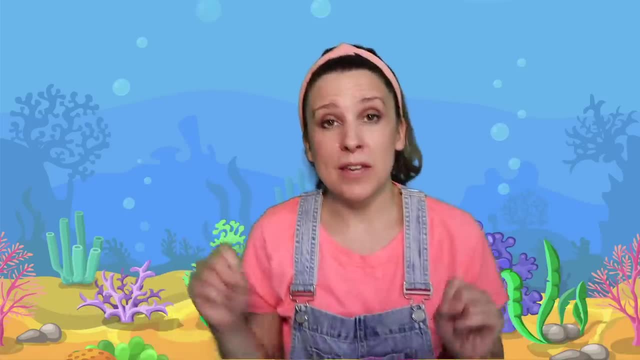 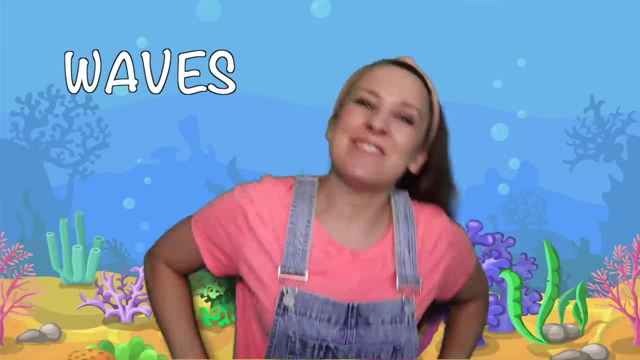 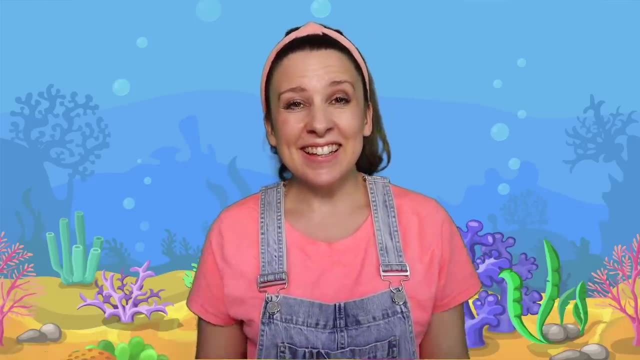 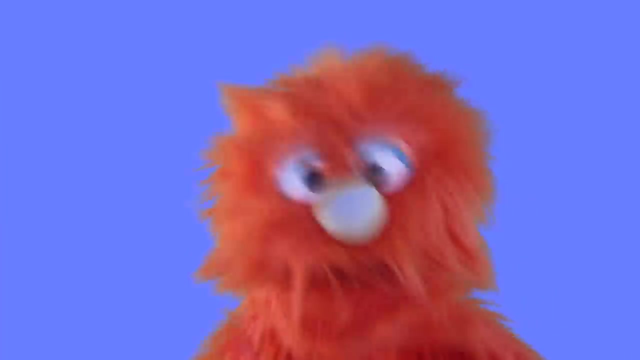 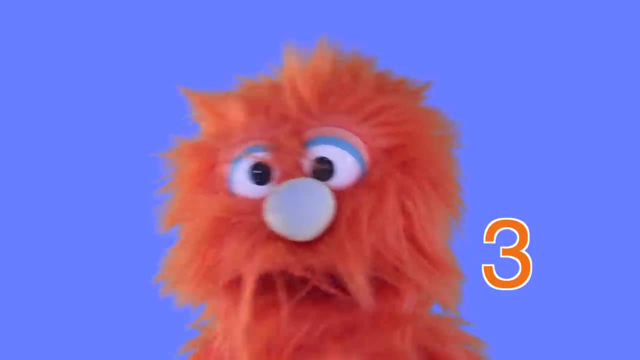 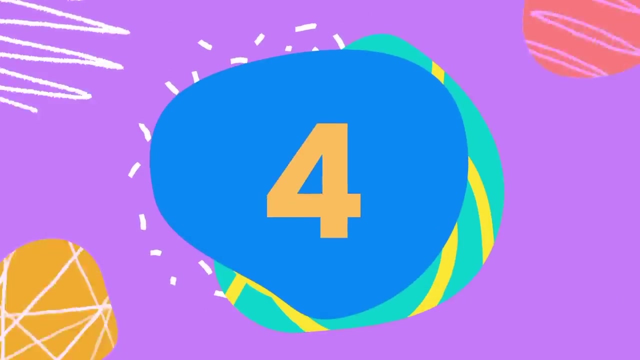 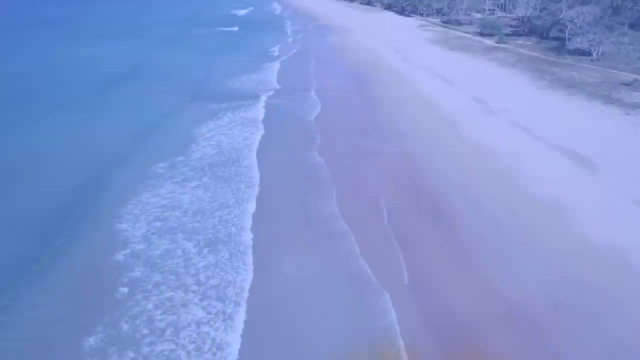 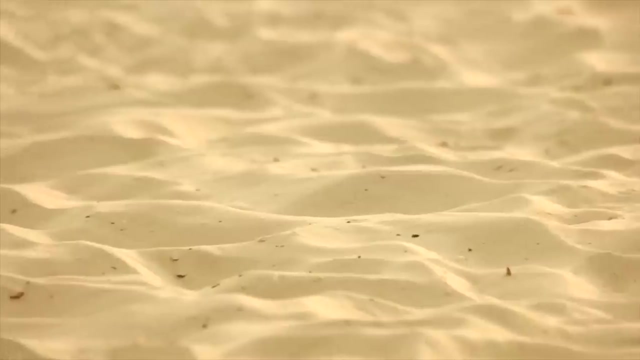 You help me. One, two, three, door Four, Miss Rachel. One, two, three, four. We did it Good job. It's time for our lesson. A beach is land next to a lot of water. It can be sandy or rocky. 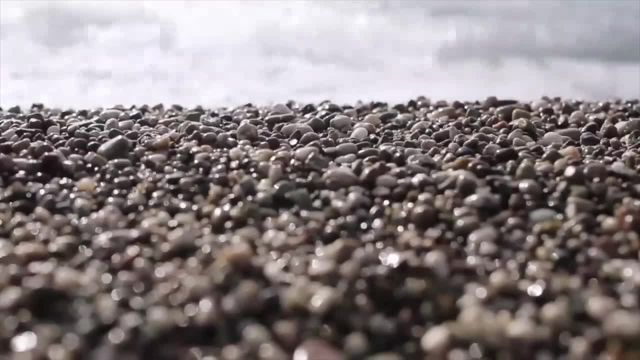 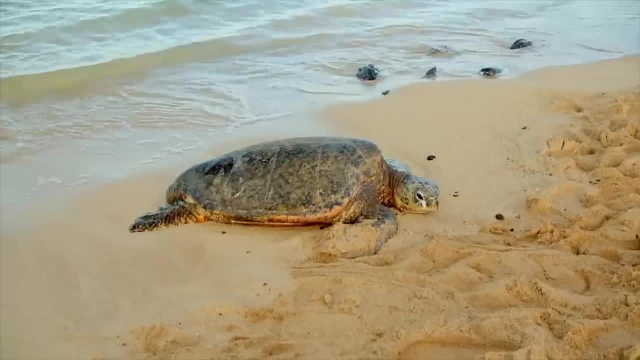 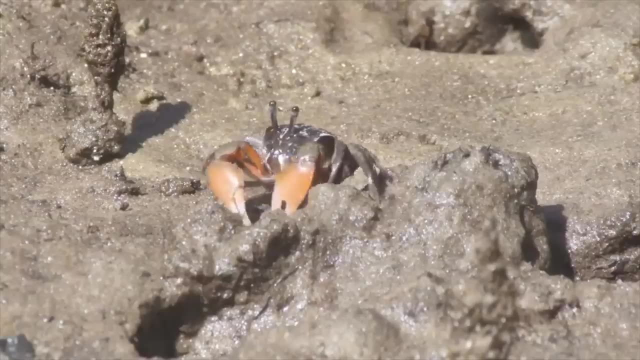 It can have lots of pebbles. Pebbles are tiny little rocks. The ocean is a big body of salt water. Some animals that like to spend time on the beach are sea turtles, birds like seagulls, crabs, seals. 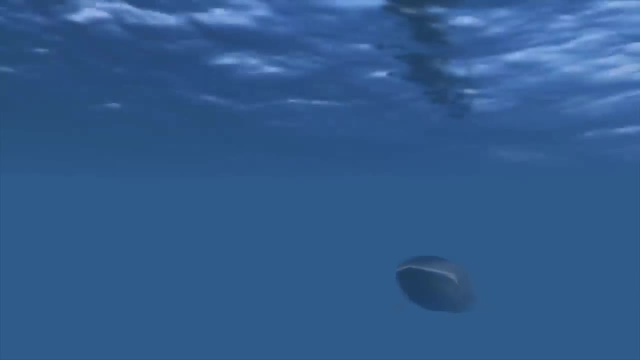 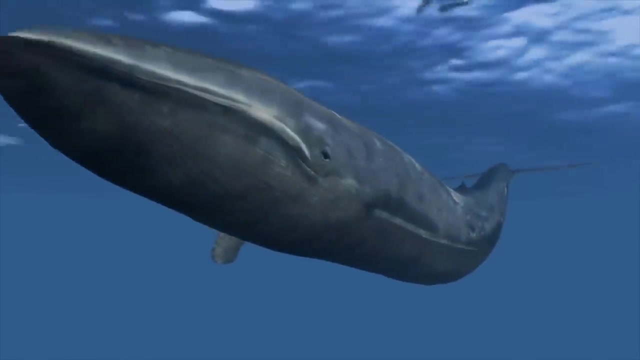 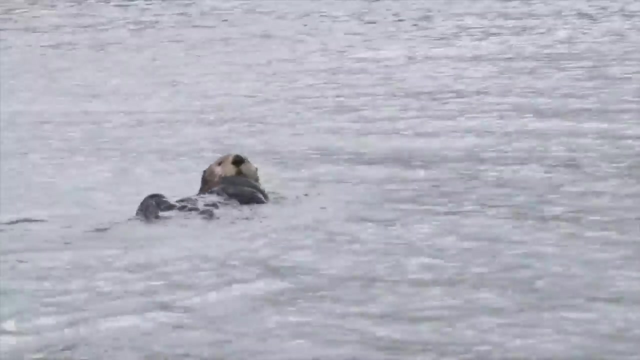 and sea lions. The biggest animal in the world lives in the ocean. It's the blue whale. Blue whales can be as long as two buses. Some other animals that live in the ocean are fish, sharks, sea otters and seals. 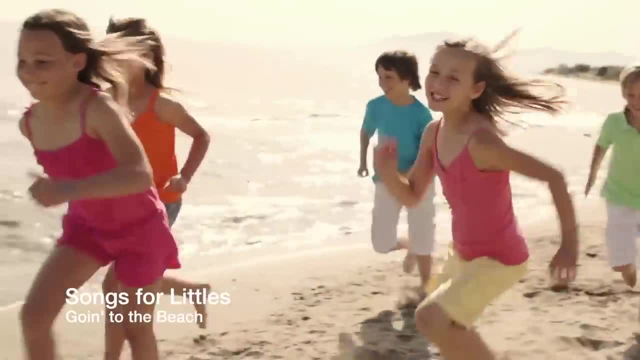 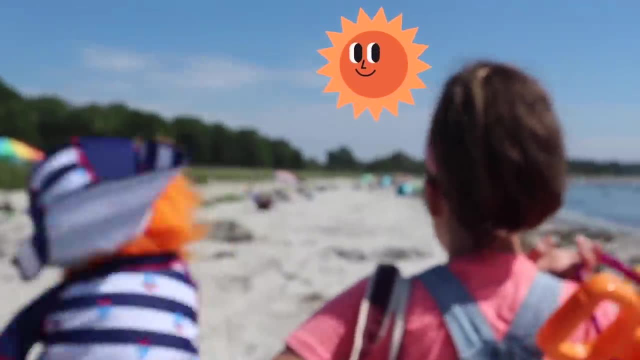 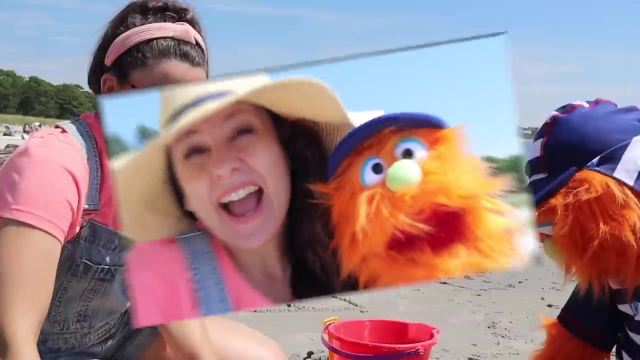 I'm going to the beach. Going to the beach. Going to the beach on a sunny day. We've got books we can read. We've got all that we need here to play. Going to the beach. Going to the beach to have some fun. 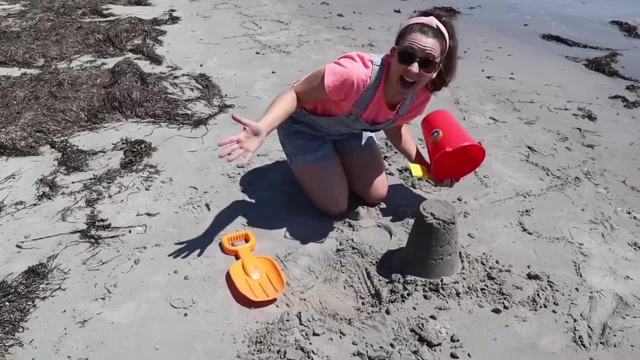 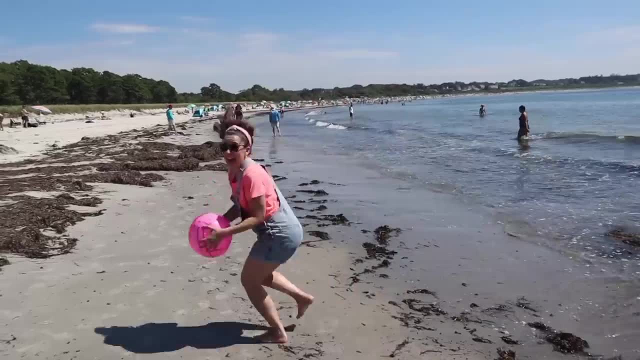 With a bucket in hand. we'll dig holes in the sand. We'll build castles and boats- and we might see some boats. Then we'll splash in the sea. You and me will have fun in the sun. We're going to the beach. 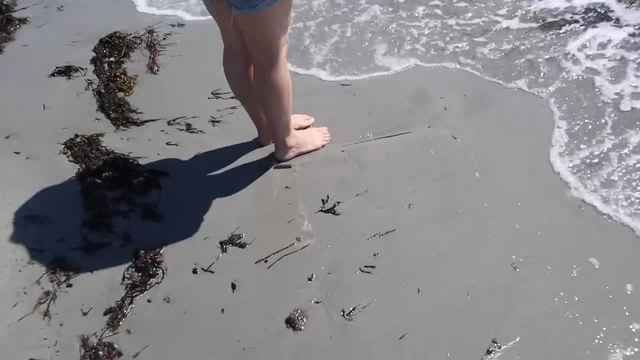 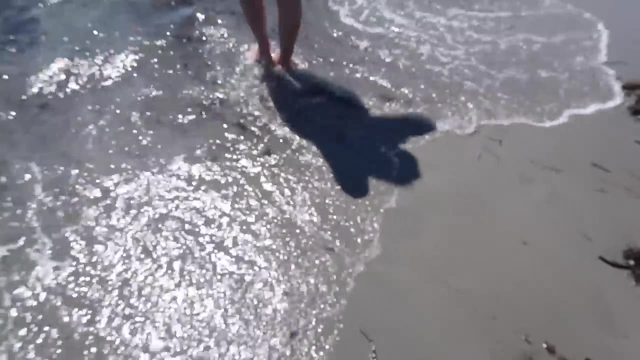 With our water and fruits And our sunscreen and suits. We'll feel the sand on our feet As we play in the heat. We'll write our names in the sand. On this beautiful Etch-a-Sketch land, We're going to the beach. 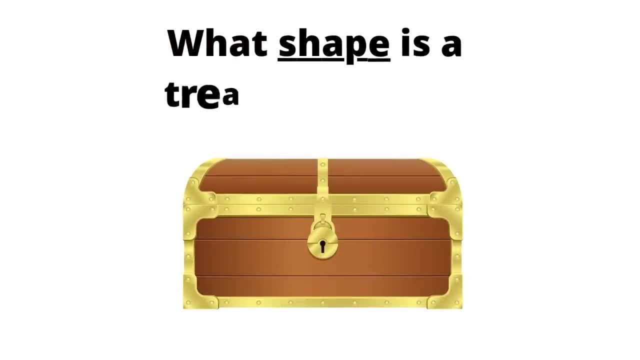 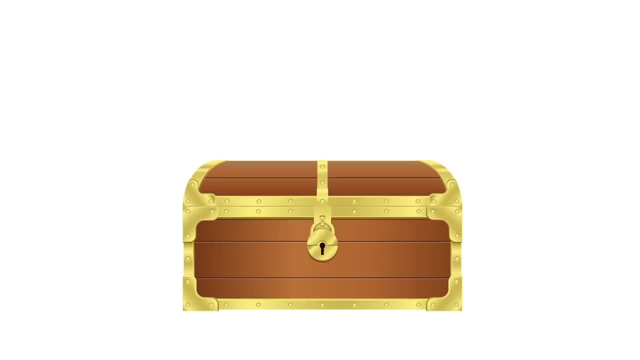 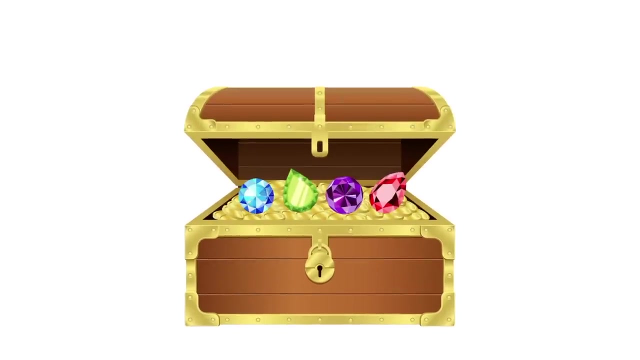 Peek-a-boo. What shape is a treasure chest? I'll give you a clue. Yeah, It's a rectangle. Can you help me open the treasure chest? Say open, Open. Wow, look at those beautiful jewels. Can we name the colors? 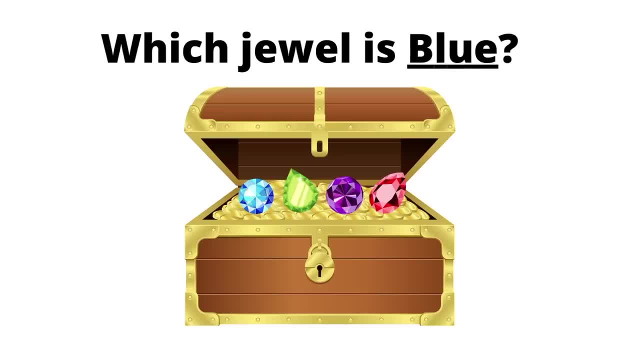 Which jewel is blue? Yeah, this jewel is blue. Which jewel is red? This one's red. Which jewel is green? Yeah, that's a green jewel. Which jewel is purple? Yeah, it's a purple jewel. Thank you for helping me name all the colors of the jewels. 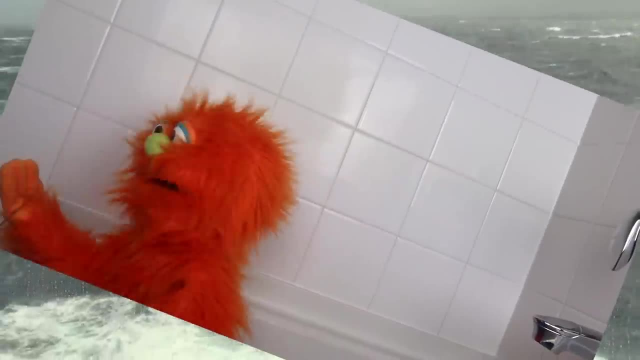 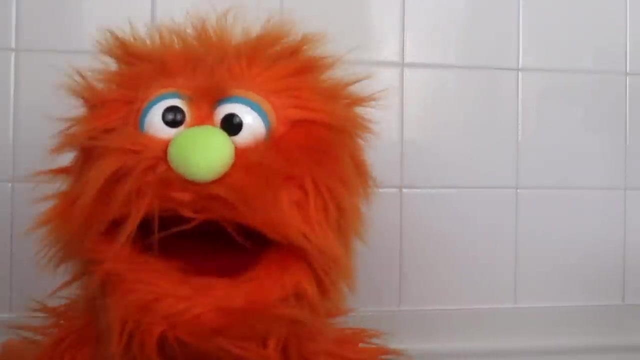 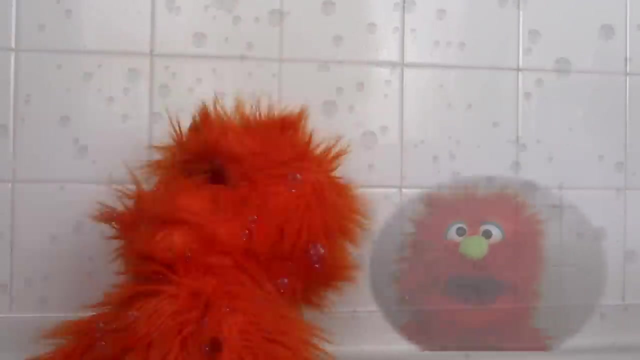 Good job. Turn the ship, Bend the hatches, Whatever that means, This is fun. Row, row, row your boat Gently down the stream, Merrily, merrily, merrily, merrily. life is but a stream. 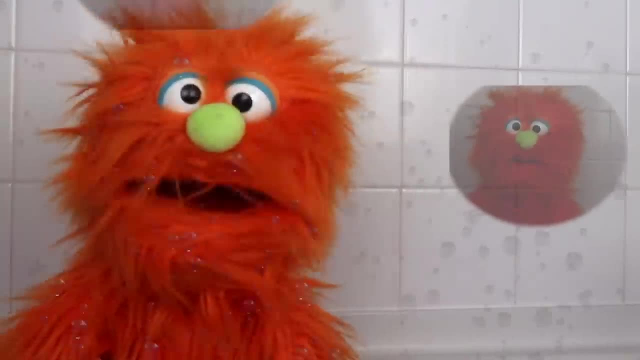 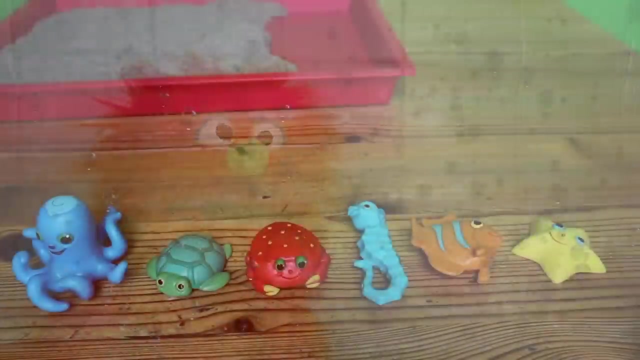 Merrily, merrily, merrily, merrily. life is but a stream. Merrily, merrily, merrily, merrily. life is but a dream. Next, I'd like to show you our little ocean animals. 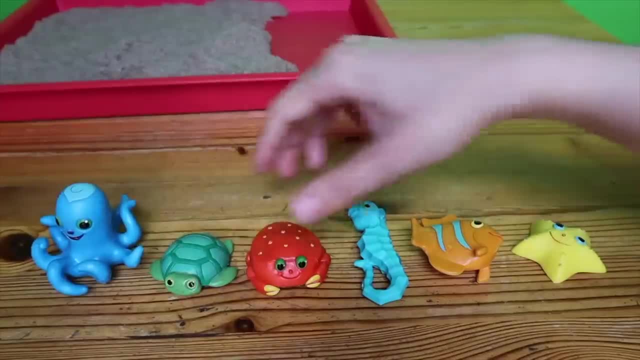 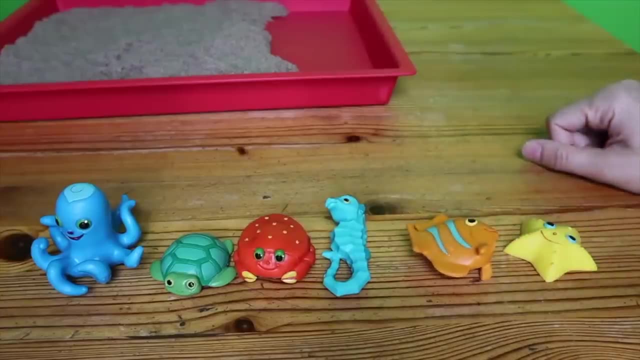 So we have an octopus, a little sea turtle, a crab, a seahorse, a fish and a star. Now look at them very closely. Now look at them very closely because I'm going to play a game with them. 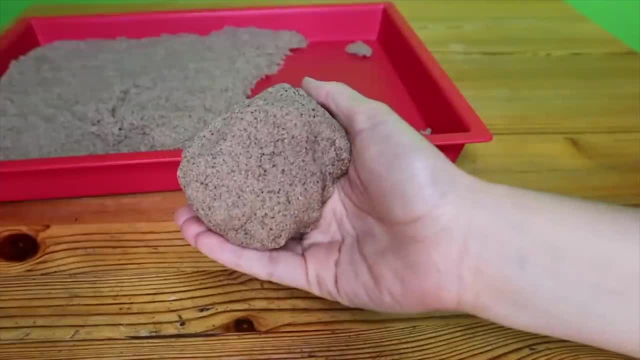 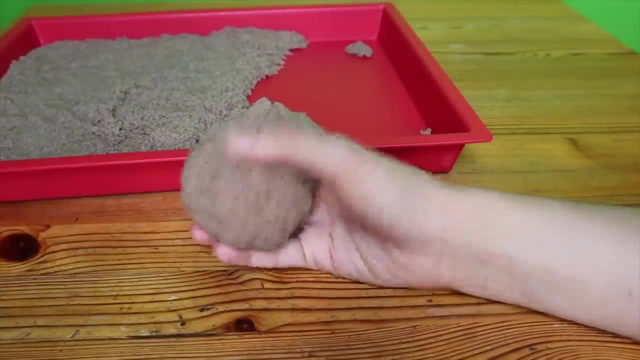 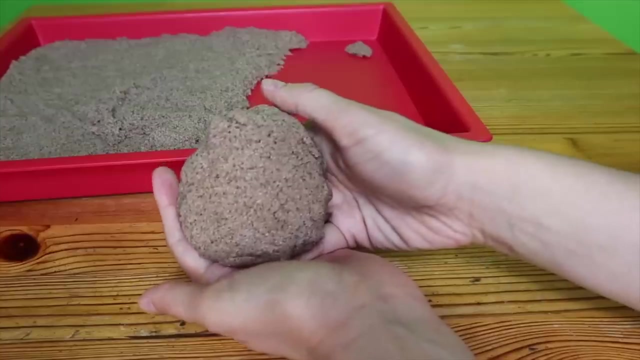 And I'm going to try and trick you. Which animal do you think is hiding in the sand? Peek-a-boo, I showed you a clue. Peek-a-boo, Oh, it was the color red. Hmm, do you know which one it is? 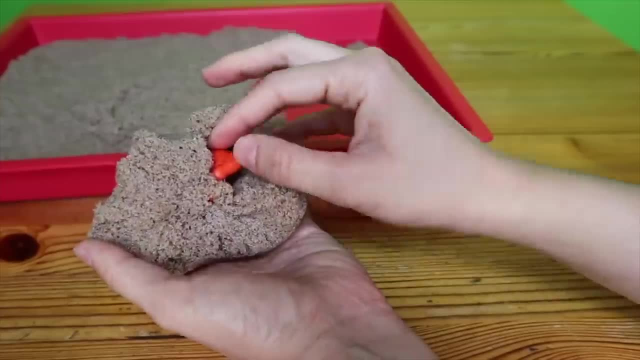 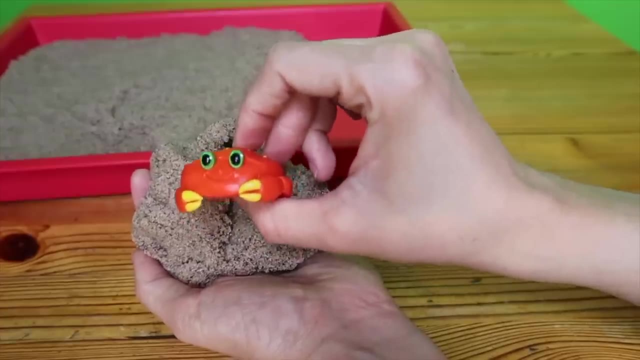 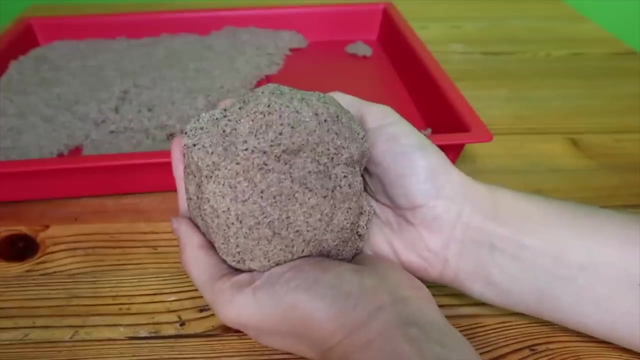 Yeah, it's the. Let's take it out The crab. Good job. I was hiding in the sand. Did I trick you? You didn't trick us. We knew it was you. Who do you think is hiding in this sand ball? 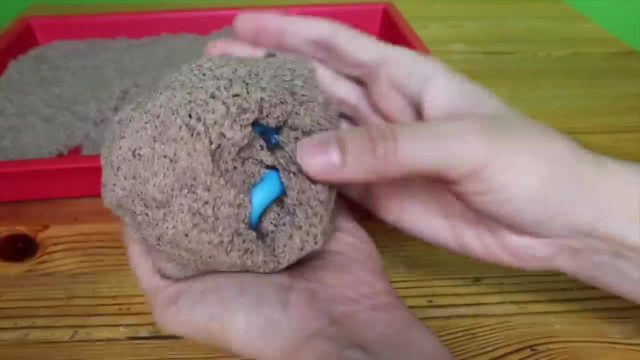 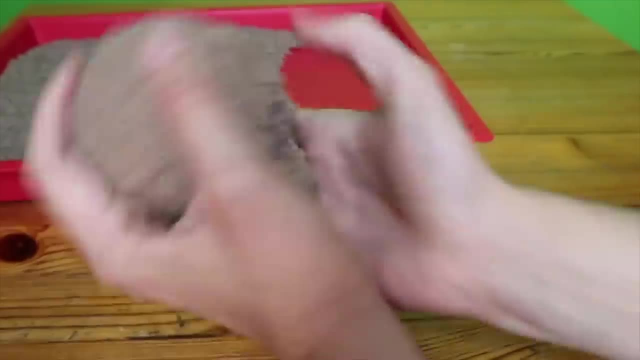 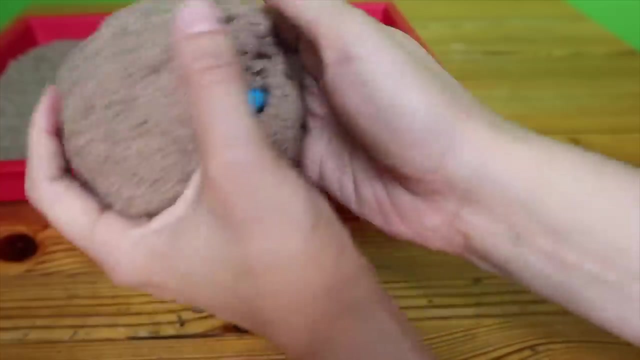 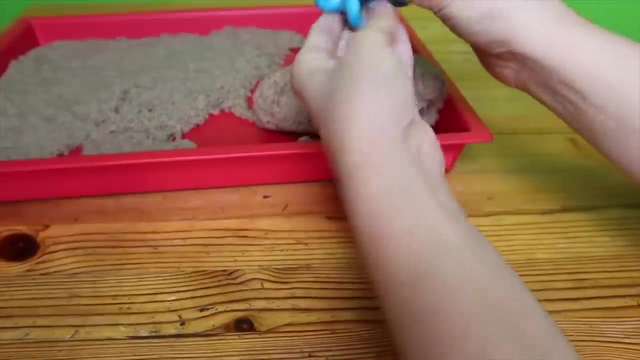 I'll give you a clue. Peek-a-boo, What did that look like? Peek-a-boo, What do you think? it is An A Octopus. What a silly octopus. There he is, You found me. 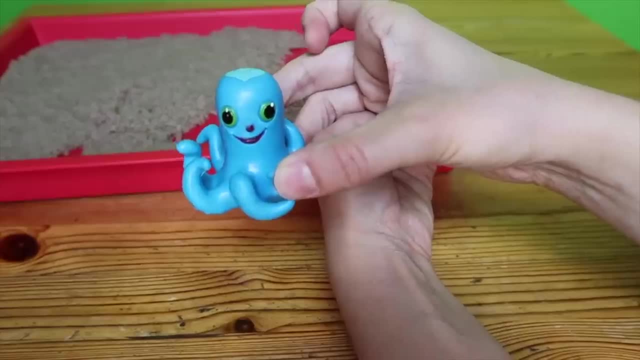 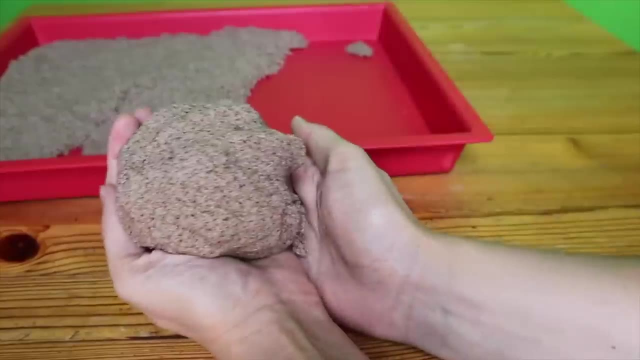 I was hiding in the sand. Did I trick you? No, you didn't trick us. We knew it was you. Good job playing the game. Who do you think is hiding in this sand ball? Peek-a-boo? Who was that? 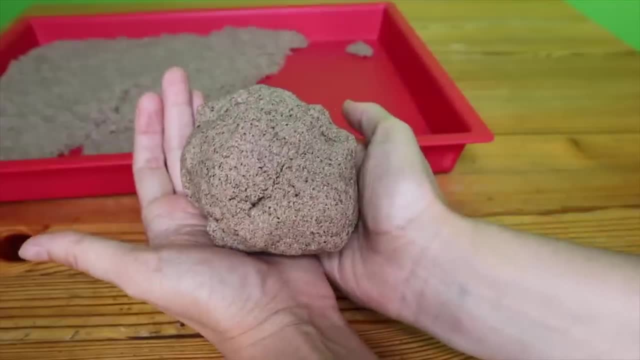 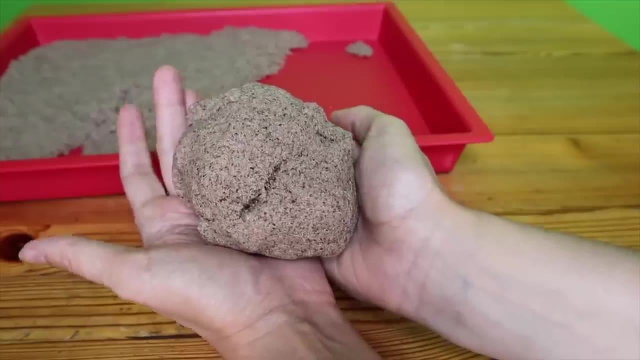 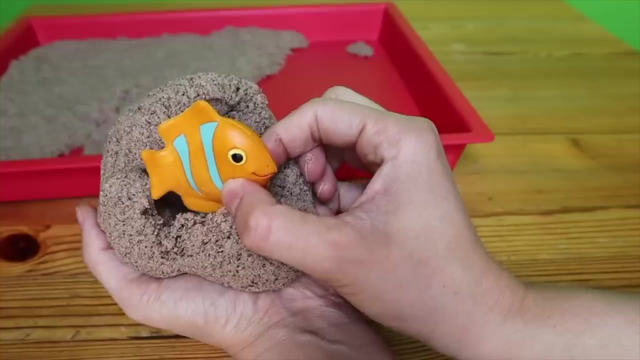 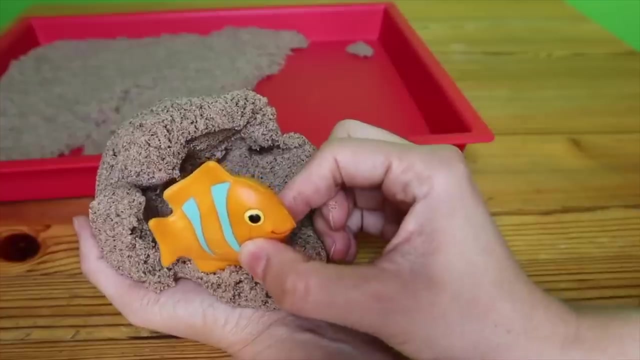 Peek-a-boo. It starts with the letter F. What do you think? It's a Fish? It was a fishy. Did I trick you? Swim, swim, swim. You didn't trick us, Mrs Fish. We knew it was you. 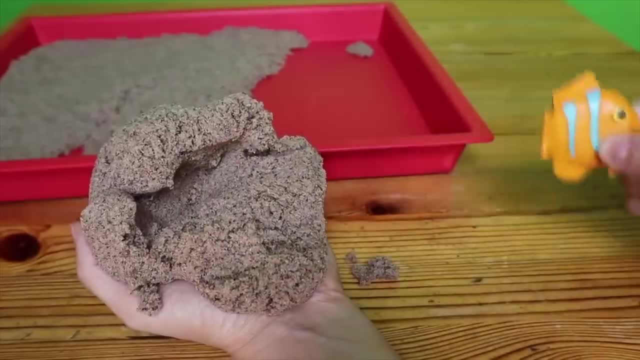 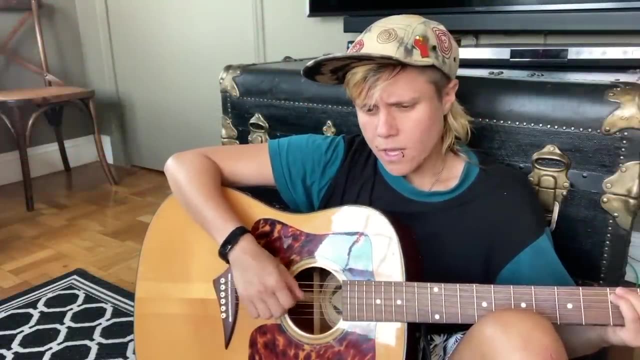 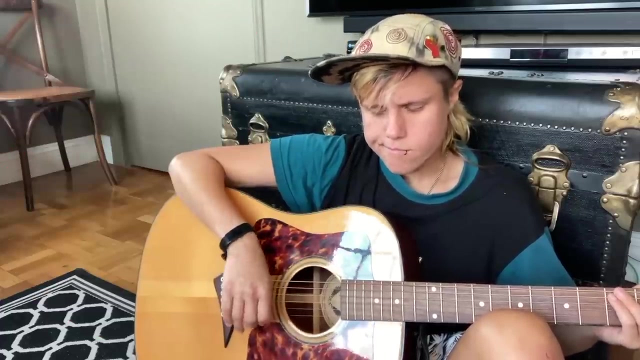 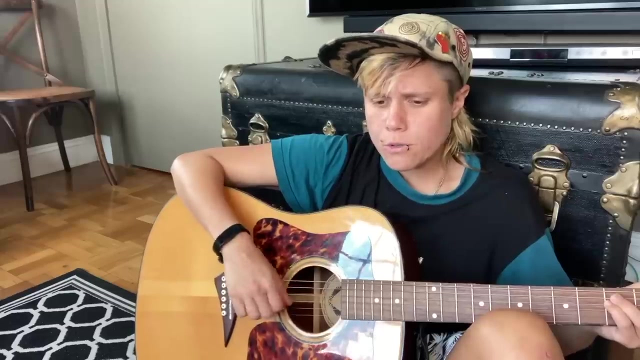 Thanks for playing. Swim, swim, swim, Bye-bye. I'm in a very bad mood. I'm feeling like a crab, A crabby crab. I'm in a terrible mood. I don't know what to do. I'm such a crab. 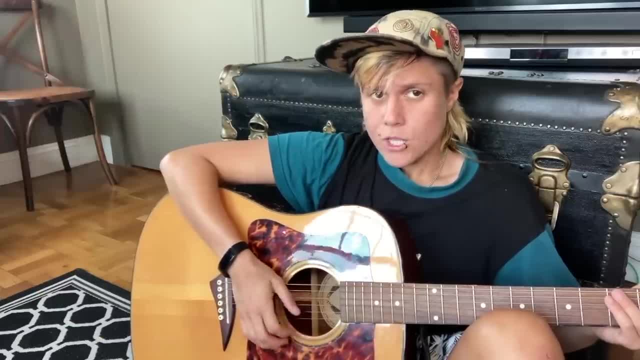 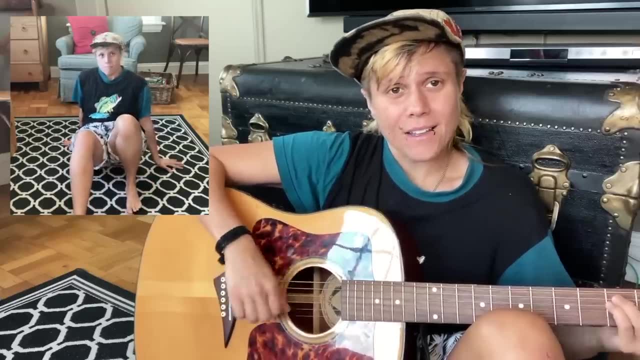 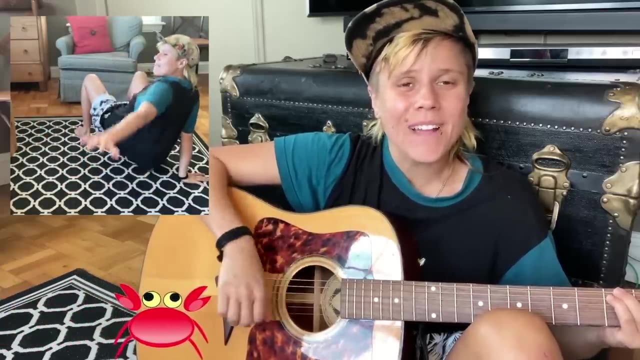 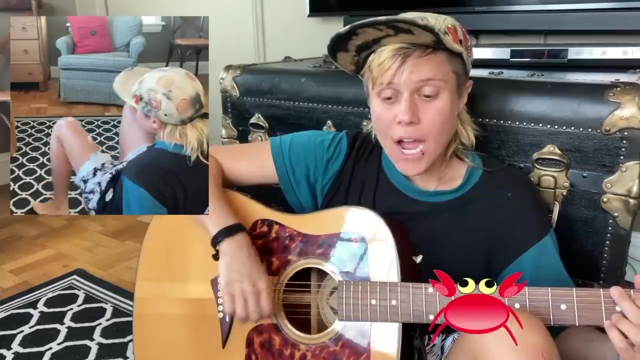 A crabby crab. So I'll put one hand back, One leg back. Do it again. Now I'm walking like a crabby crab. One hand back, One leg back. Do it again. Now I'm walking like the crabby crab stew. 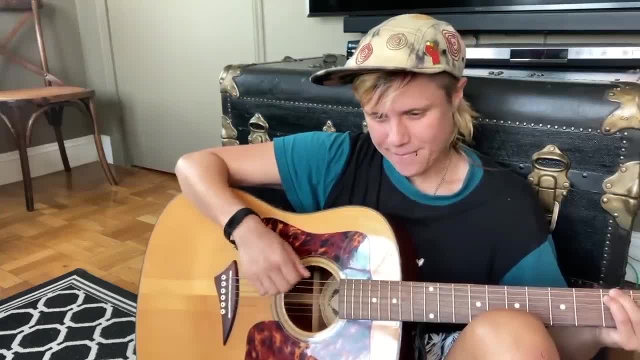 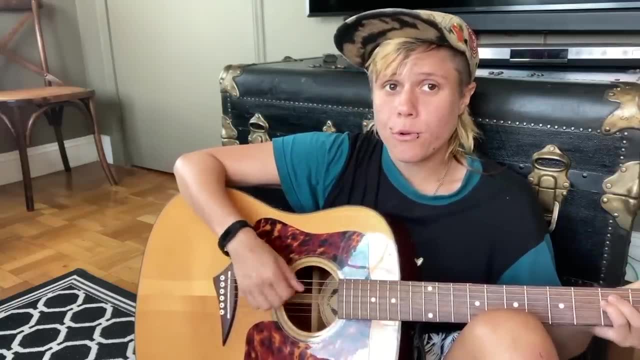 In my crabby, crab mood. I have to walk it through And breathe, And I know I'll feel better soon, Pretending I'm a crab In the ocean blue. Yes, I'll put one hand back, One leg back. 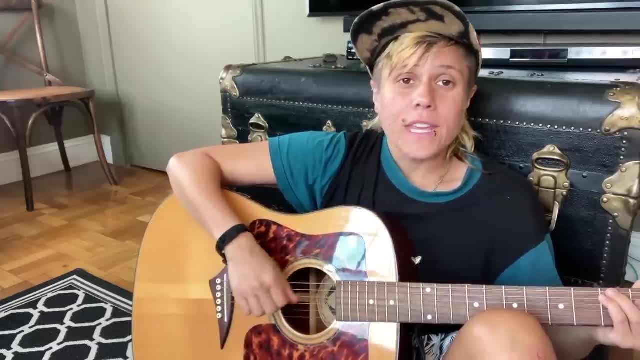 Do it again Now. I'm in a terrible mood. I'm feeling like a crabby crab. I don't know what to do. Swim, swim, swim. You didn't trick us, Mrs Fish. We knew it was you. 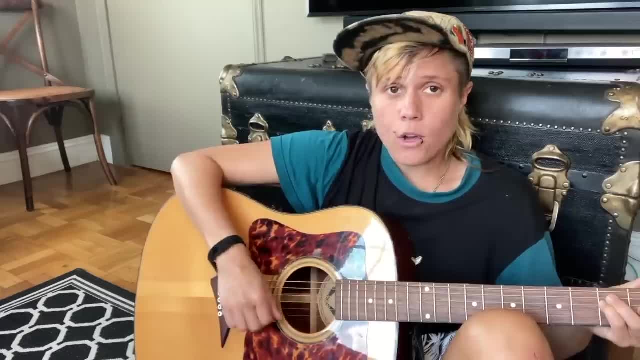 We knew it was you. We knew it was you. Swim, swim, swim. I'm feeling like a crabby, crabby crab. One hand back, One leg back, One leg back. Do it again Now. I'm feeling like a crabby crab. 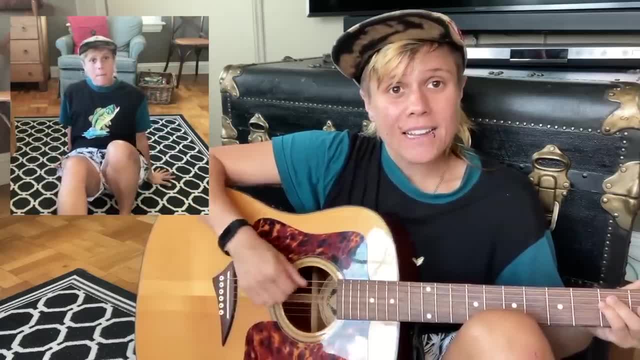 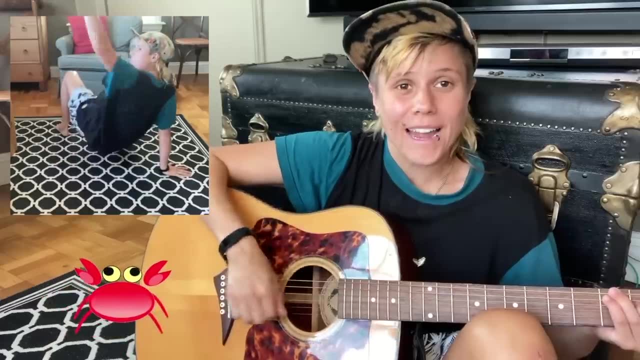 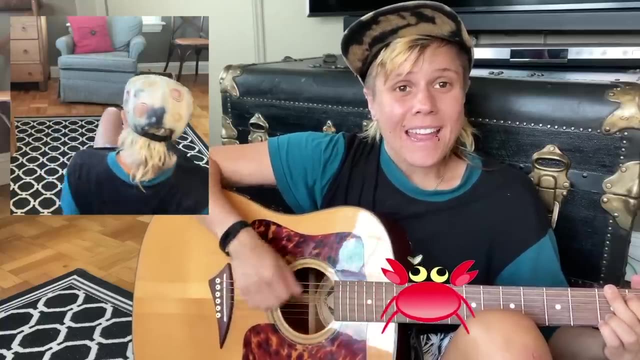 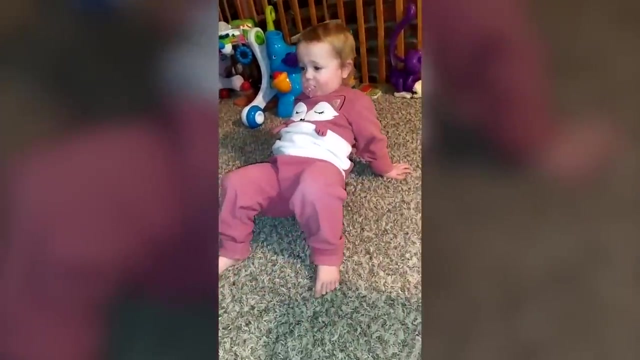 One leg back, One leg back, One leg back. Do it again. Now I'm walking like a crabby crab. One hand back, One leg back. Do it again. Now I'm walking like the crabby crabs. do Wow, I feel so much better. 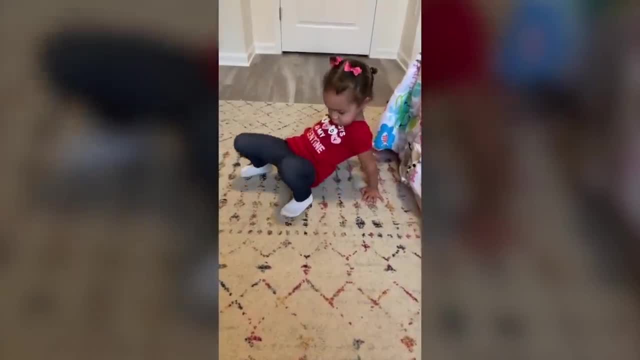 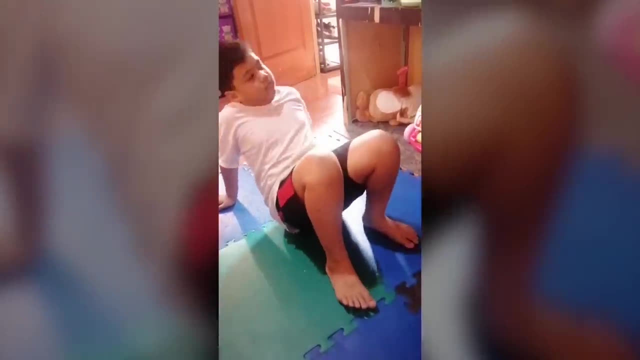 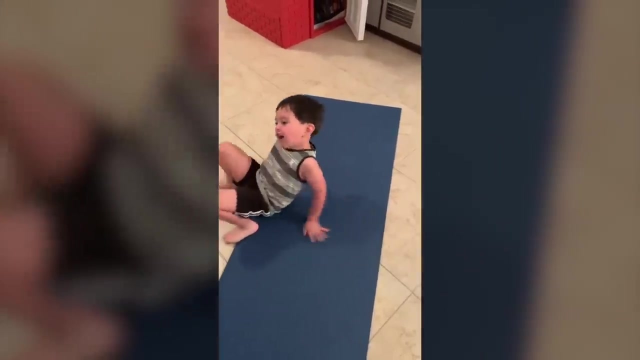 Let's keep walking. One hand back, One leg back. Do it again Now. we're walking like the crabby crabs. One hand back, One leg back, One leg back. Do it again Now. we're walking like the crabby crabs do. 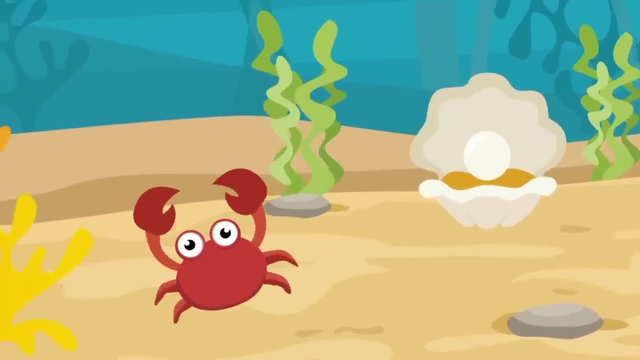 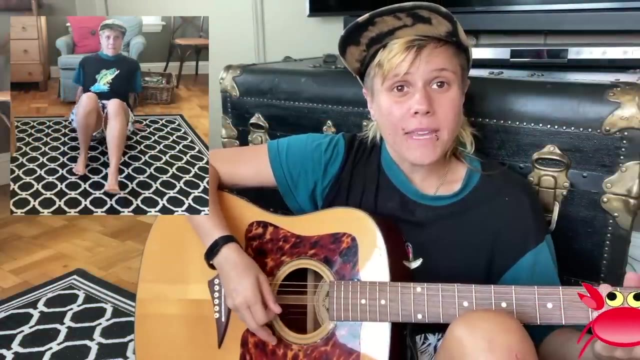 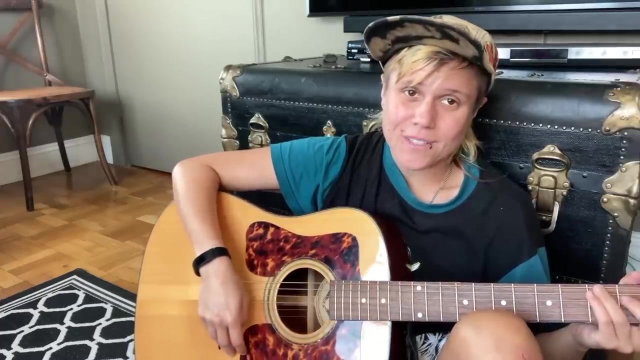 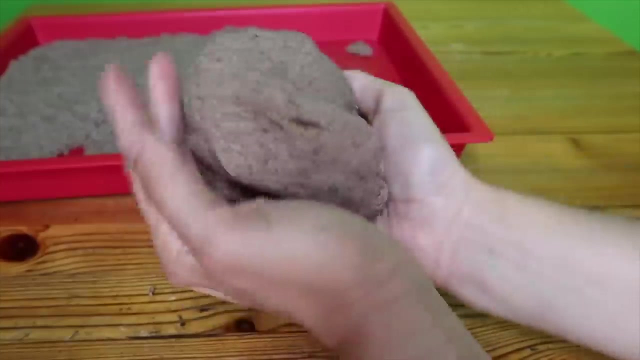 Walking like a crabby crab. do I feel so much better? Hmm, I wonder who's in this sandball, Who's hiding? Here's your clue: Boop, It's yellow. Do you remember what one of our ocean animals was? yellow? 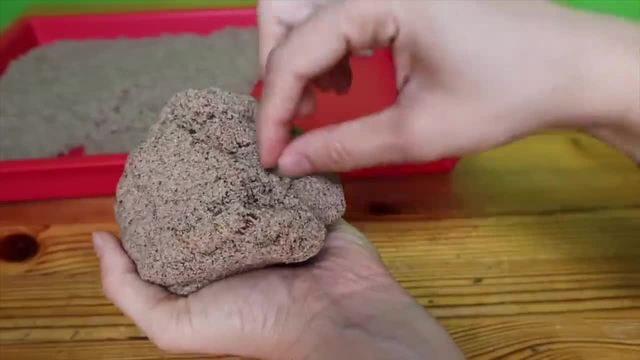 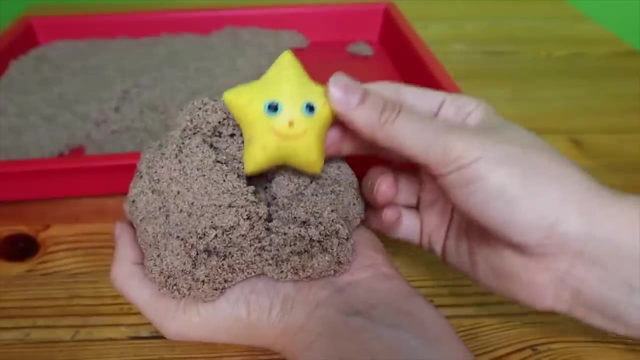 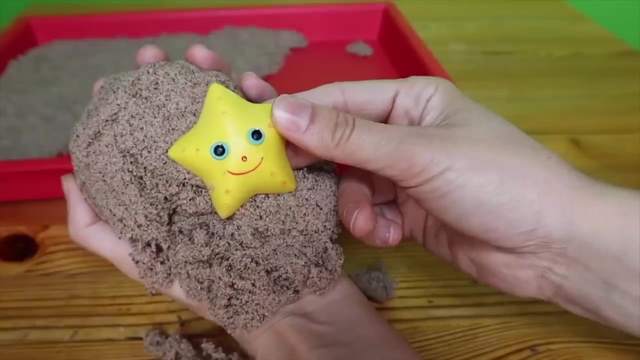 Hmm, it's the starfish. Oh, you found me. I was hiding. Did you know? it was me? when you saw the color yellow, We did. You didn't fool us, starfish, Who thinks hiding this ball? I'll give you a clue. 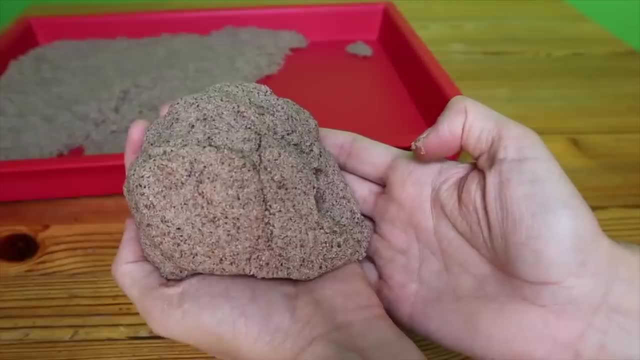 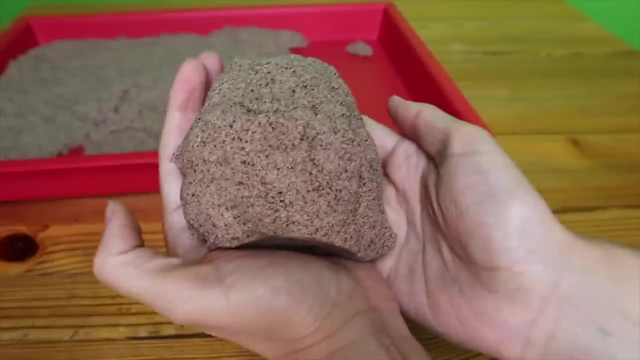 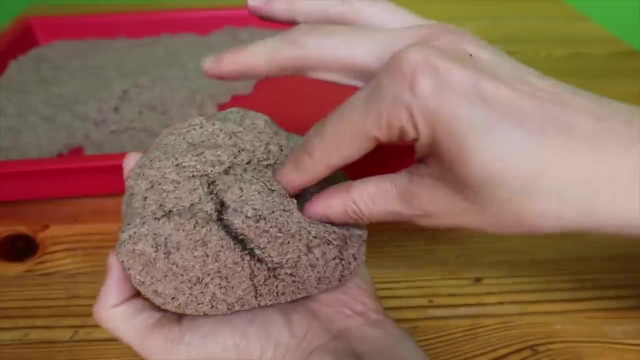 It begins with the letter T T T, T T T T. And here's a little clue: we can see him peeking out. Oh, did you see that? Did you see that? It's a turtle. 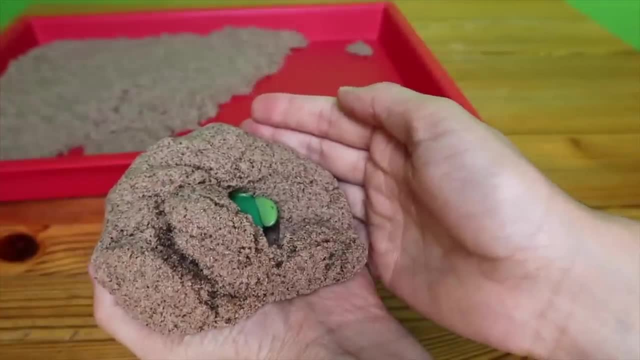 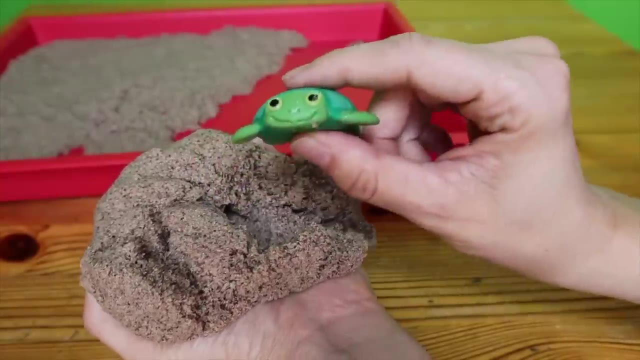 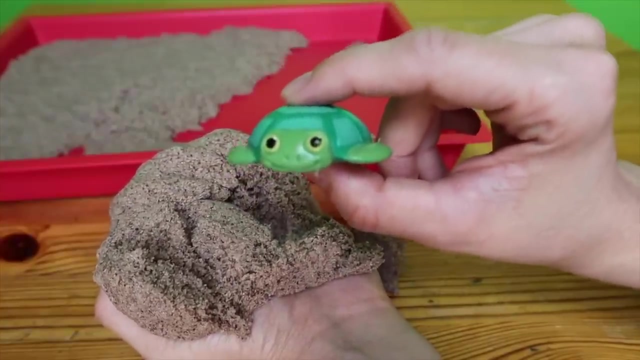 Oh no, it's stuck. Say out and we'll get him out Out. Oh, Thank you so much. I was stuck. You're so nice, Did you know it was me a turtle? We did because we saw the green and we knew that it started with a T. 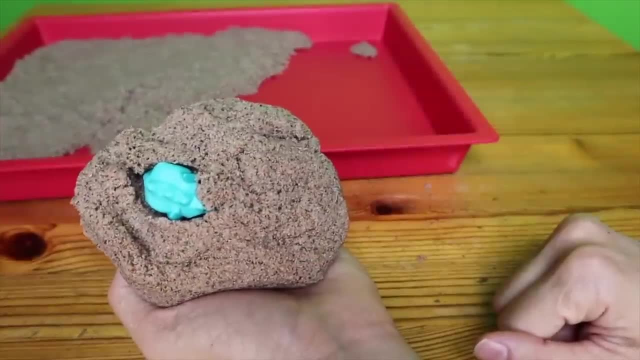 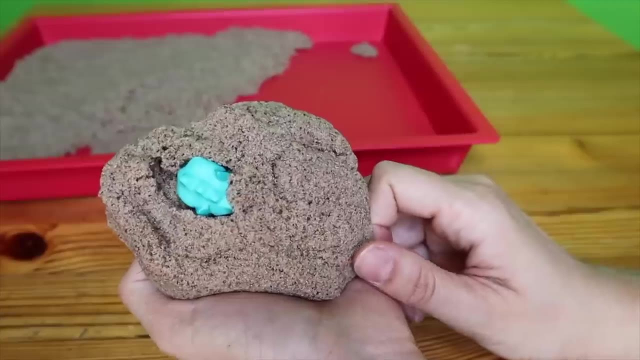 T T turtle. Who do you think's in our last ball? Oh my, She is peeking out. Hmm, Well, the octopus was blue, but we already found the octopus. Do you think it's another octopus? 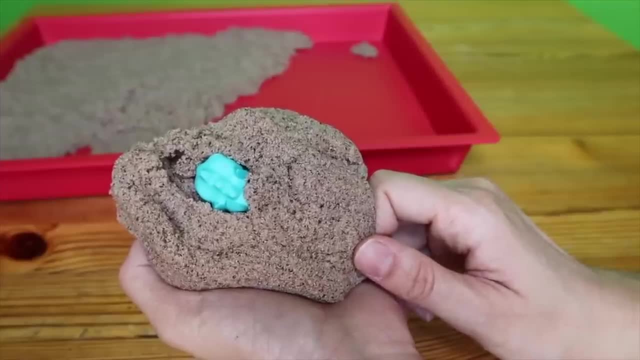 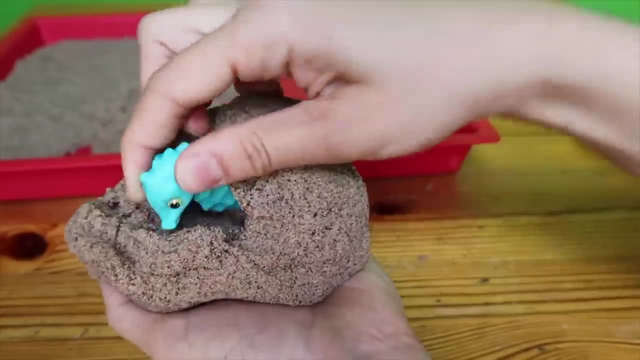 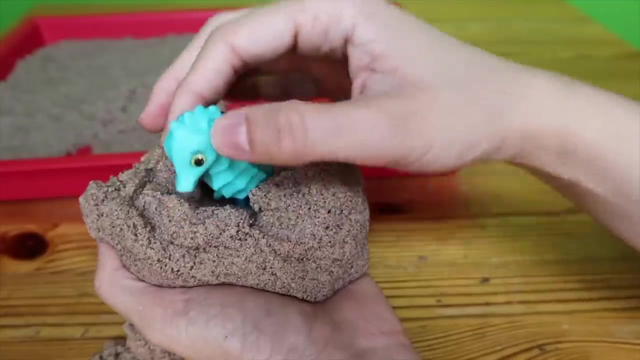 What other animals did we have? Hmm, Let's get out a little more and see what we think Out out out. Do you recognize this little animal? It's a seahorse. Wow, Hello, I'm a seahorse. 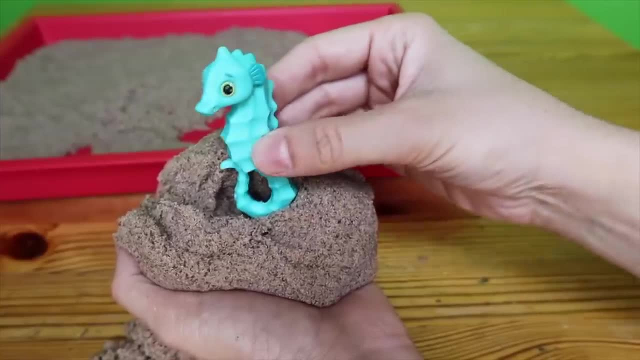 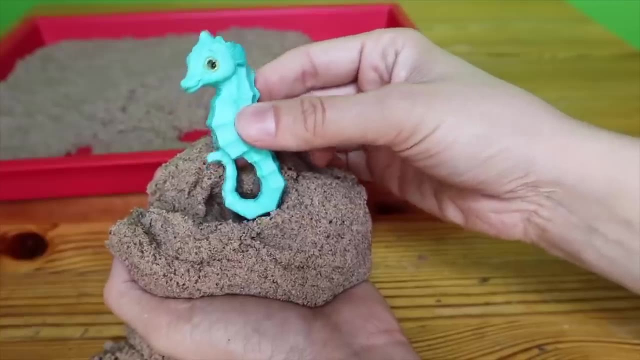 Did you know it was me or did you think it was the octopus? We thought it might be an octopus because it was blue like the octopus, but we knew it was you. Thank you for finding me. Oh, she gave us a kiss. 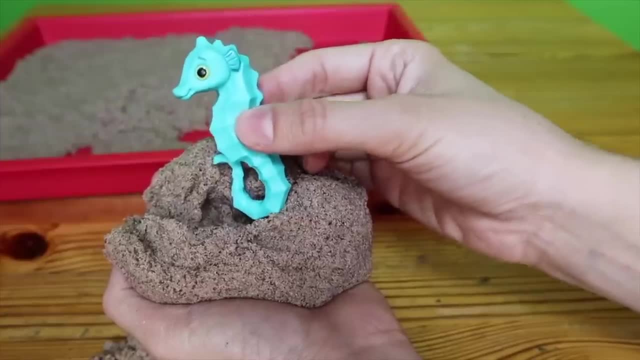 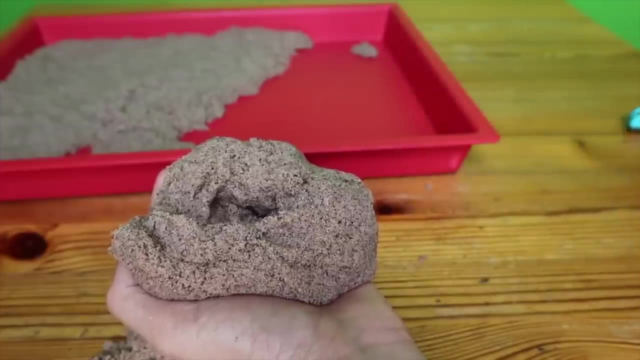 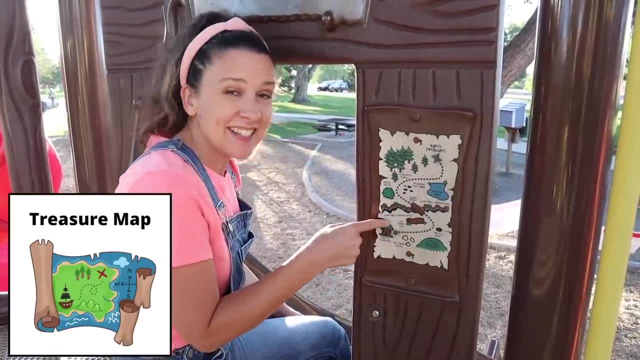 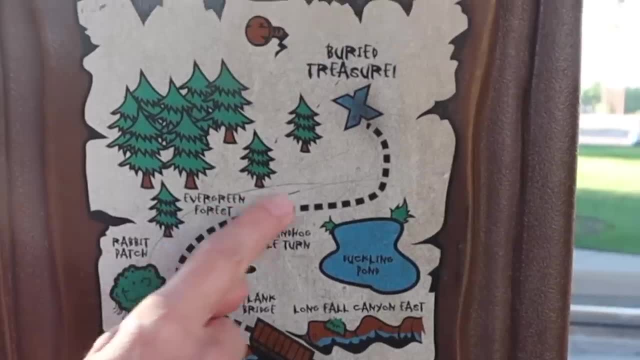 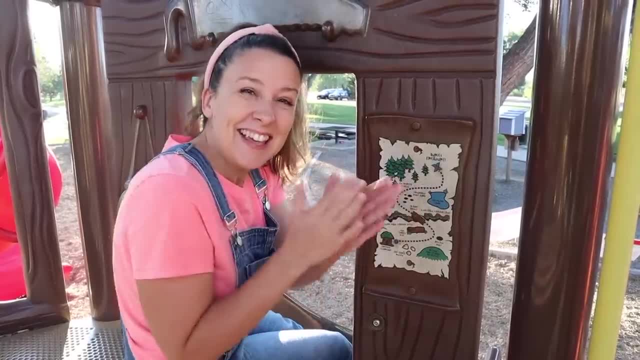 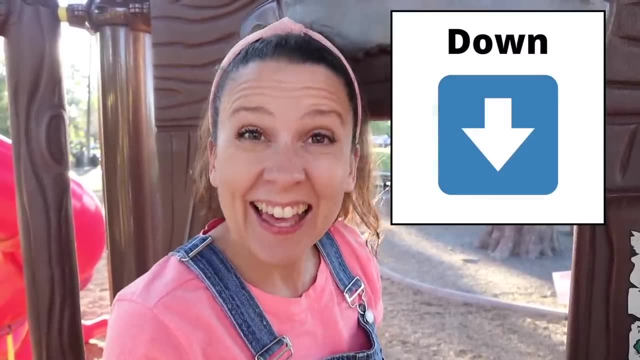 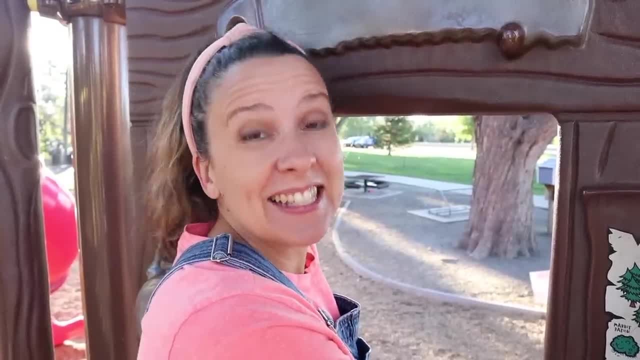 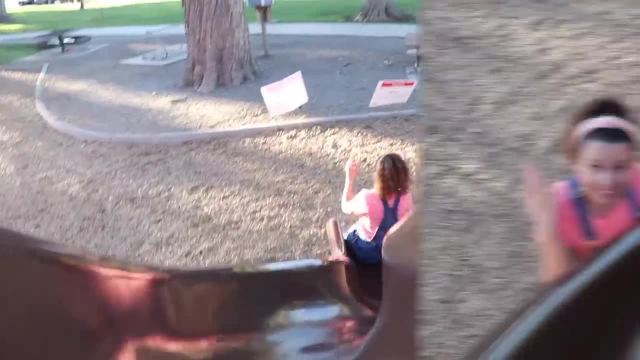 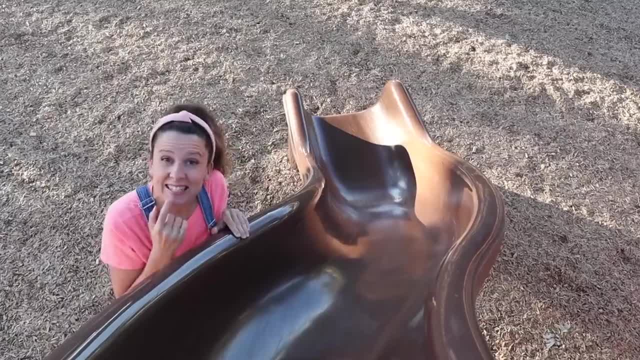 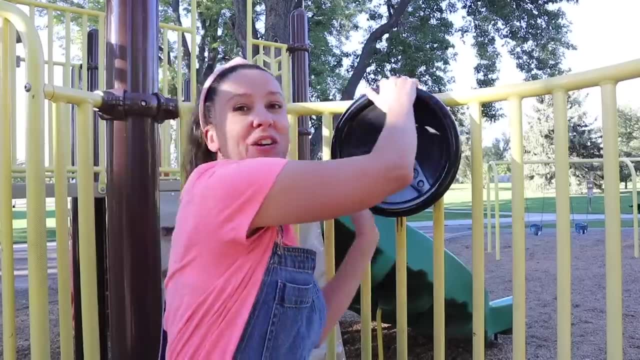 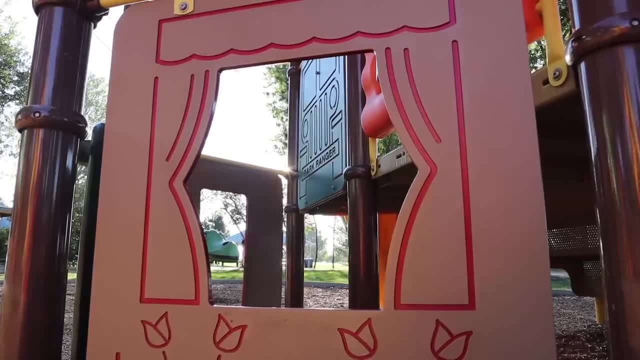 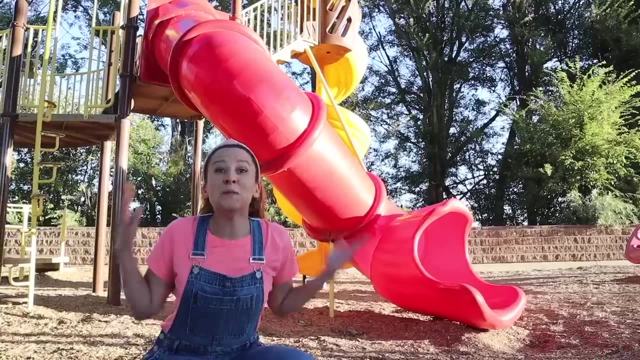 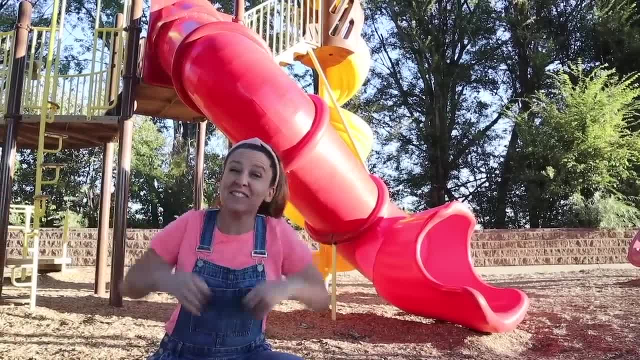 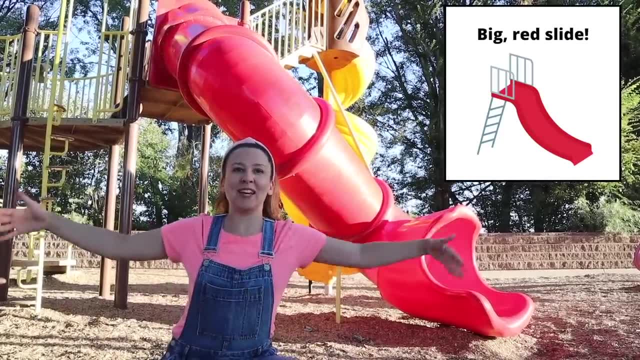 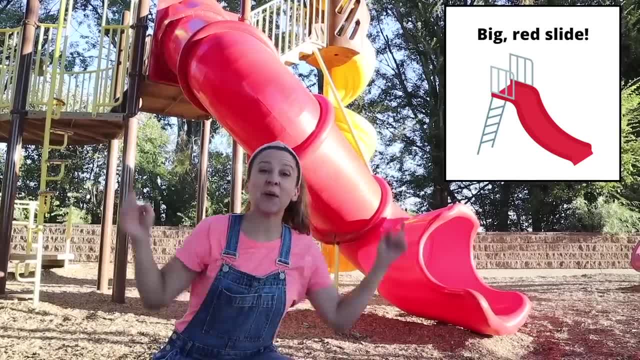 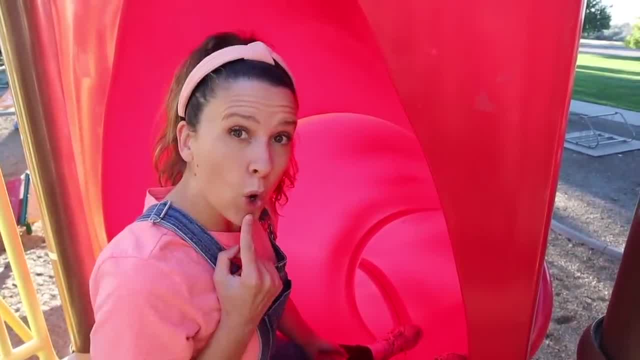 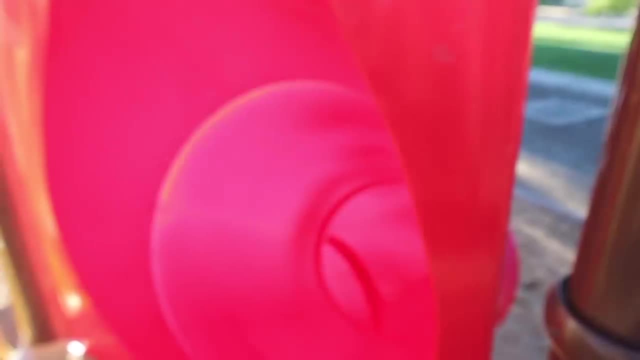 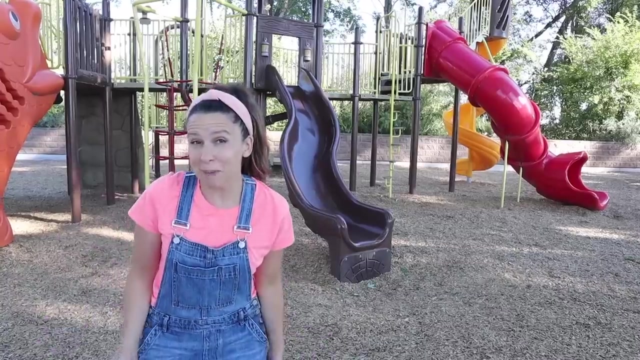 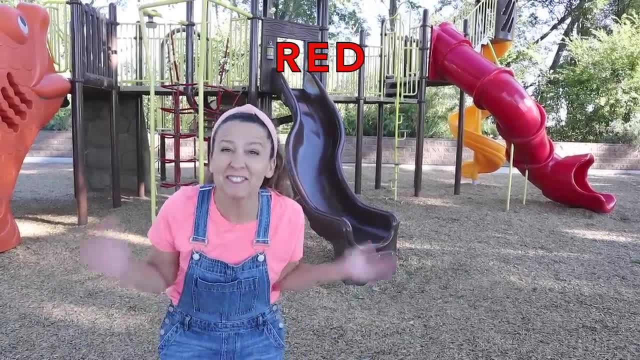 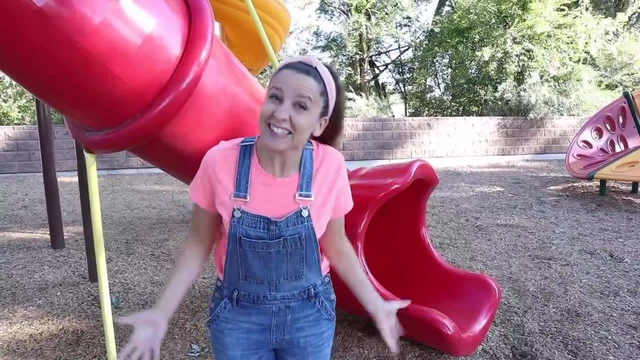 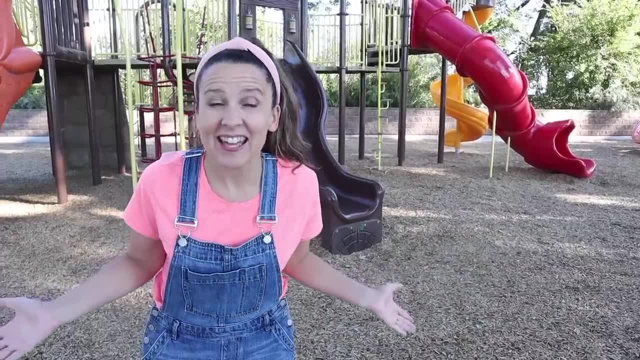 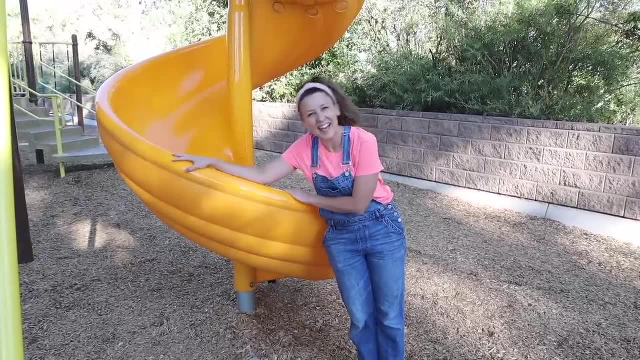 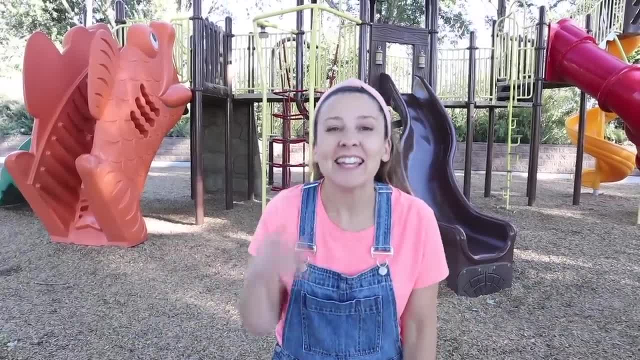 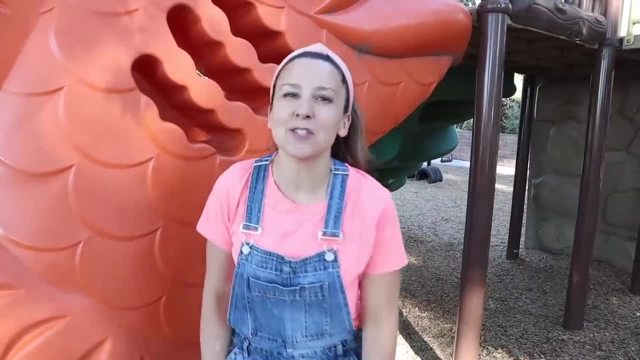 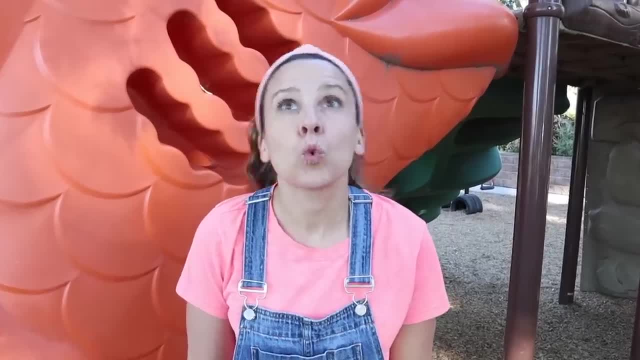 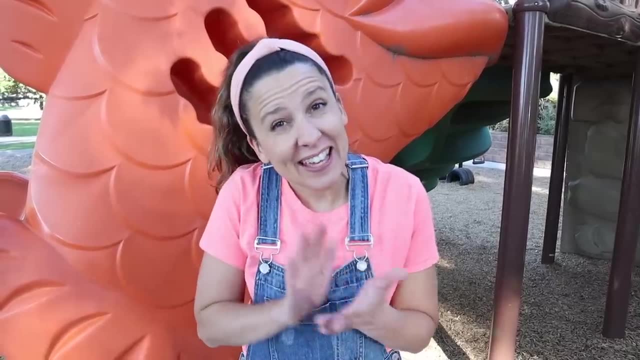 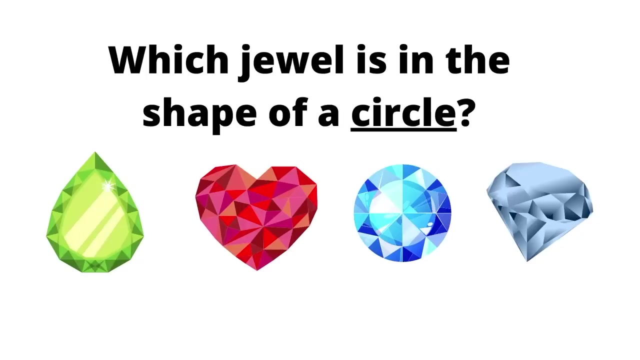 I'm a treasure, I'm a treasure, I'm a treasure. Can you kiss like a fish? Good job, Great job playing. I Spy Now which jewel is in the shape of a circle? Yeah, that one, That's a circle. 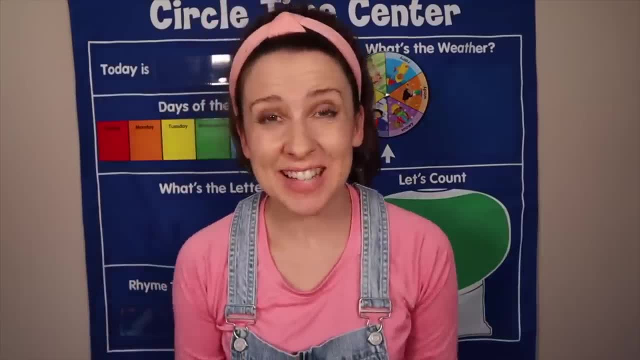 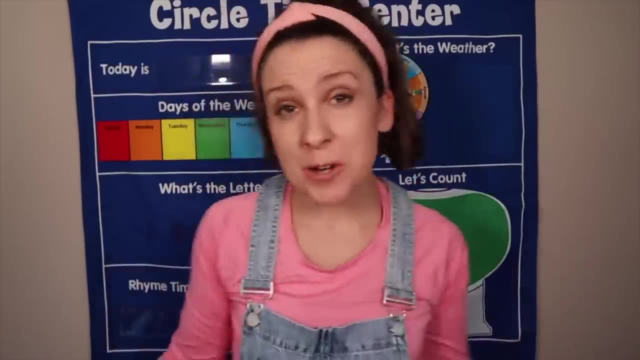 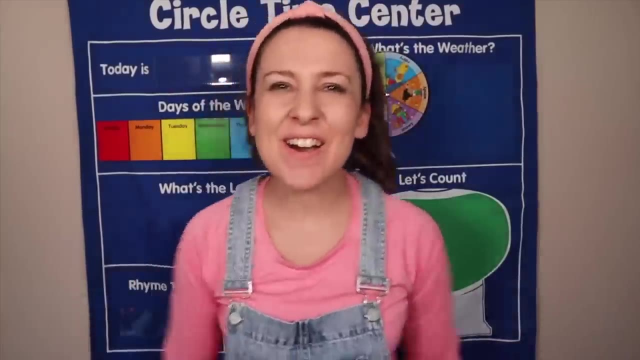 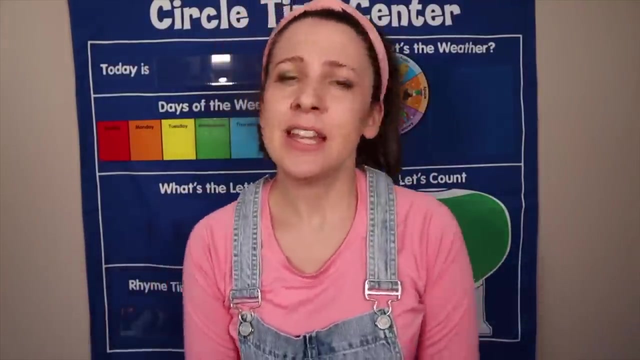 Good job. Now we're ready to sing Down by the Bay with the piano and guitar. Down by the bay, Down by the bay Where the watermelons grow. Back to my home, I dare not go, For if I do My mother will say: Did you ever see a goose kissing a moose? Down by the bay? 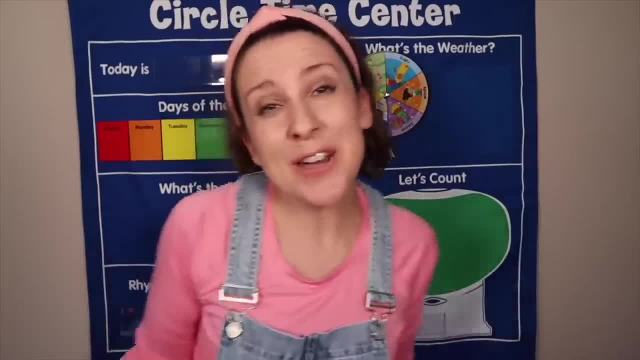 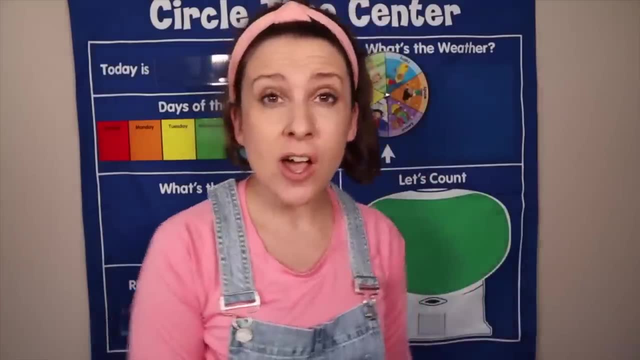 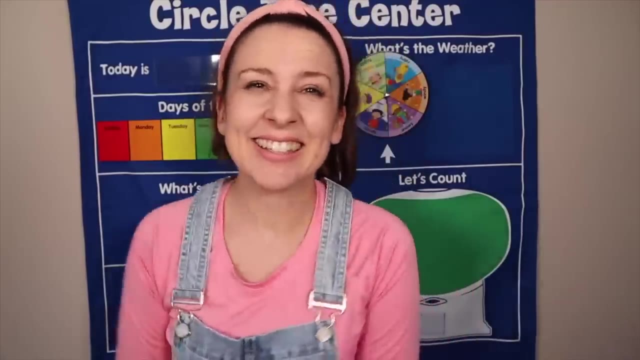 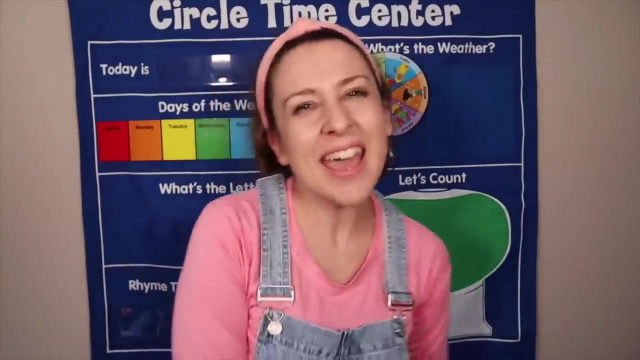 Down by the bay Where the watermelons grow, Back to my home. I dare not go. I dare not go, for if I do, for if I do, my mother will say. my mother will say: did you ever see a whale with a polka dot tail? Down by the bay, down by the bay, down by the bay. 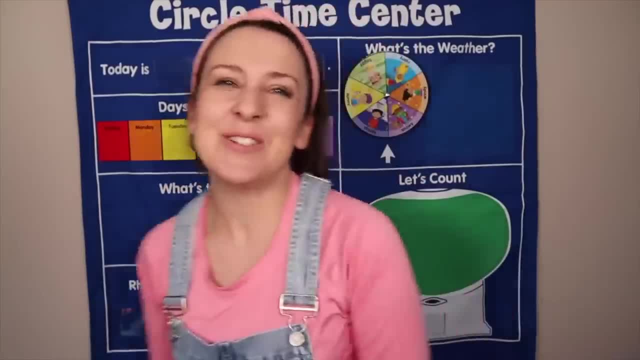 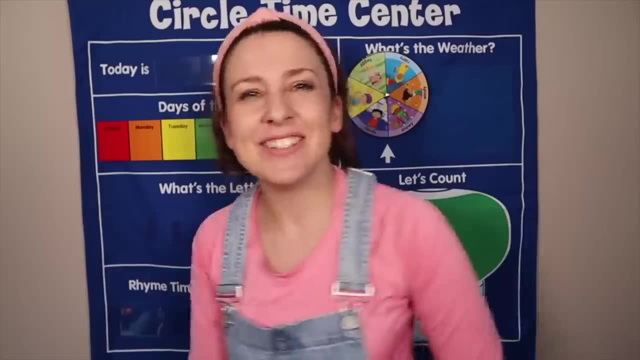 where the watermelons grow, where the watermelons grow, back to my home, back to my home, I dare not go. I dare not go, for if I do, for if I do, my mother will say, my mother will say: 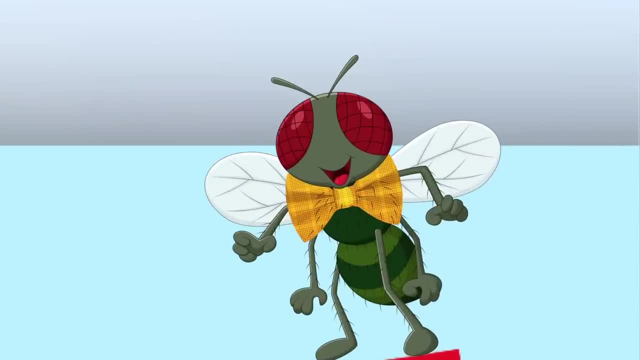 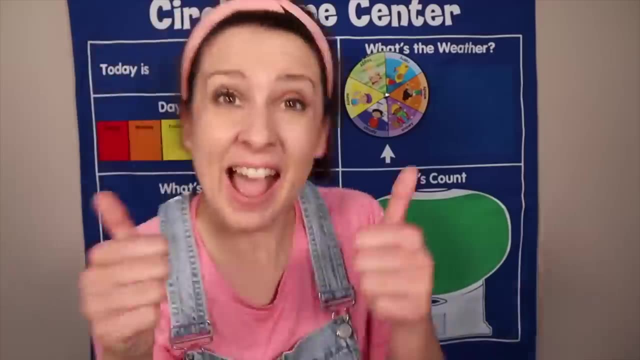 did you ever see a fly wearing a tie? Down by the bay, down by the bay, down by the bay where the watermelons grow, where the watermelons grow? back to my home, back to my home. I dare not go. 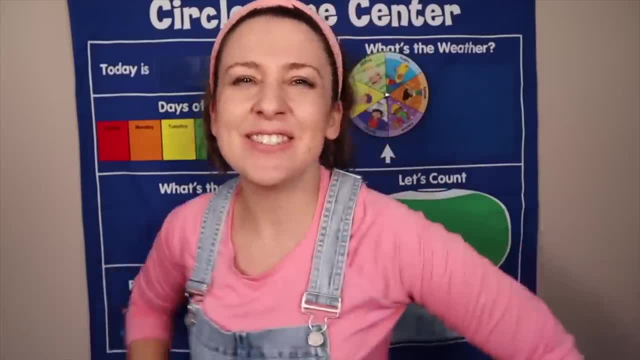 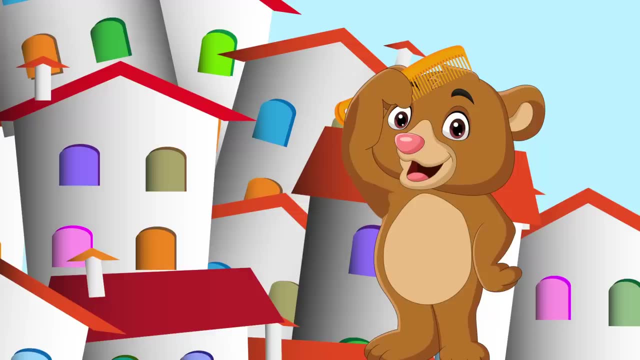 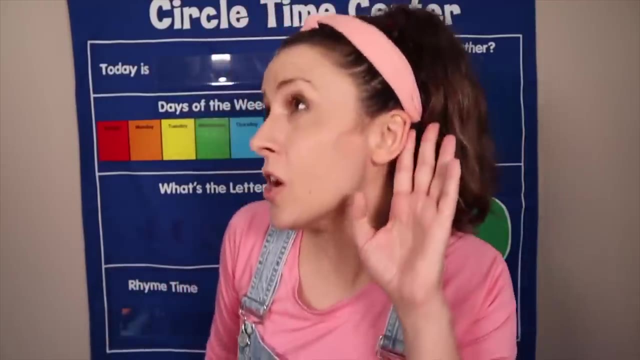 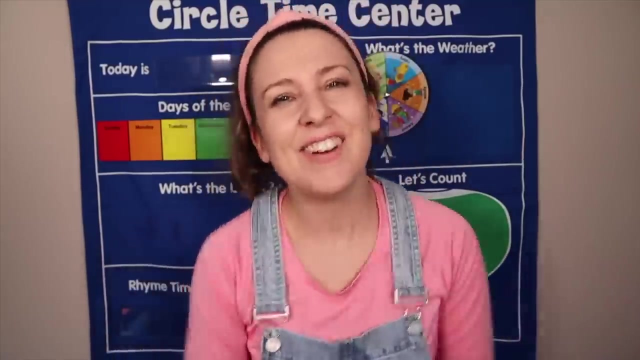 I dare not go, for if I do, my mother will say: my mother will say: did you ever see a bear combing his hair? Down by the bay, down by the bay where the watermelons grow, where the watermelons grow. back to my home, back to my home, I dare not go. I dare not go, for if I do, 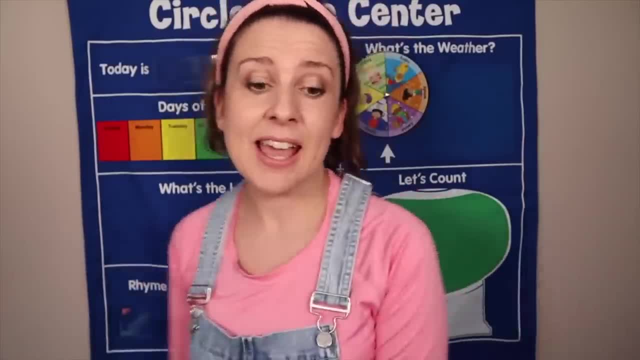 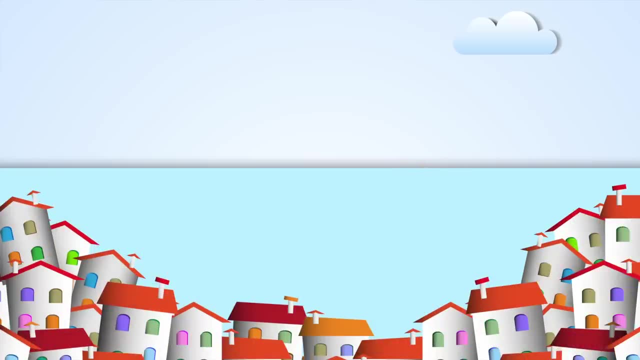 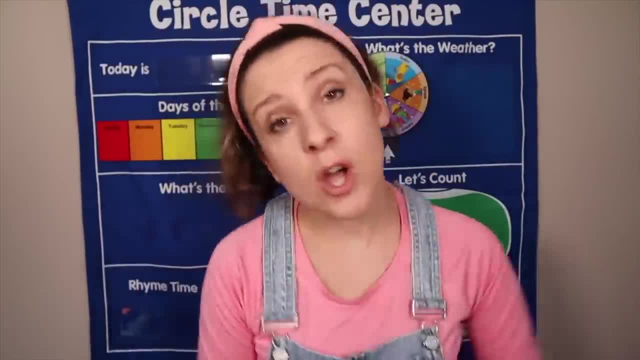 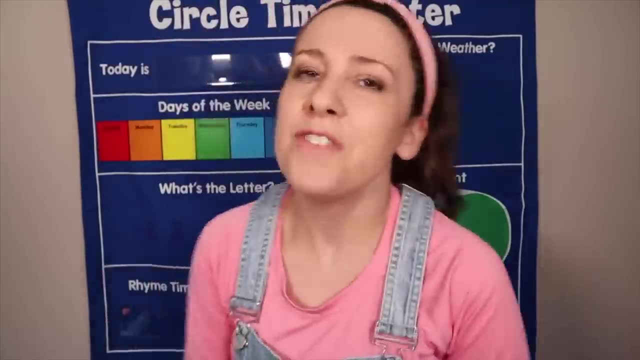 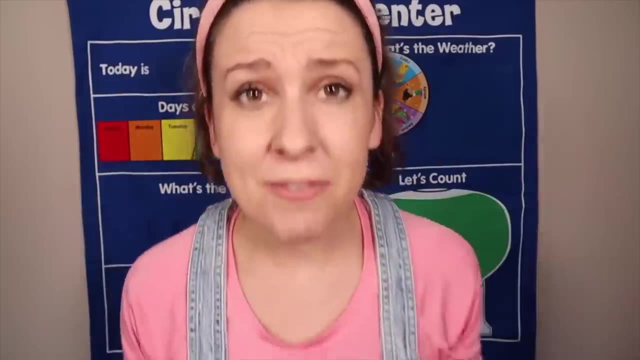 where the watermelons grow, where the watermelons grow, back to my home. back to my home. I dare not go. I dare not go, for if I do, my mother will say: did you ever have a time where you couldn't make a rhyme? 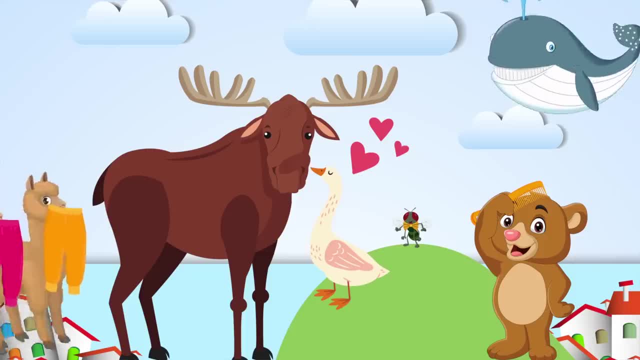 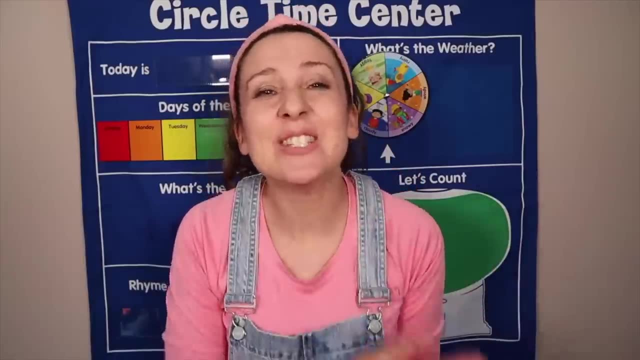 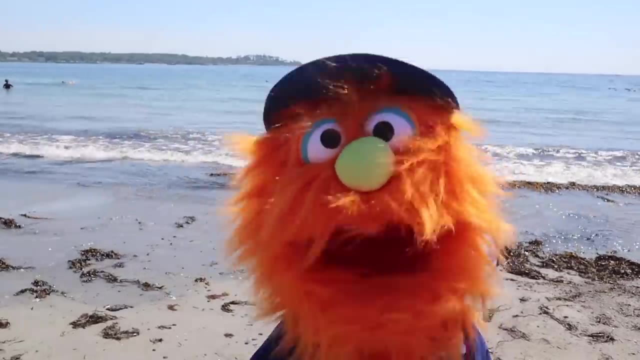 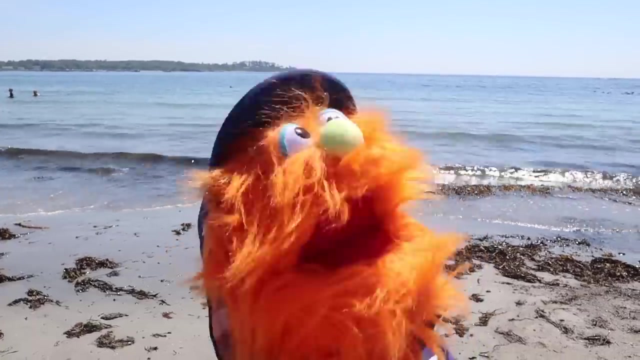 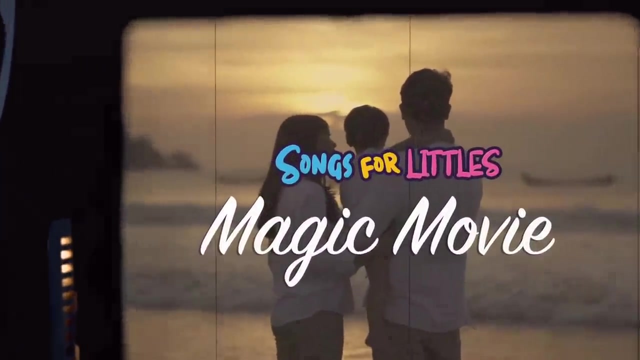 Down by the bay. Yay, That was so much fun. What's the difference between a fish and a piano? You can't tuna fish, Tuna fish, Guess what? it's time for Our magic movie. What do you see? 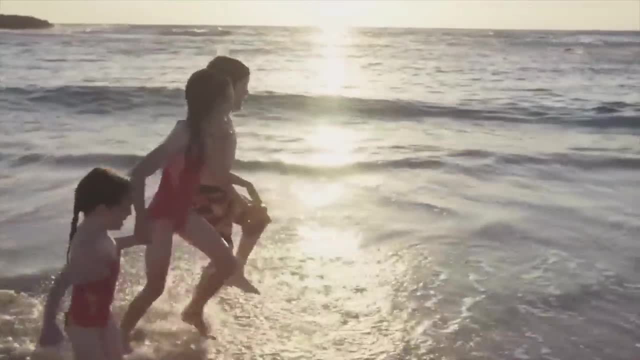 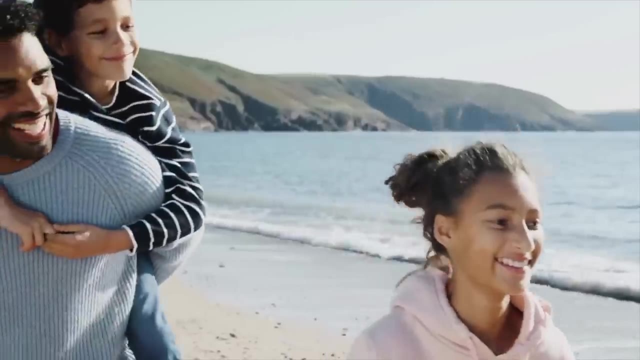 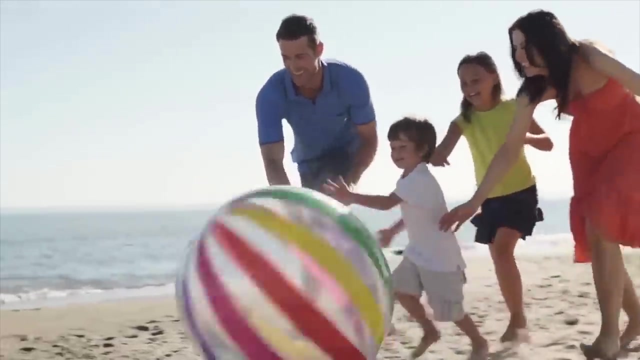 I see children running through the ocean, splashing in the water waves. That looks like fun. This family looks happy. They're running on the beach together. This family is playing with a ball on the beach. Ooh, what do you see? 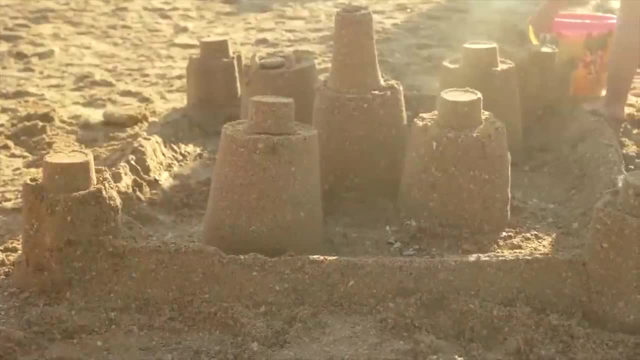 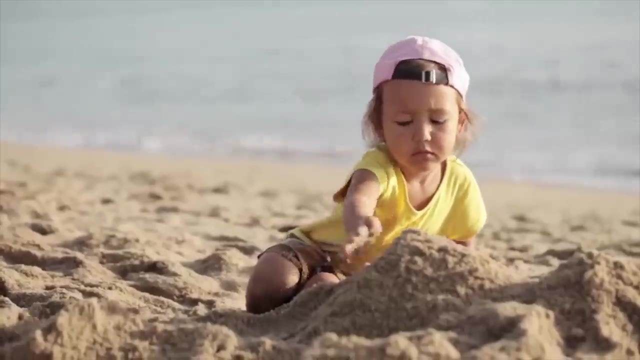 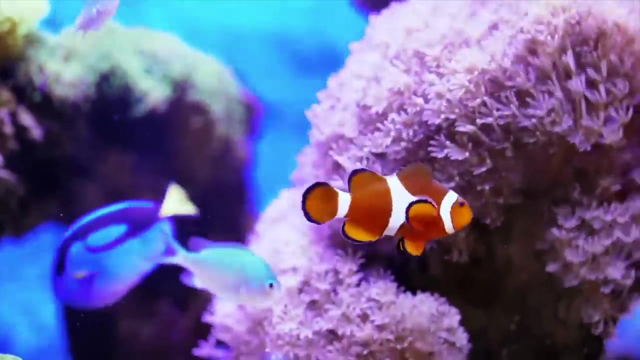 I see sandcastles. It's fun to build sandcastles. Oh, one little girl is patting the sand. Pat, pat, pat. Ooh, now we're underwater. I see a fish. Do you see one? It looks kind of like Nemo. 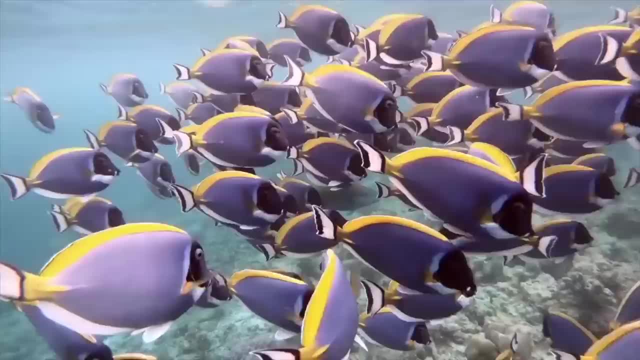 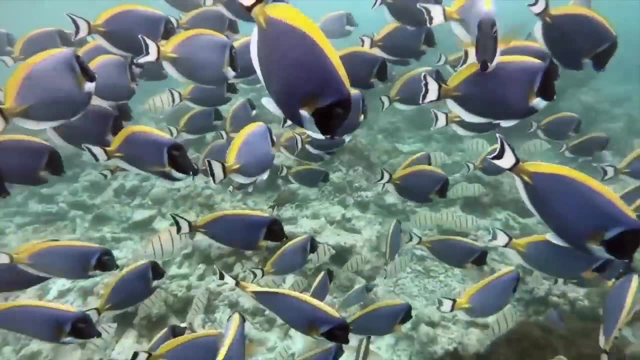 And the other fish in the back looks kind of like Dory. Oh wow, I see many fish. There are lots of fish swimming together. That's called a school of fish. Oh wow, Do you see the seahorses? 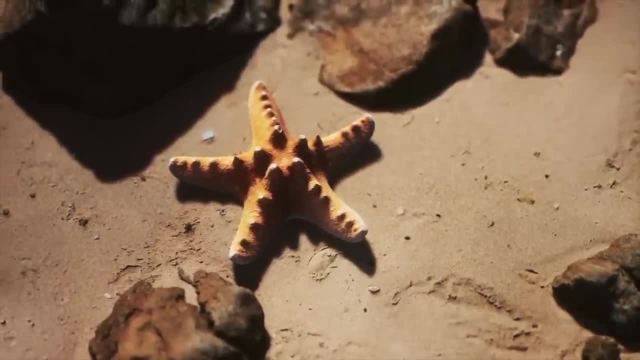 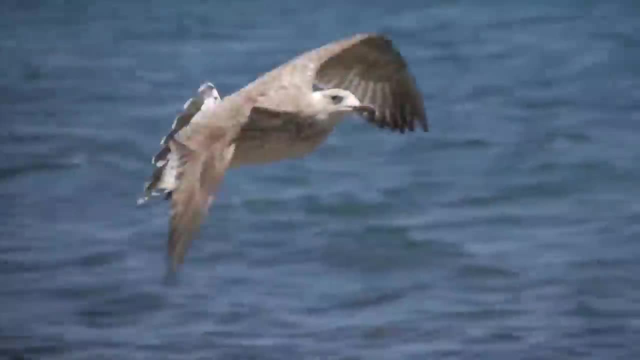 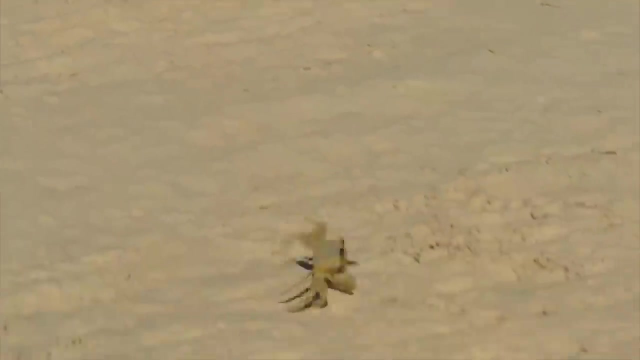 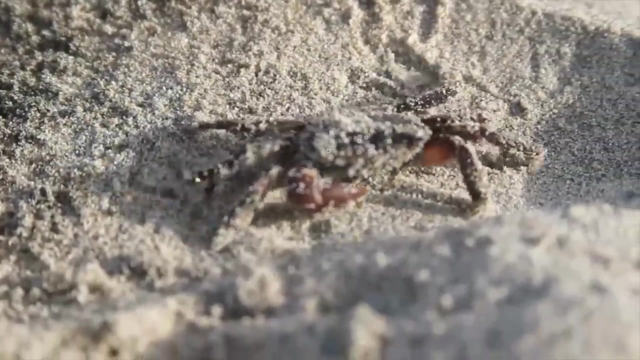 What's that? It's a starfish. Wow, Do you know what kind of bird that is? Yeah, it's a seagull Running so fast. What is that little animal running so fast? It's a crab. Ooh, this crab's walking kind of slow. 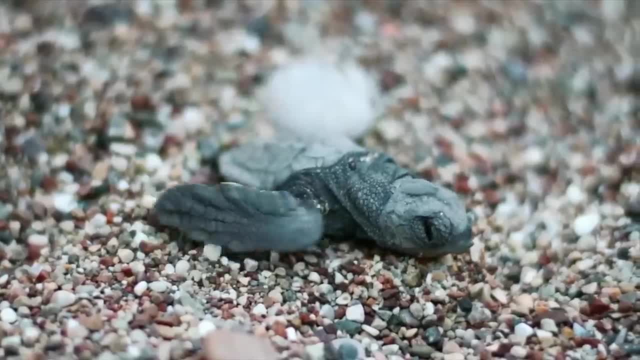 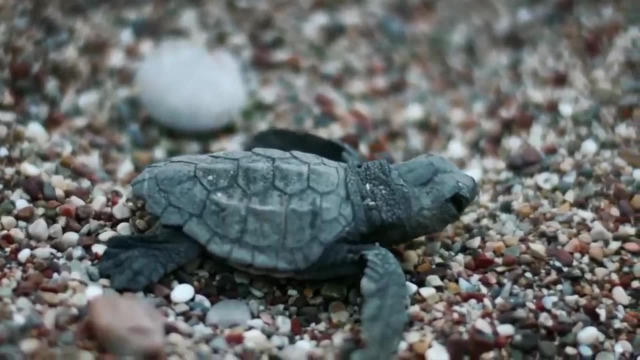 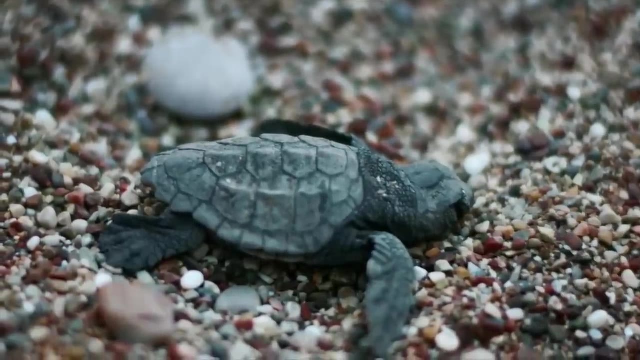 Aww, I see a little baby turtle. So cute, Do you see the turtle? Wow, Wow, there's a lot of pebbles on that beach. Remember, pebbles are little rocks. Wow, that was such a good magic movie about the beach and the ocean. 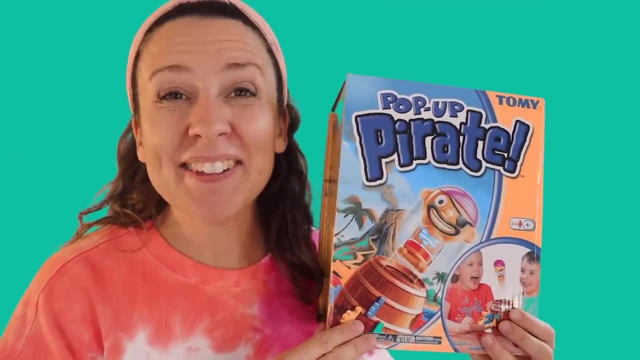 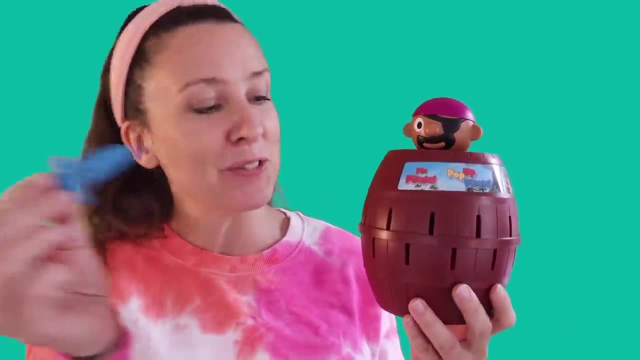 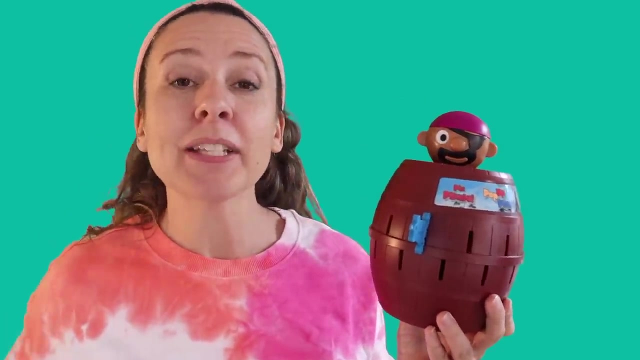 Hi friends, Look, it's Pop-Up Pirate. Let's play together. Let's take turns. You can go first, Put the sword. say in In: Yay, Good job, Now it's my turn. Put the sword in. 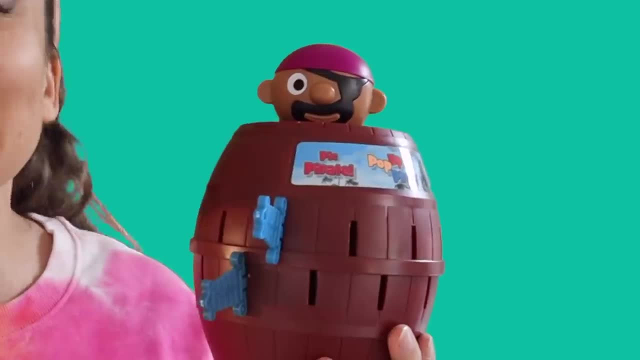 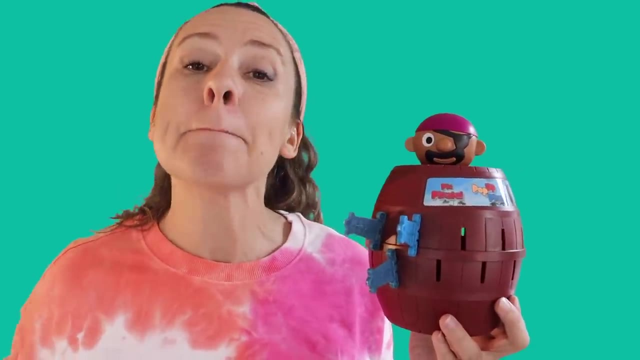 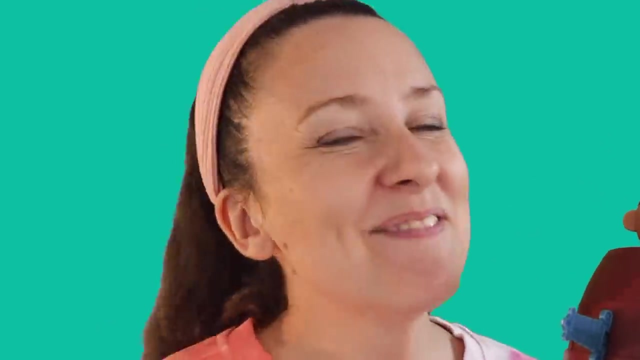 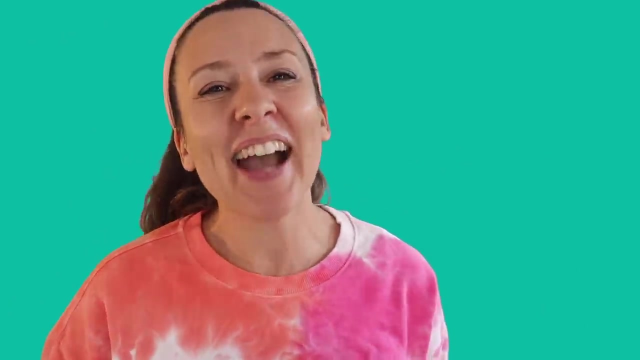 Now it's your turn. Say in: Put it in. You did it, Now it's my turn, Put it in. It didn't pop yet Put it in. Oh, you got it, You popped the pirate, Good job. 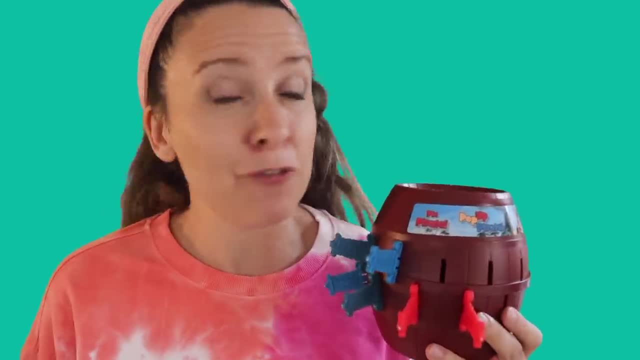 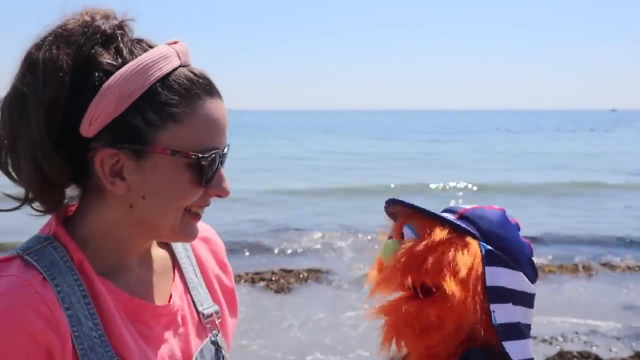 I didn't win this time, but that's okay, It's just fun to play and it's no big deal, Miss Rachel. Miss Rachel, Yeah, I found a triangle Where It's that sailboat. See, look at the sail. 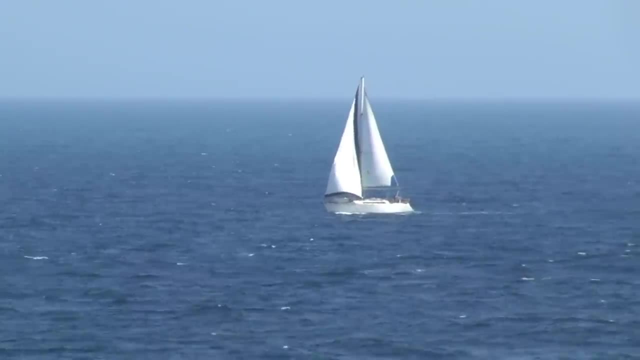 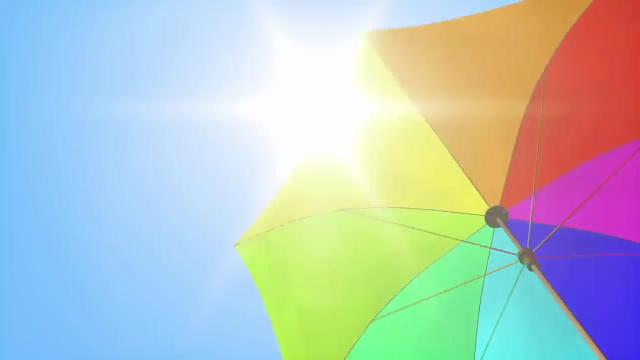 It looks like a triangle. It does great job. I also found a triangle Where It's that umbrella. Oh, I, it's in the umbrella. Yeah, it has triangles on it. Good triangle looking. Can you find any triangles at your house? 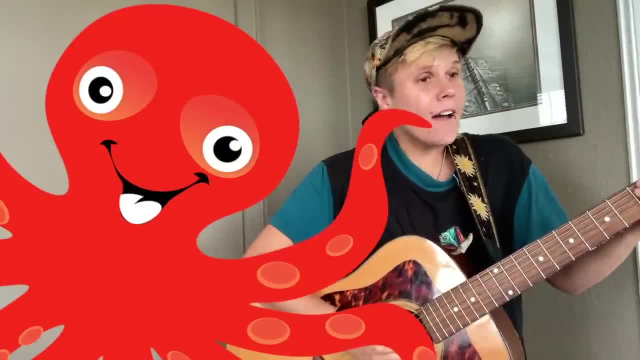 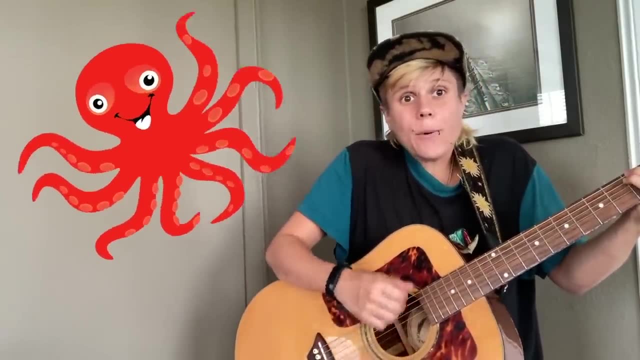 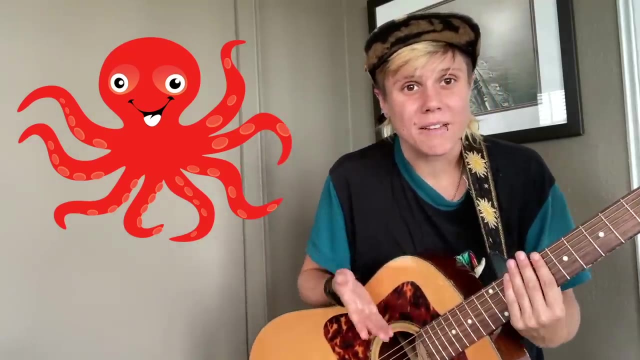 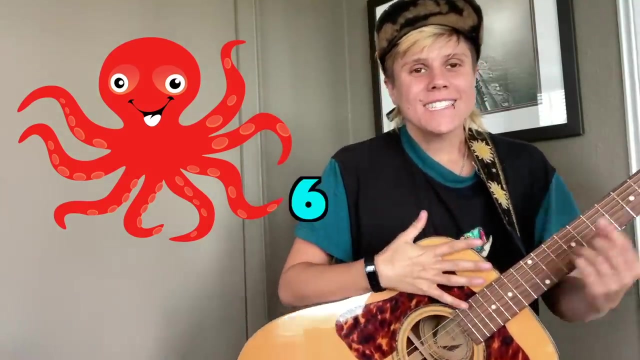 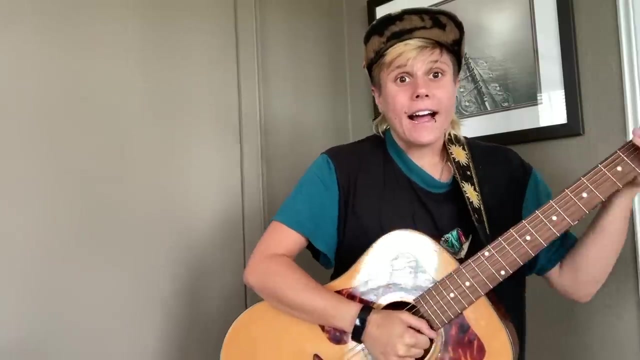 I am a squiggly wiggly octopus. I have eight legs to swim. A squiggly wiggly octopus, wiggly octopus, I have eight legs to swim. stop, let's count them: one, two, three, four, five, six, seven, eight, eight legs. I am a starfish floating through the sea. I have 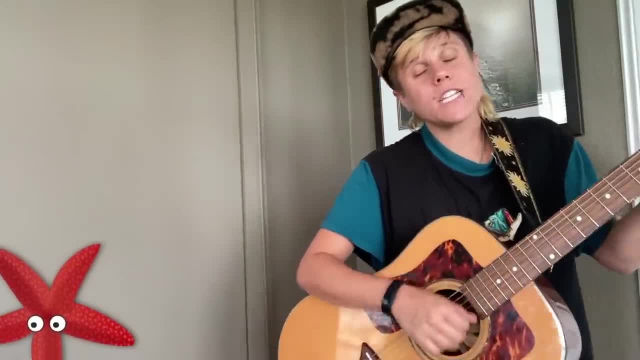 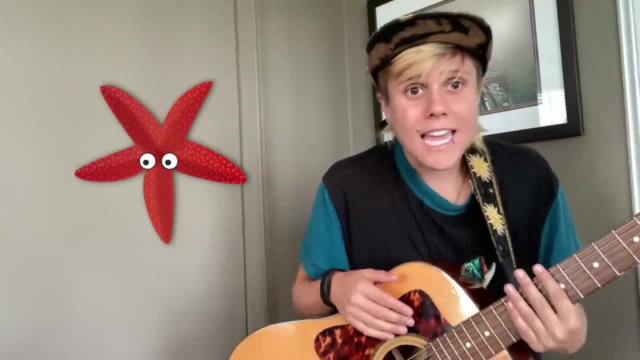 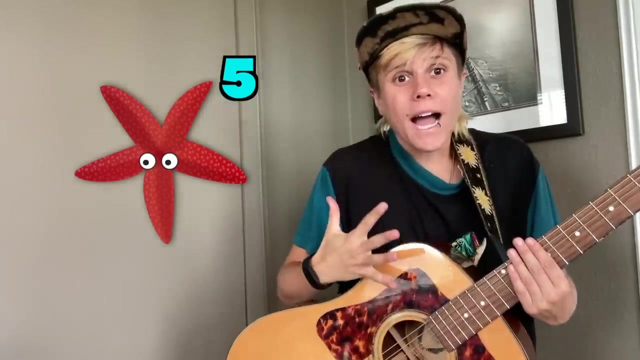 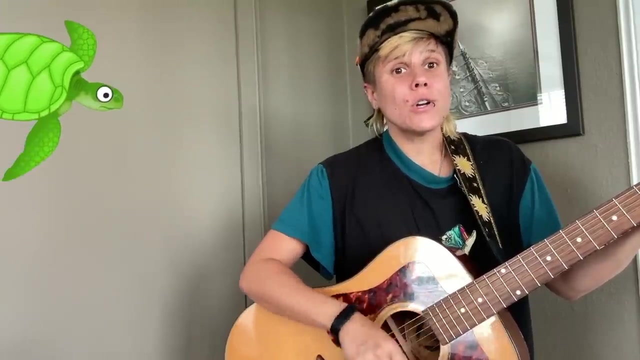 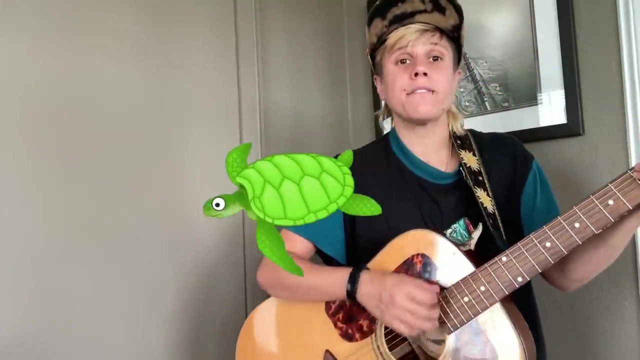 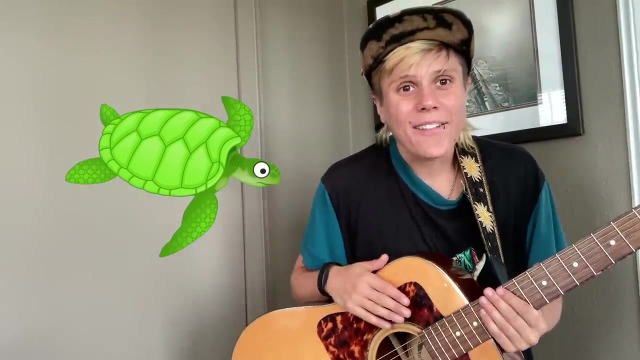 five legs to swim. a starfish floating through the sea. I have five legs to swim. stop, let's count them. one, two, three, four, five, five legs. I am a sea turtle swimming three. I have four legs to swim. stop, let's count them. one, two, three, four, four legs. 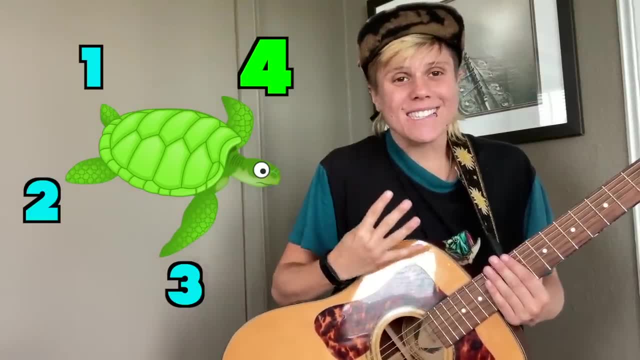 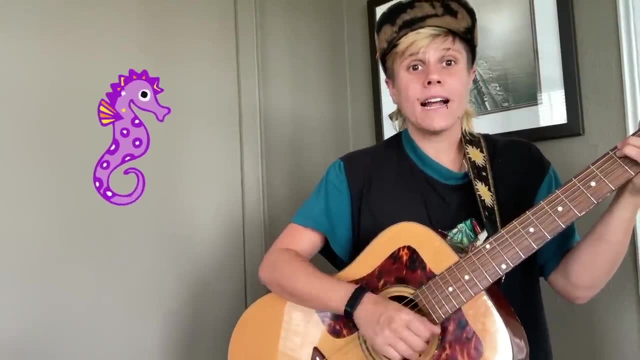 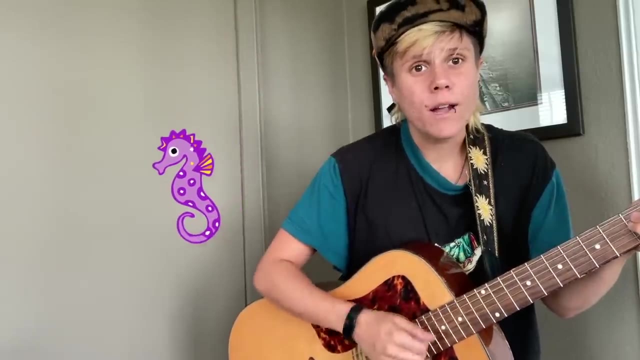 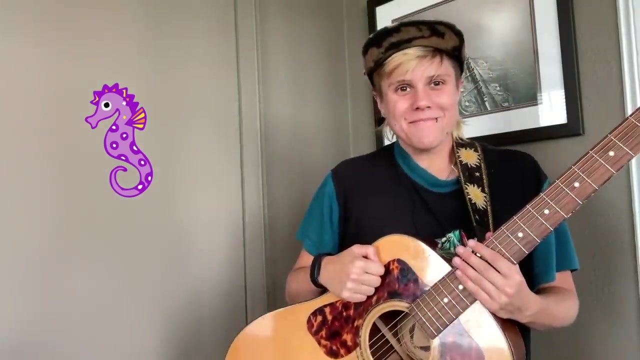 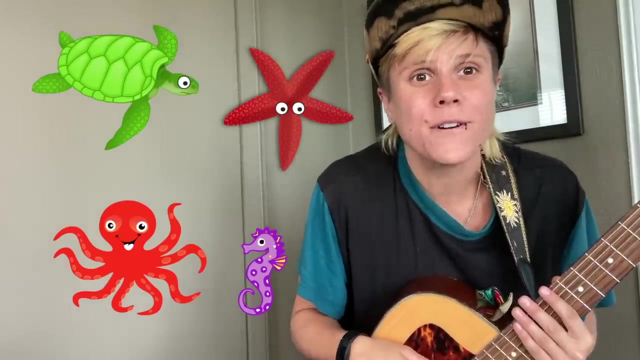 I am a seahorse slowly galloping. I have one leg to swim. a seahorse slowly galloping, I have one leg to swim. leg to swim, stop, let's count it one. y'all did such a good job counting some of the legs of my favorite sea creatures, bye-bye. can you help these animals get? 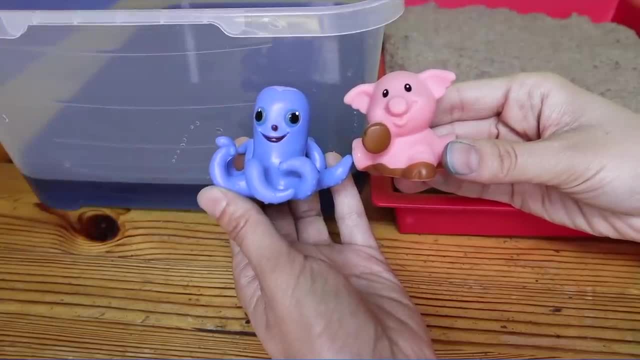 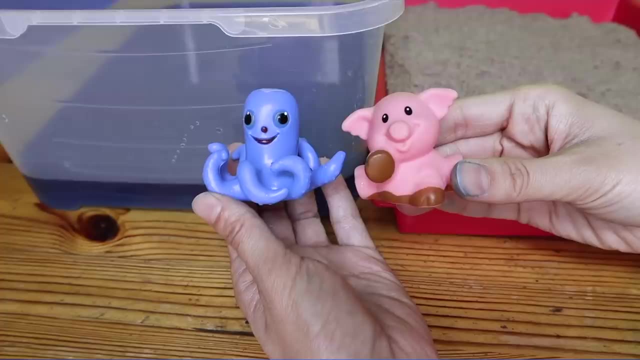 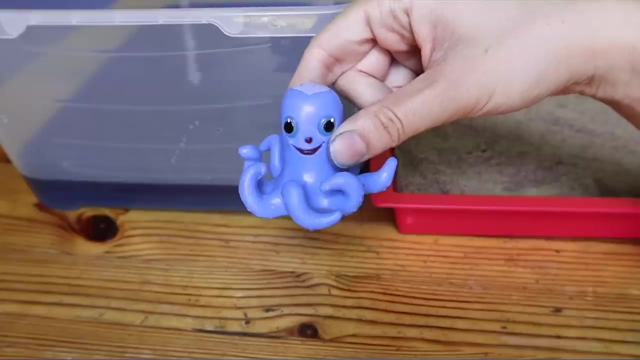 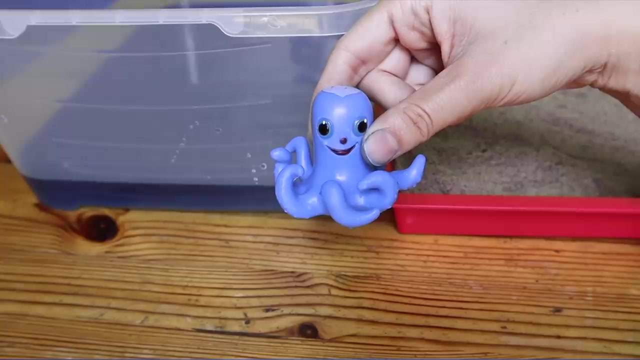 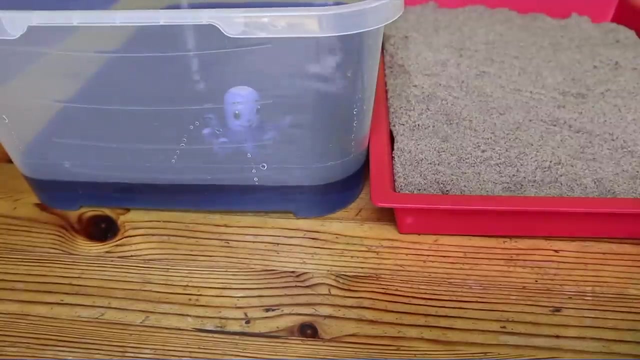 back to their homes. thank you. who belongs in the ocean- the octopus or the pig? yeah, the octopus. let's let the pig go back to the farm. thank you for finding my home. I swim in the ocean. okay, you say in and I'll put the octopus in. put it in, put it in. put it. you said in and the octopus went back. 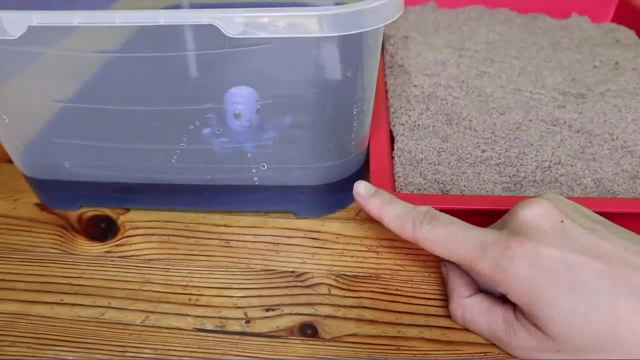 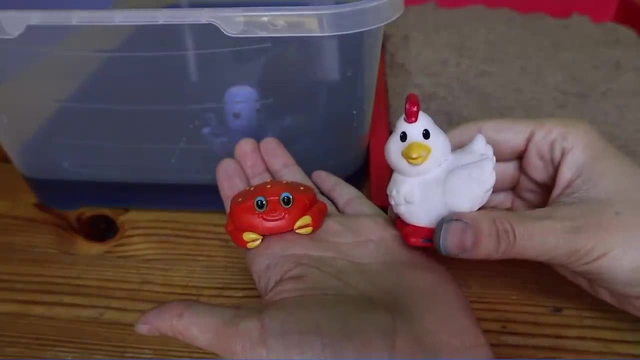 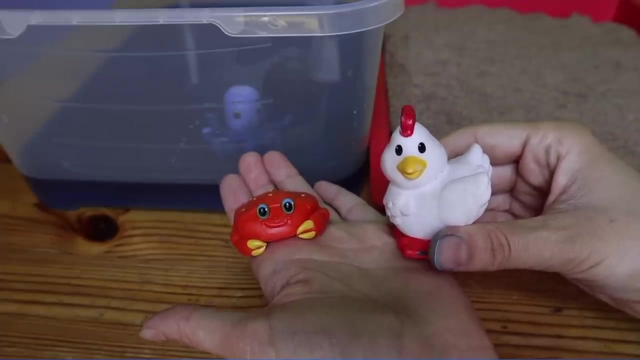 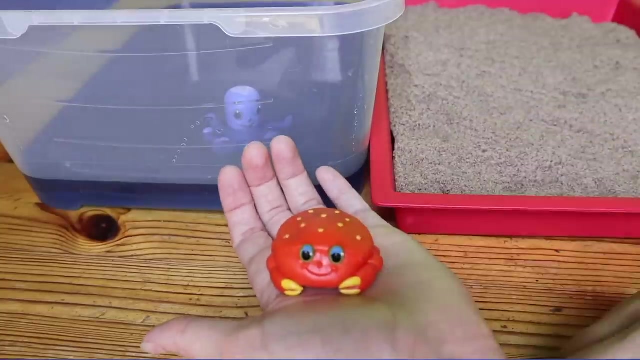 in the ocean. I'm so happy in the ocean. can you help them, these animals, find their home? who belongs in the sand, the crab or the chicken? yeah, the crab. the chicken should go back to the farm. the chicken lives on the farm. so let's say bye-bye chicken, bye-bye chicken, bye-bye. let's put the. 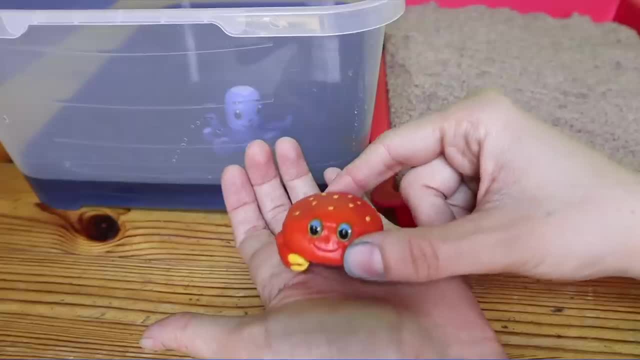 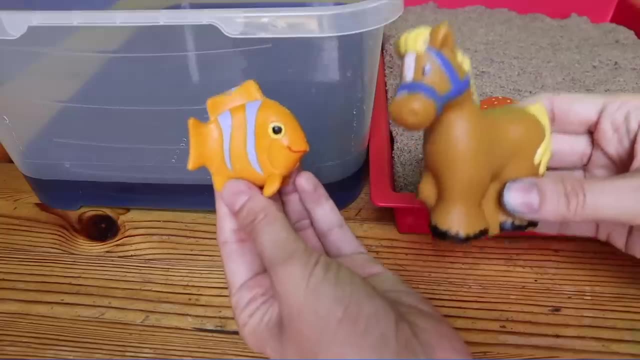 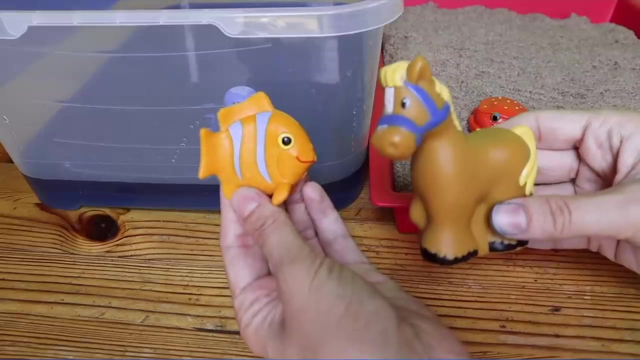 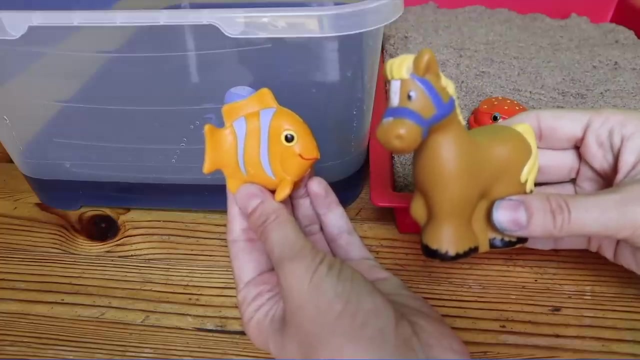 crab on the sand, put it on, put it on, put it on. thank you so much. I love the sand. can you help us find our homes? can you help them? awesome, okay, who belongs in the ocean, the fish or the horse? yeah, the fish. let's let the horse go back to the farm. 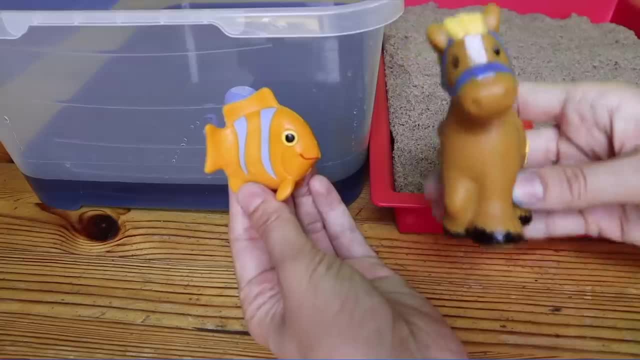 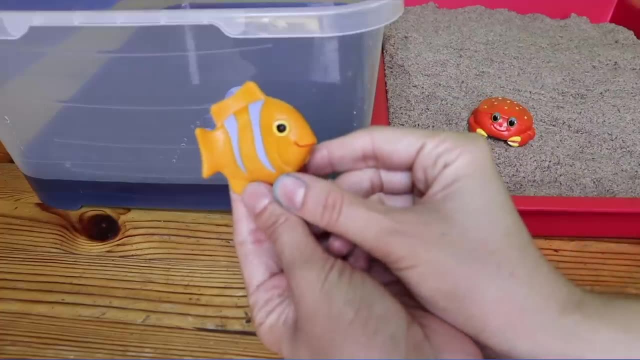 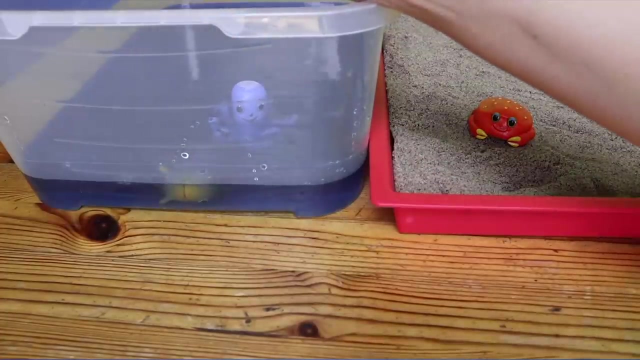 to the farm. you belong on the farm, mister horse. oh, thank you bye-bye. say bye-bye" my horse say bye-bye. thank you so much. can you put me in the water? sure, put her in. put her in. put her in the water. okay, put my hardly hands by. 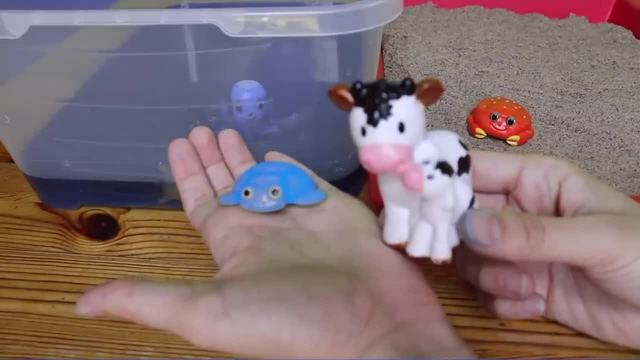 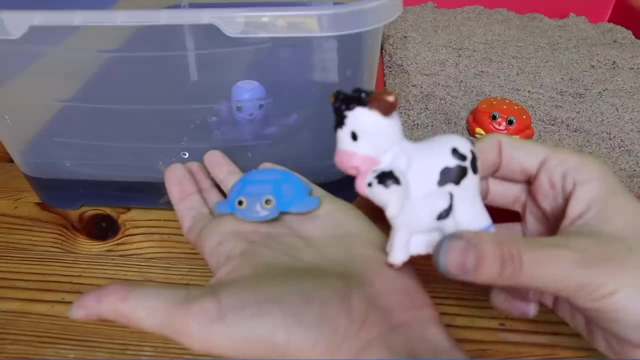 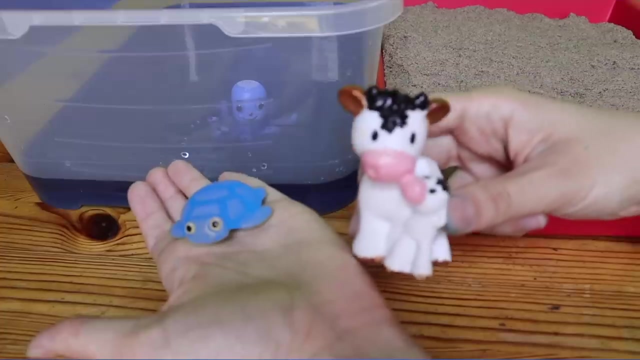 her: I s mess. what are you? you're coming, hey, where are you going? where are you going? where are needed? wait, that way, the good guy sea turtle, or the cow, Yeah, the sea turtle, The cow, is going to go back to the farm. Moo, Moo, Thank you, Bye-bye. 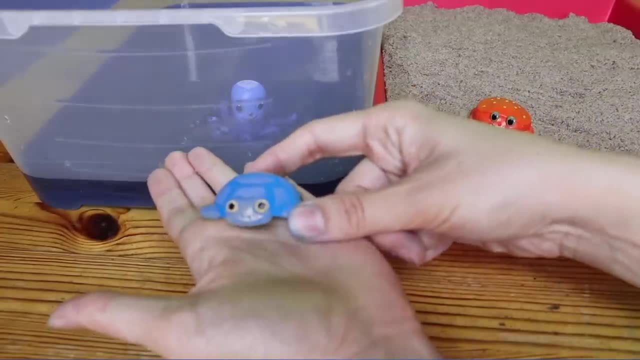 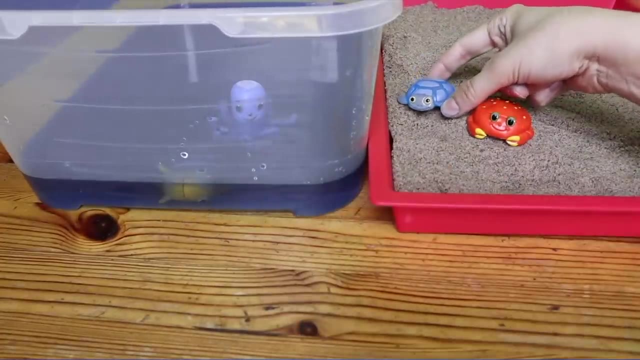 And we'll put the sea turtle in the sand. They also like the water. Thank you so much. I love the sand And put him on, put him on, put him on. Oh, he's already crawling around. This is fun. 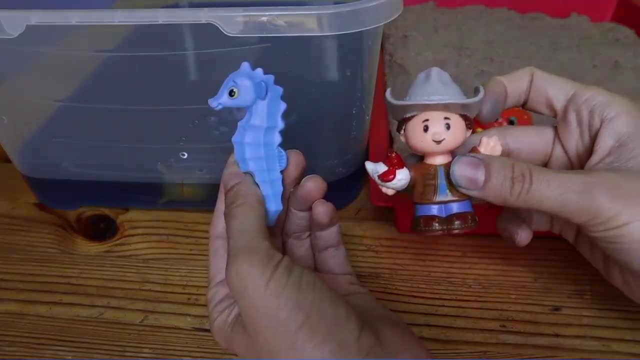 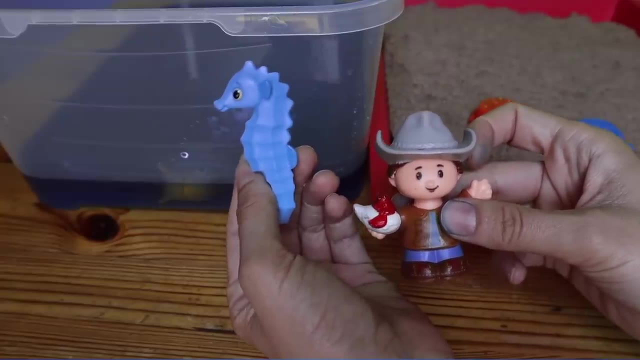 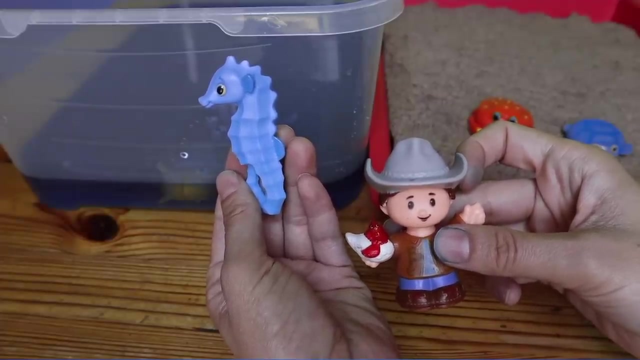 Who should we put in the water, The farmer or the seahorse? This one's kind of tricky, because seahorse has the word horse in its name, But a seahorse actually belongs in the water or the ocean It swims. 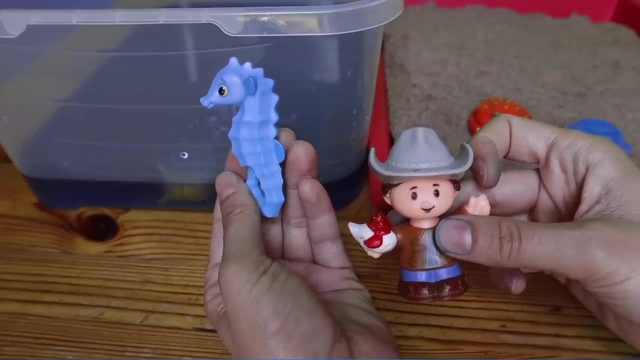 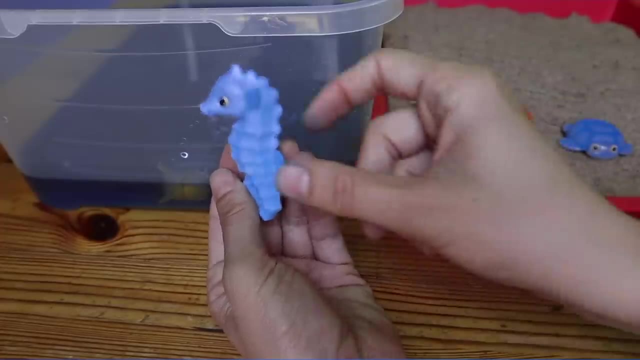 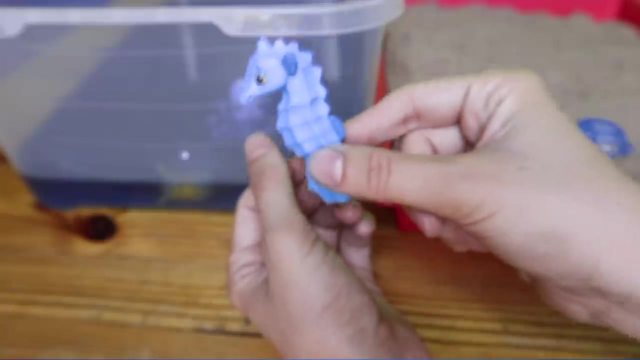 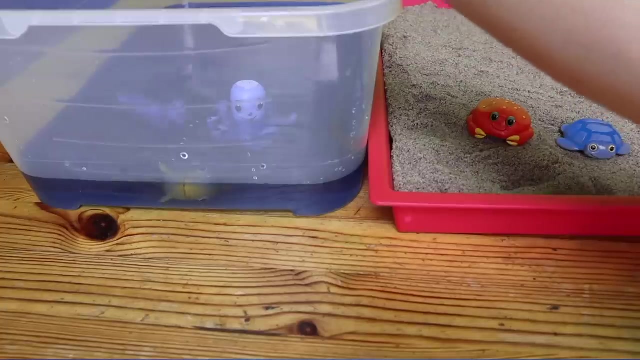 And the farmer belongs on the farm. Okay, I'm going back to the farm. Bye-bye, Good job. Thank you so much. You helped me find my home, which is in the water on the beach. Put her in. put her in. put her, Say in and she'll dive in In. Yay, Here's our last one. 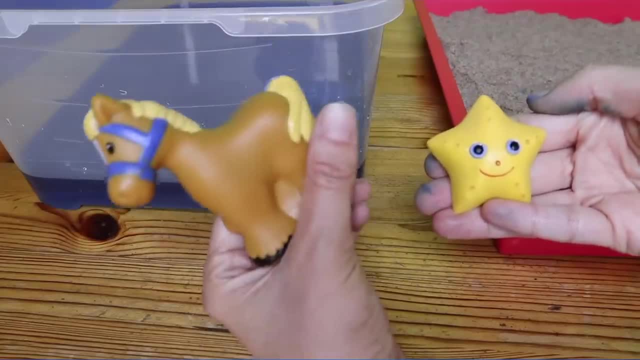 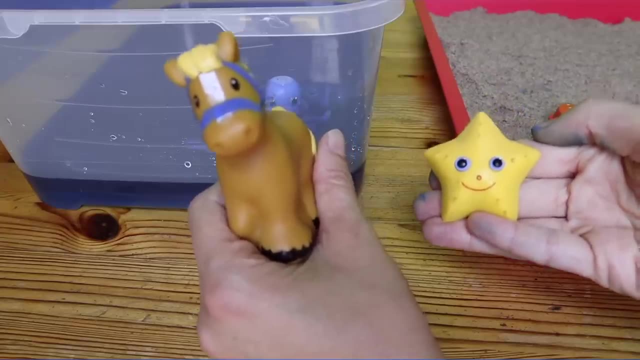 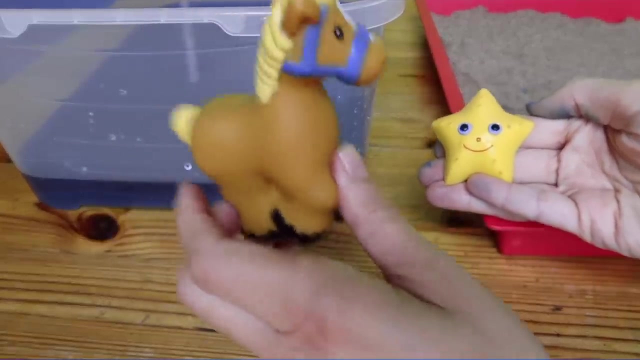 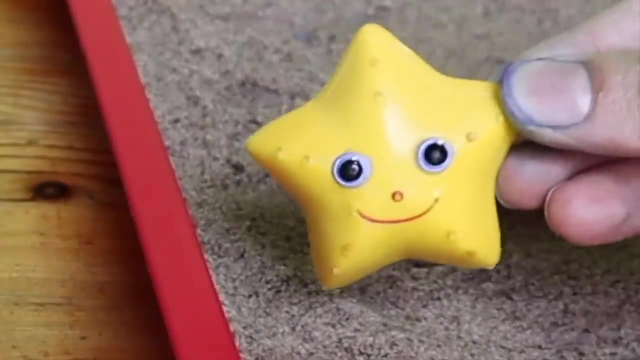 Who belongs on the seashore, On the sand or in the ocean, The horse, Nay Or the starfish? Hello, The starfish. The horse lives on the farm Nay. Oh, bye, Let's put the starfish in the sand. Thank you so much. I love the sand. 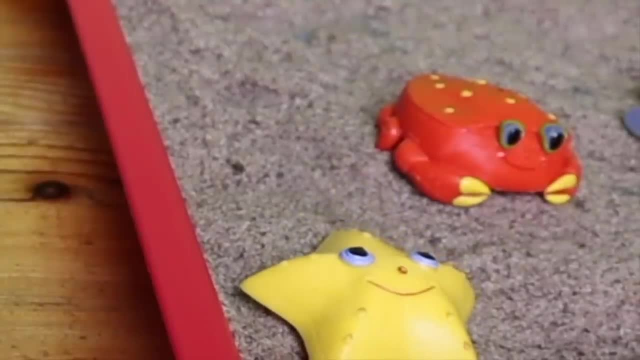 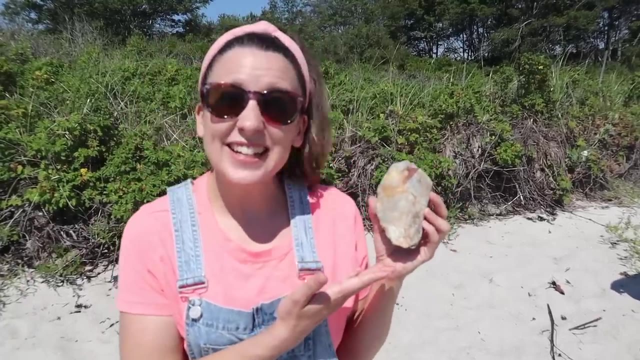 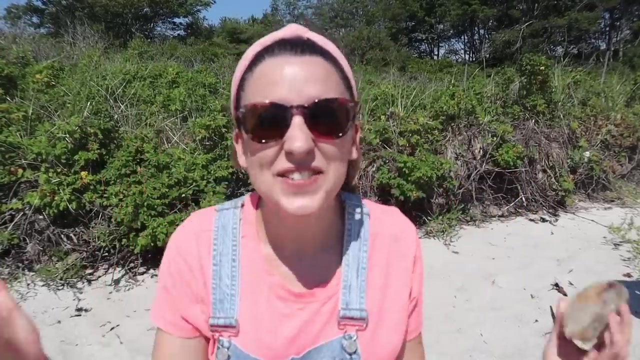 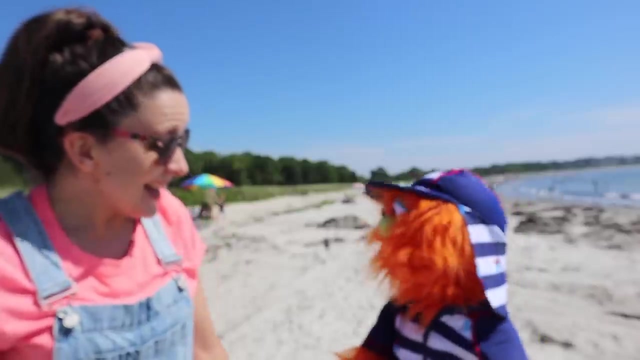 Ah, I love that. It's so nice. Oh, what fun. My sister loves the sand the most. Wow, I found a really shiny rock. Have you ever looked for rocks and shells at the beach? It's so much fun. 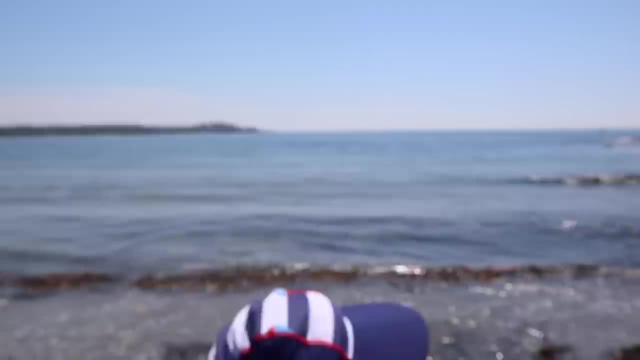 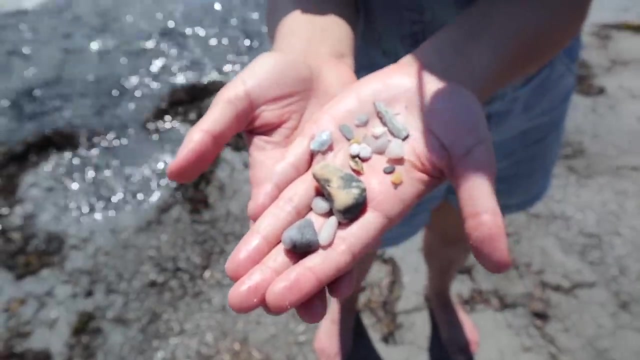 It's like hunting for treasure- Must make a look what I found. Wow, Herbie found a seashell. Awesome, Herbie, Let's play with it. Wow, I found some really cool little pebbles and rocks on the beach. 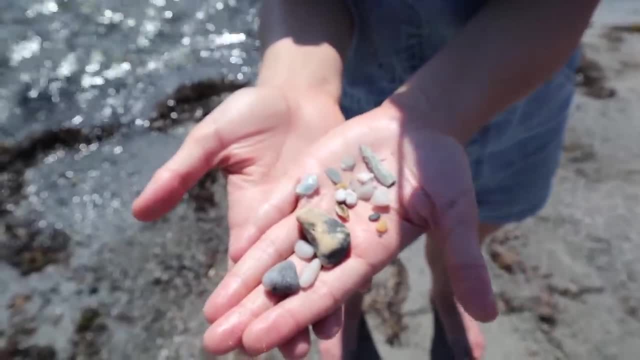 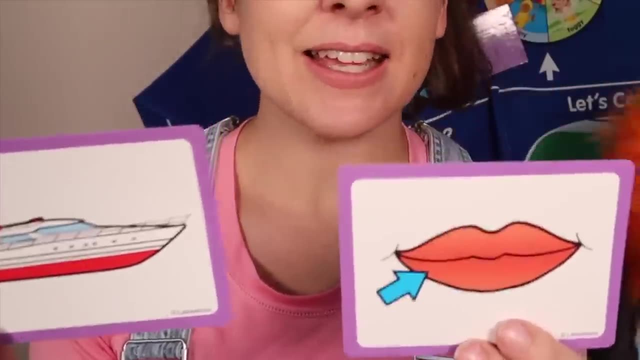 It's like treasure. Yeah, it was so fun searching for them. Next it's time for our rhyme of the day. Rhymes are words that sound the same at the end. Yeah, Lip and ship, Do those sound the same at the end? 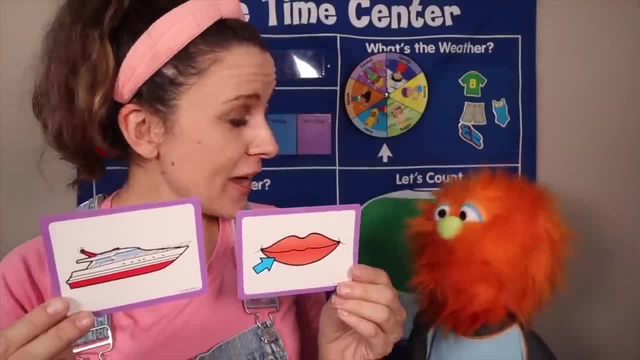 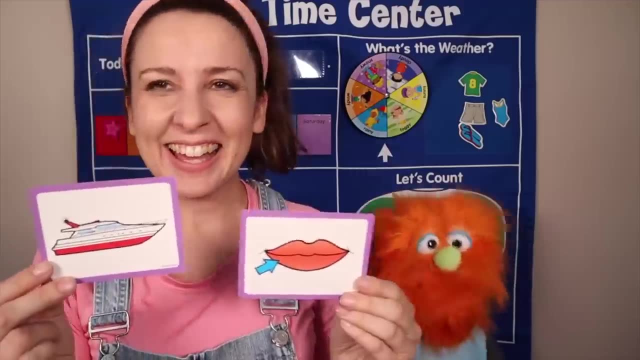 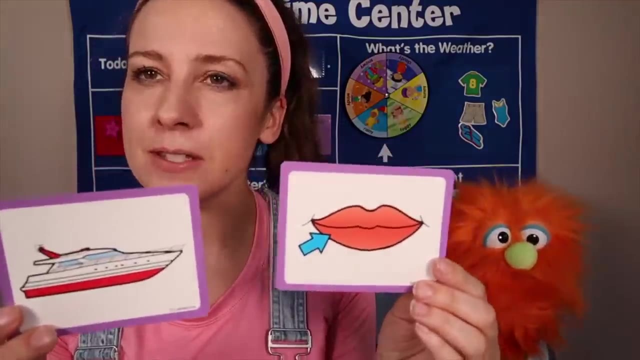 Yeah, they do. Yeah, You know what else rhymes What? Herbie and burbie. That's so silly. Except burbie's not really a word, That's so funny. And Rachel and Wachel Wachel. Okay, do you know where your lip is? 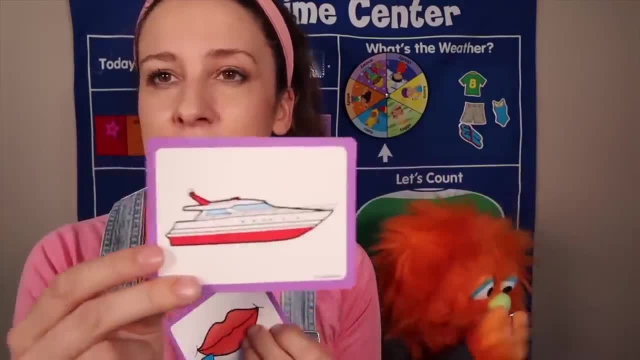 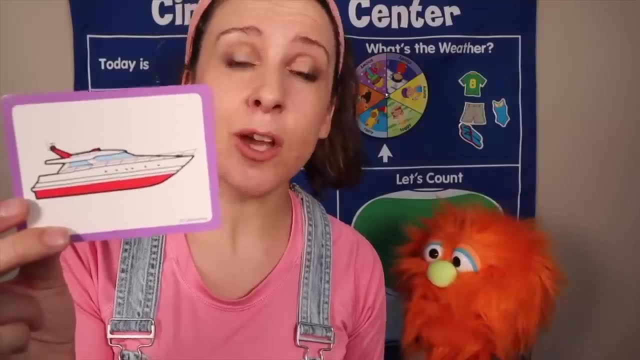 We have two lips, Lip, And then there's ship. A ship is really really, really big. It's bigger than a boat. Whoa Yeah, Ships go in the ocean. Now let's pretend we're on a big ship. 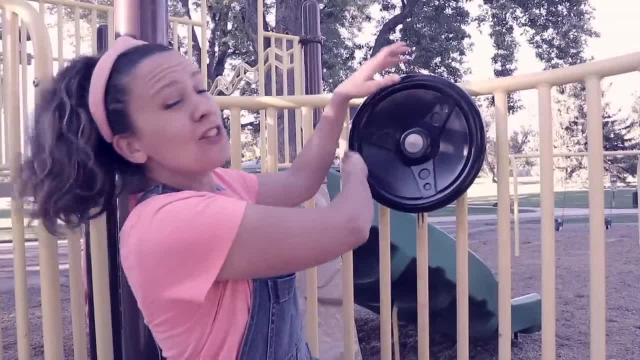 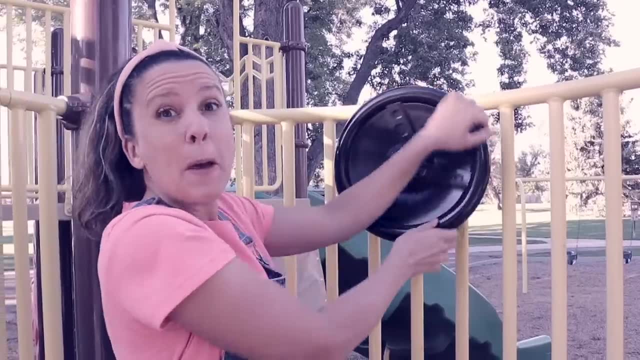 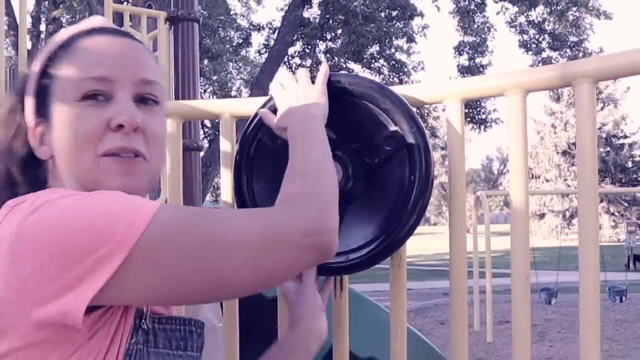 That's a big ship. We're on a big boat and we have to turn the ship and we have to turn the other way. We're on a big ship. Wow, This is the way we steer the ship. Steer the ship. 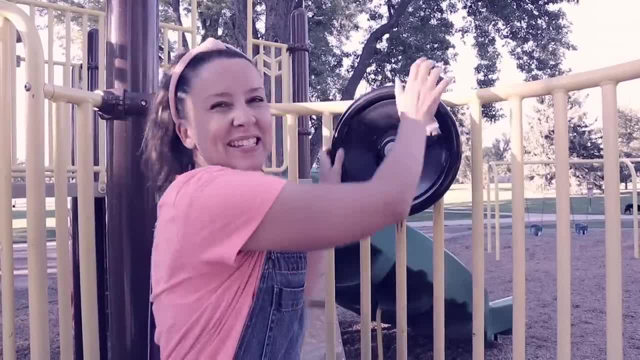 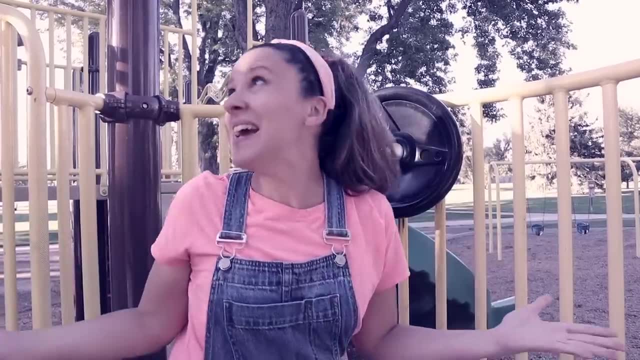 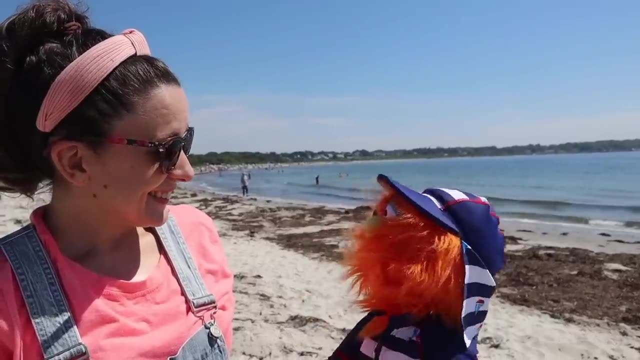 Steer the ship. This is the way we steer the ship. We're steering a big ship, So big. Yay, I'm so excited. I'm going to go play in the water now. Wait, Herbie, You need an adult to go with you. 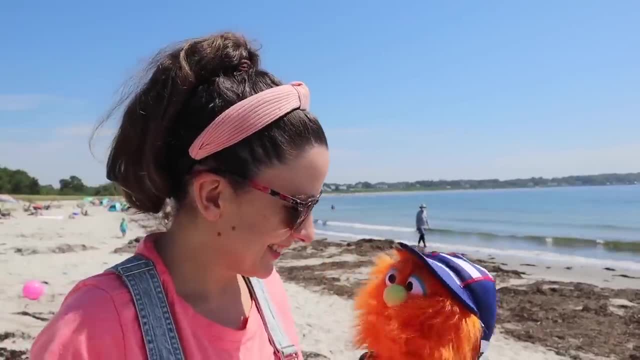 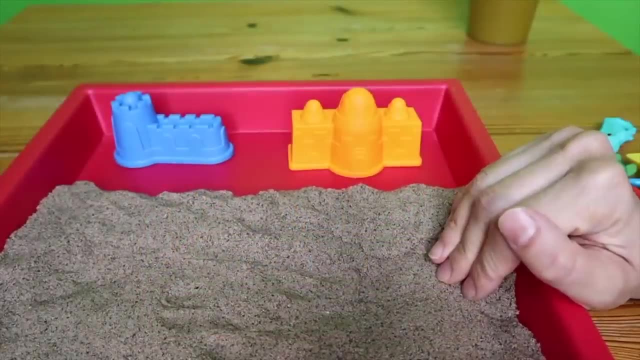 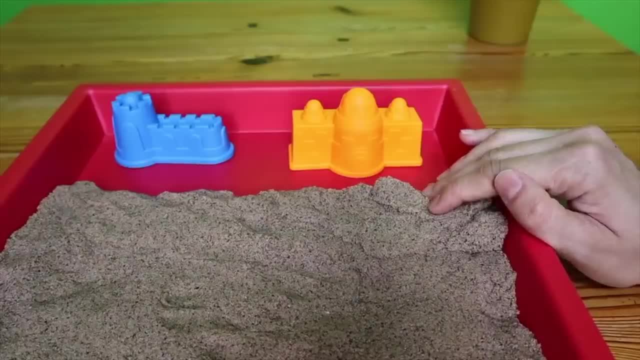 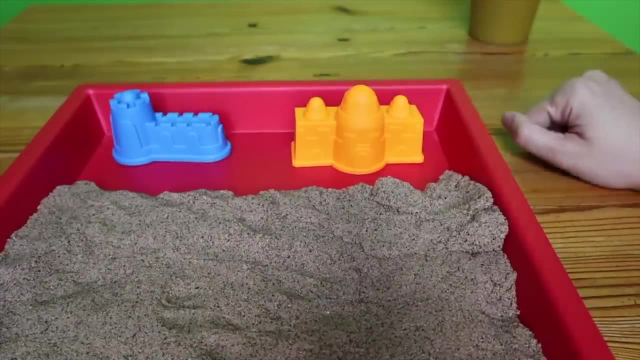 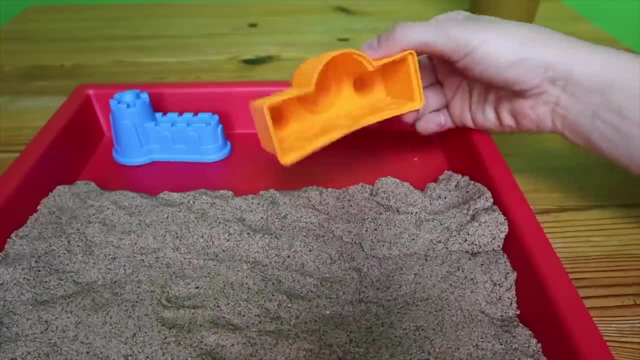 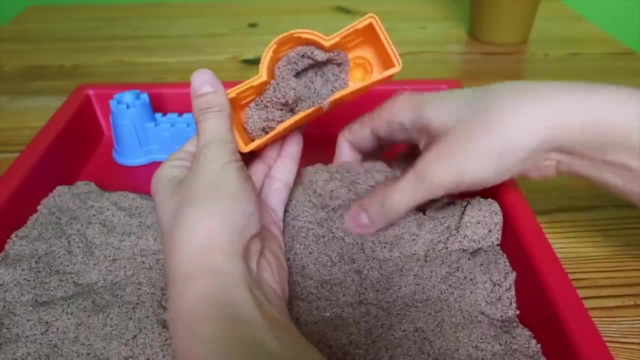 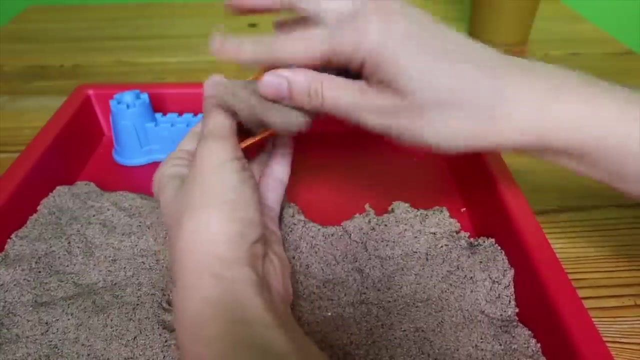 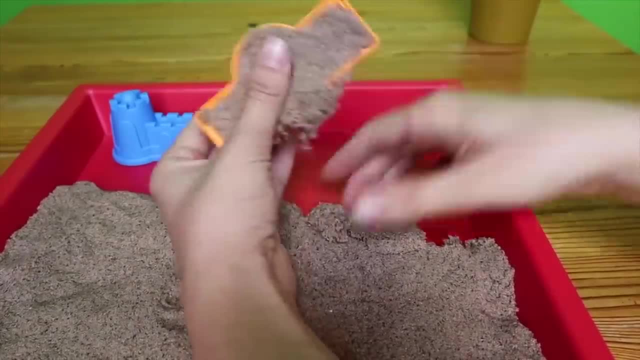 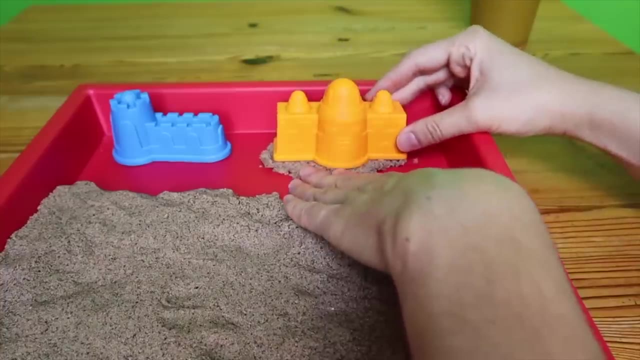 Put it in. Good job, Thank you for helping. Now I'm going to say: ready, set. and then you say: go the magic word and we'll see if it made a sand castle. Are you ready? Yay? 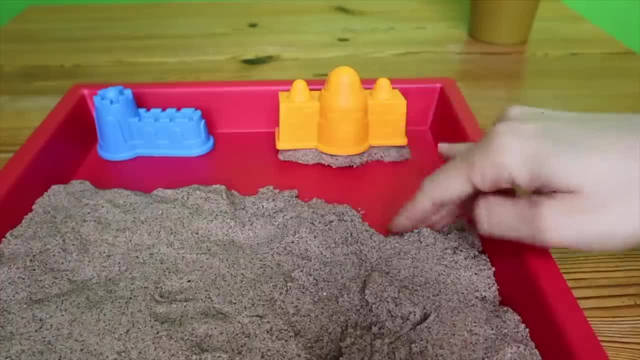 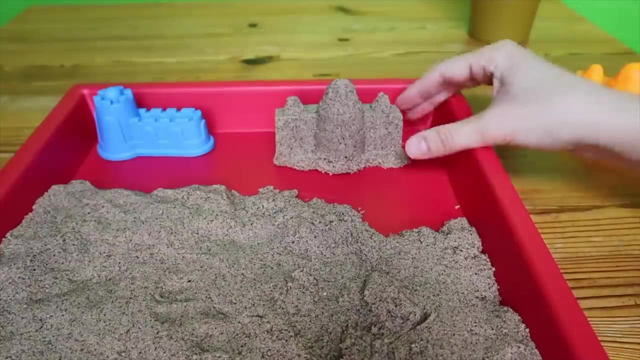 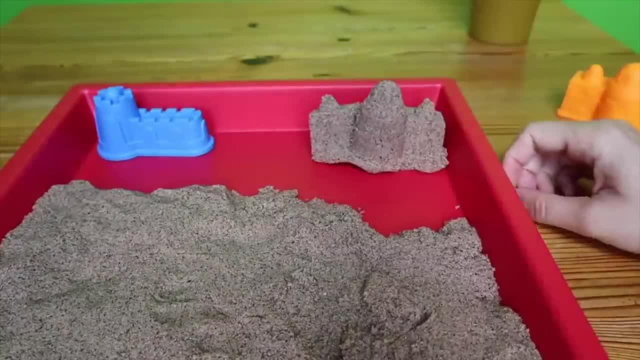 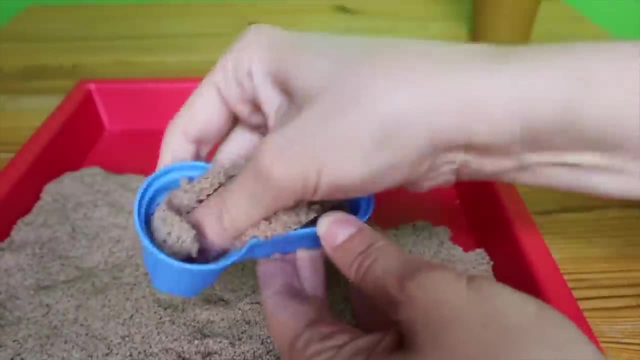 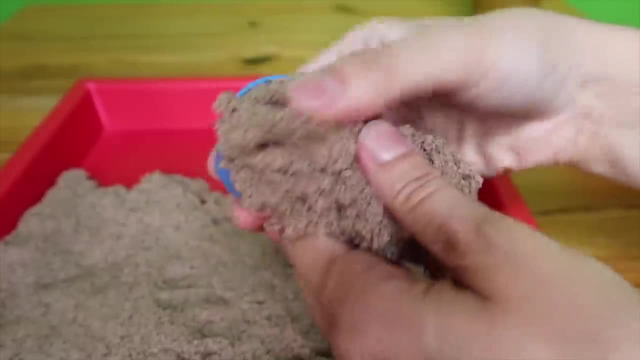 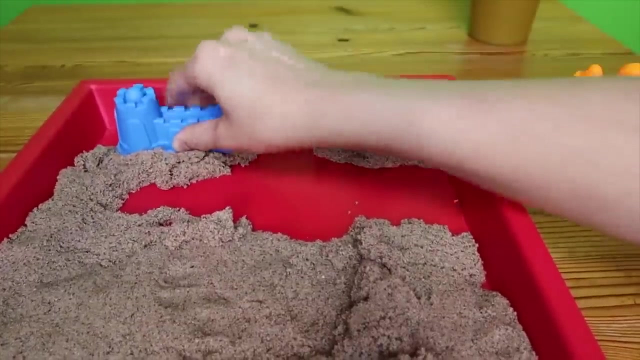 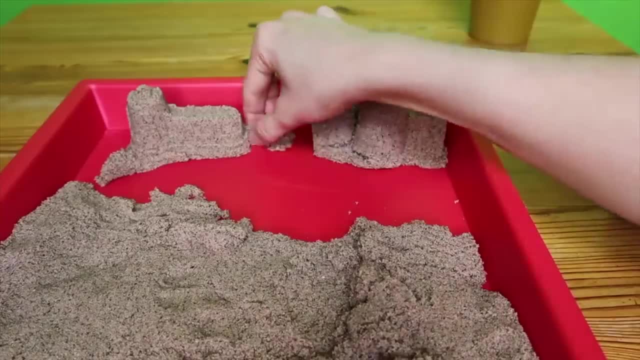 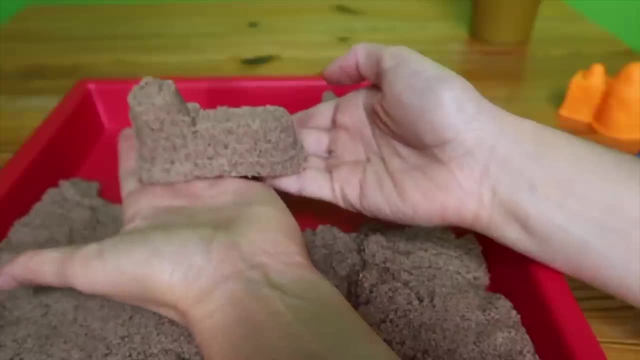 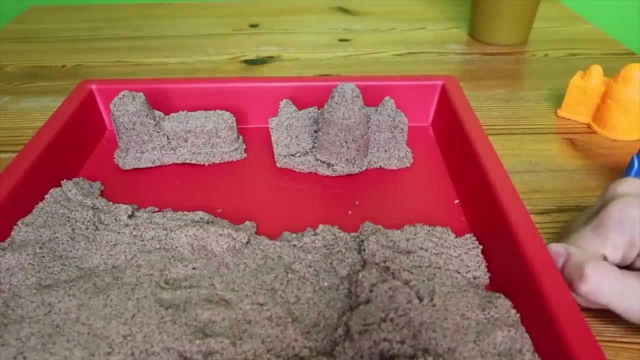 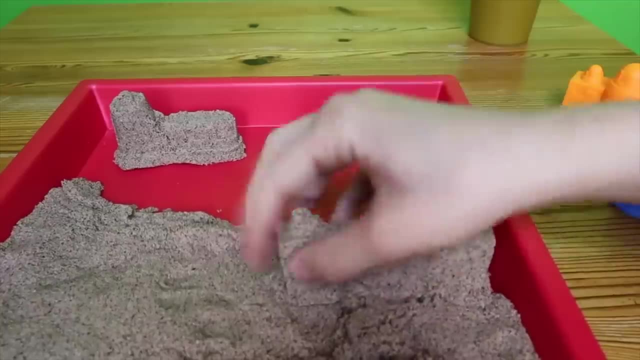 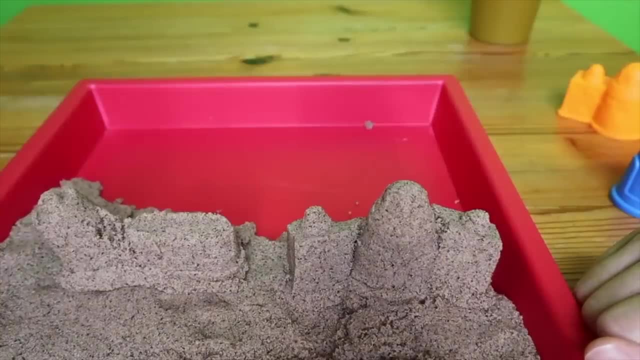 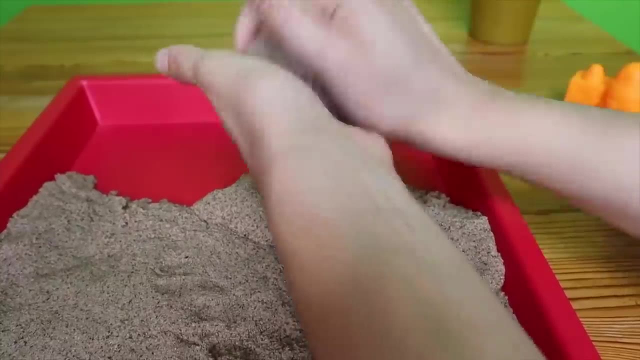 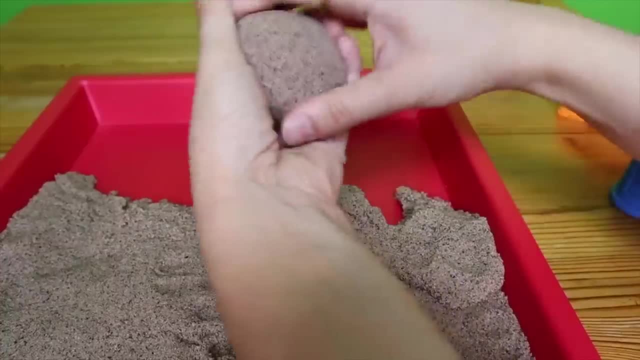 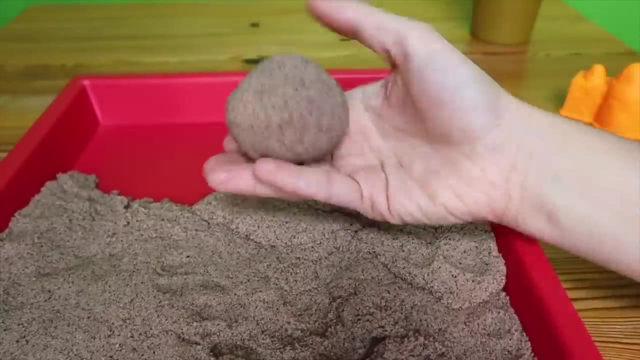 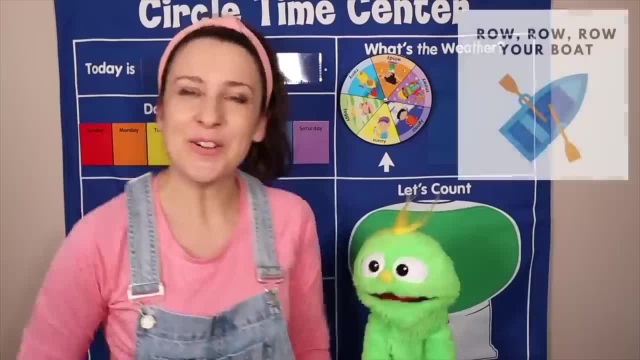 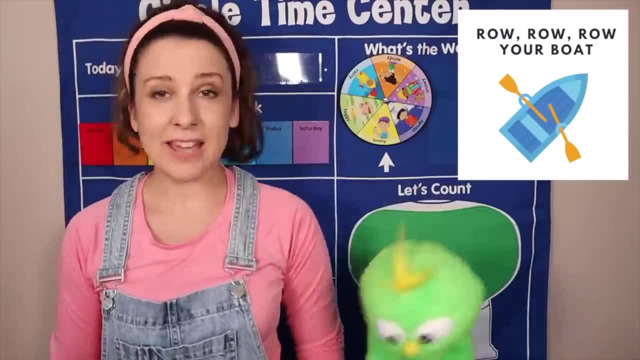 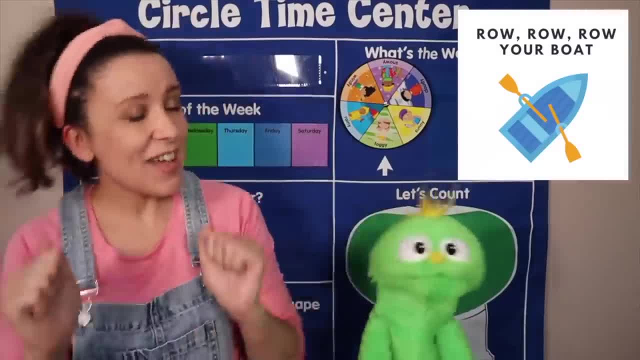 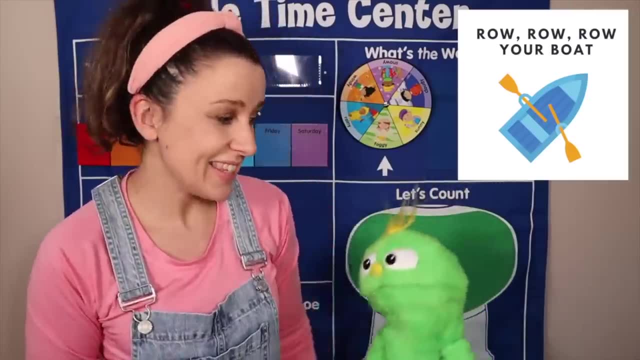 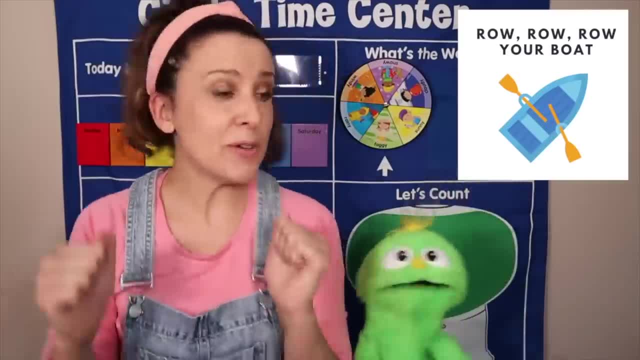 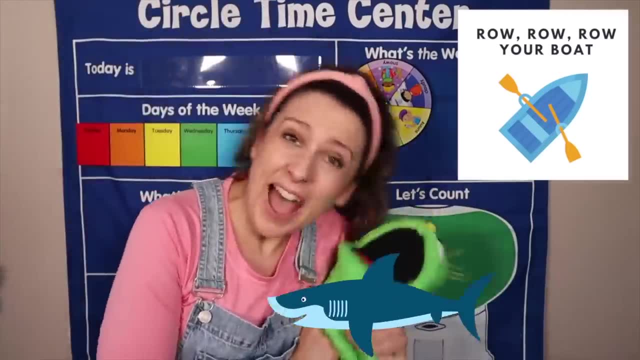 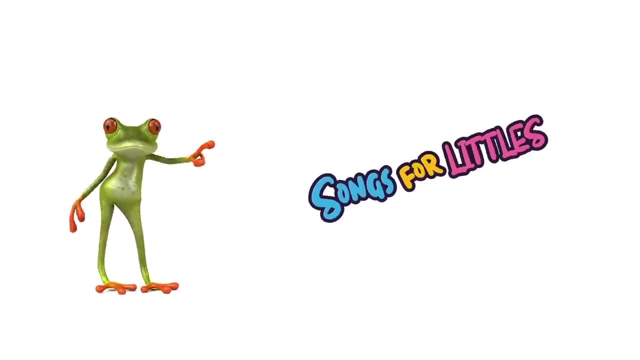 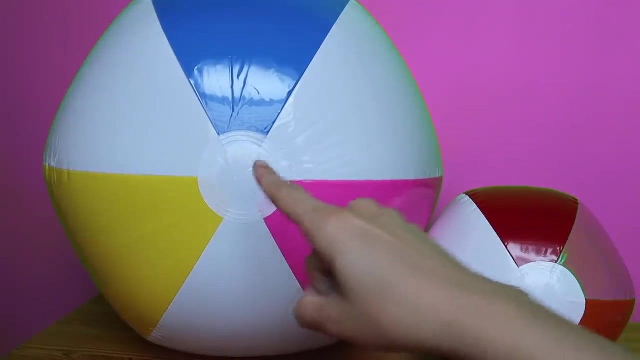 Yay, Yay, Yay, Yay, Yay, Yay. If you see a great white shark, don't forget to scream: ahhhhhh, How many beach balls do we have? Let's count One, two, Two beach balls. 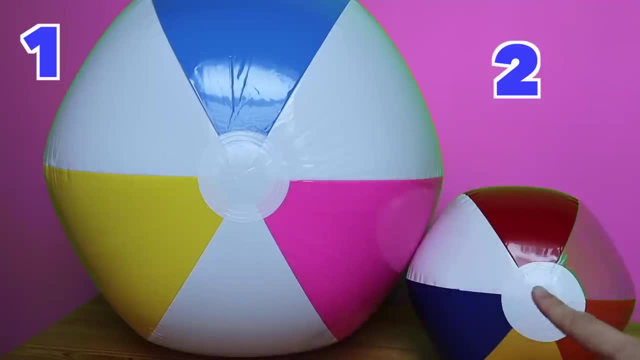 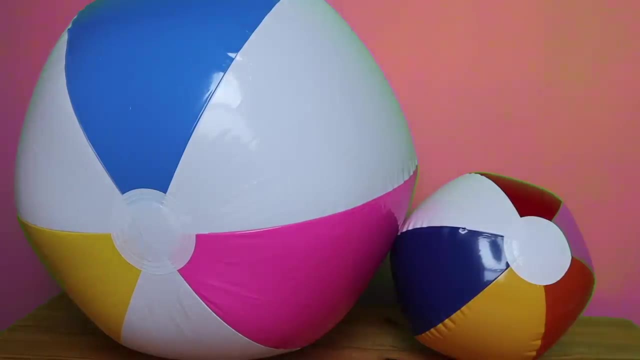 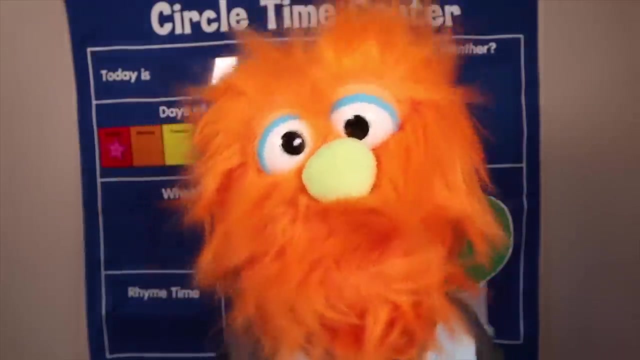 Two beach balls, One, two. One of the beach balls is bigger. Which beach ball is bigger? Yeah, This beach ball is bigger And this beach ball is smaller. Good job. What did the beach say to the shore? Nothing, It just waved. 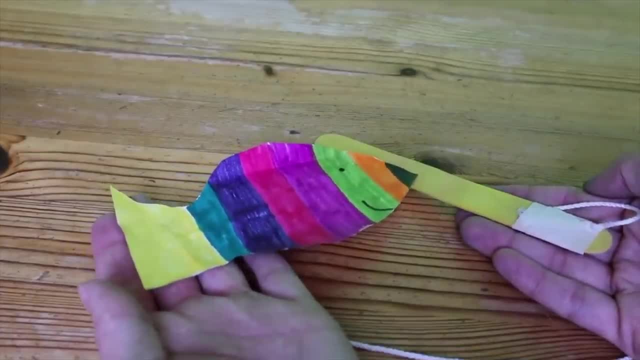 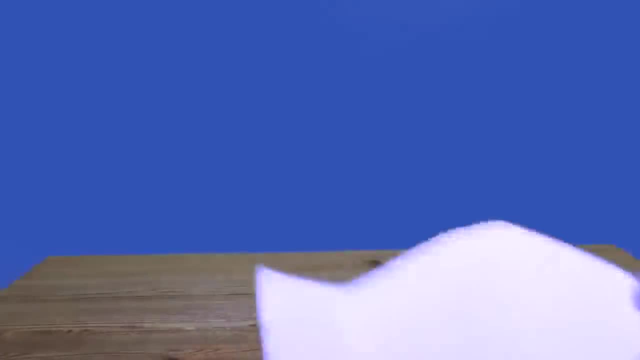 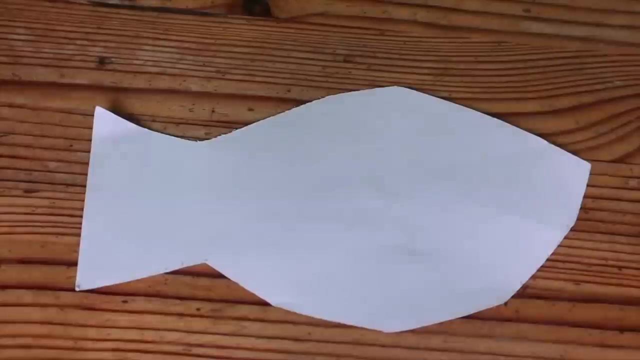 It's time for art. Today we're going to make a fish on a pretend fishing pole. Yeah, The first thing you do is cut a fish out of paper. Have a grown-up help you with the scissors. Now we get to decorate the fish. 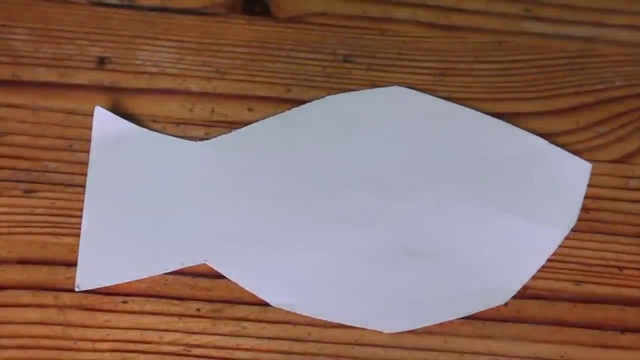 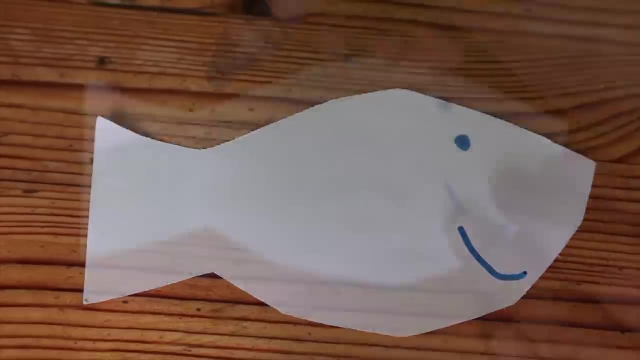 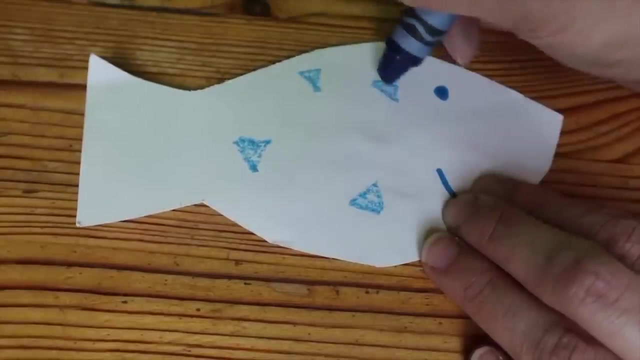 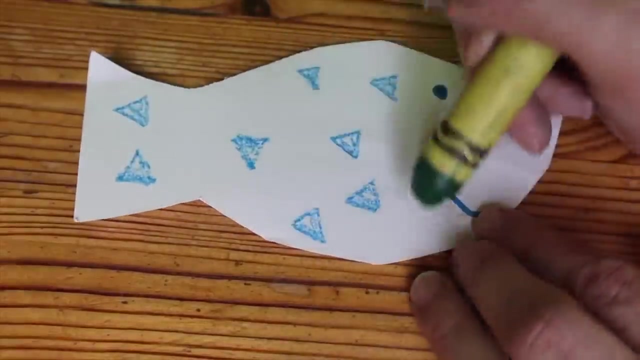 How would you decorate your fish? I like to put a little eye and then a smile: Happy fish. I think I'll color this fish with blue triangles- The shape of the day. So fun, I like decorating the fish. Now I'm going to add some green. 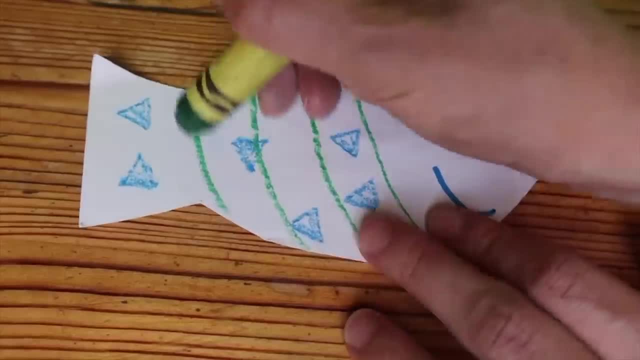 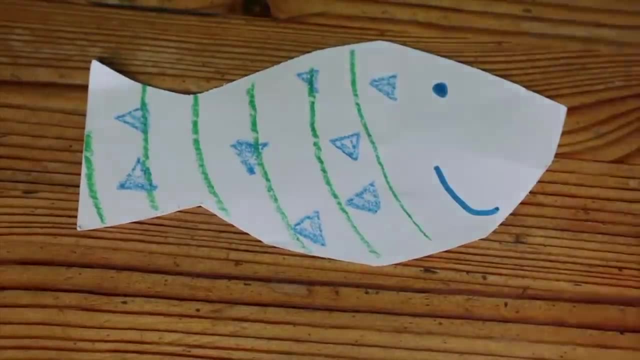 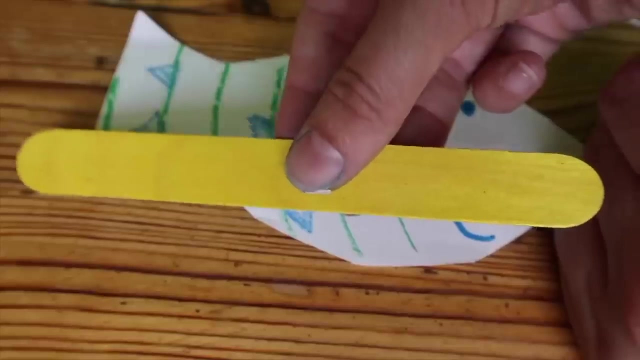 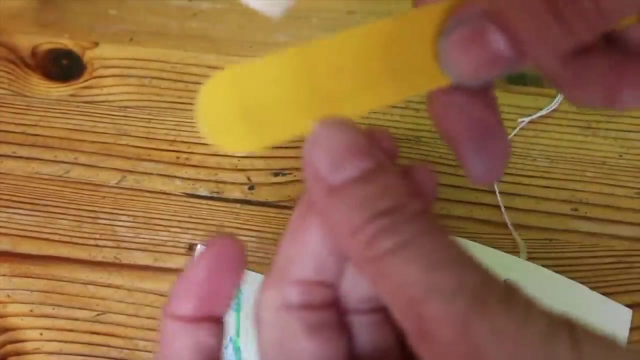 Green stripes. What are you putting on your fish? Next, we take a piece of string and we're going to tape it to a popsicle stick. Get out a piece of tape- This is called masking tape- And I'm going to tape the string. 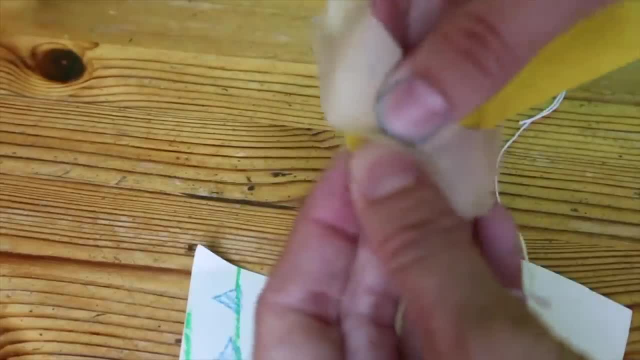 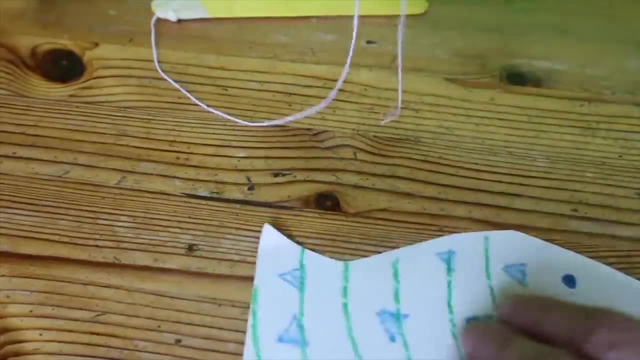 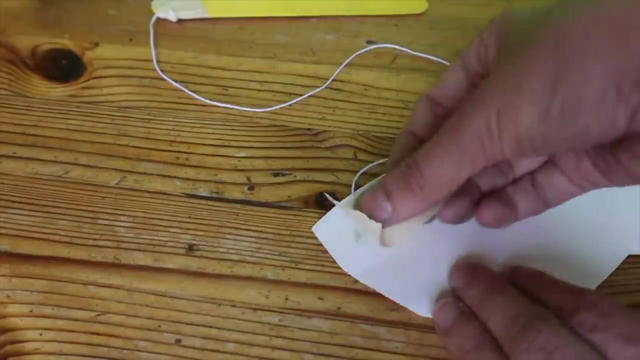 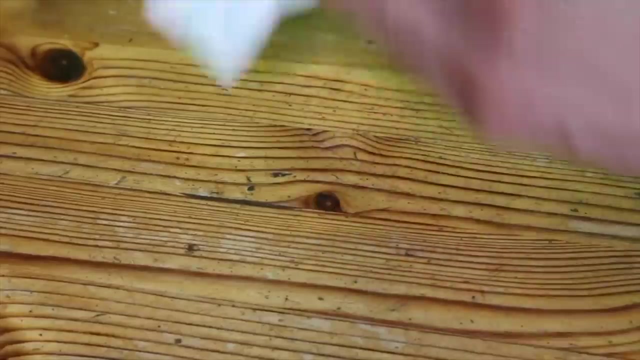 to the popsicle stick. Tape it, Tape it on. Now I'm going to put some tape on this side and tape the fish. Okay, let's put some tape on the fish. Yay, We put it on. And now the fish is on a fishing pole. 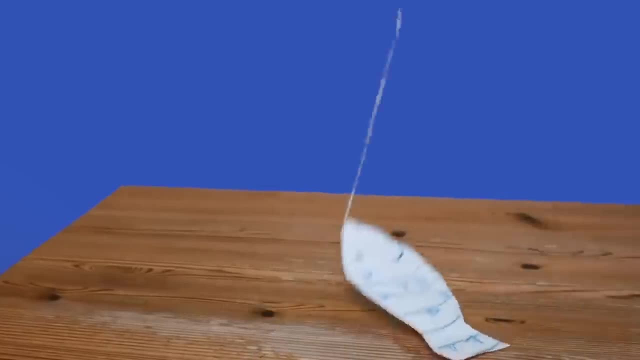 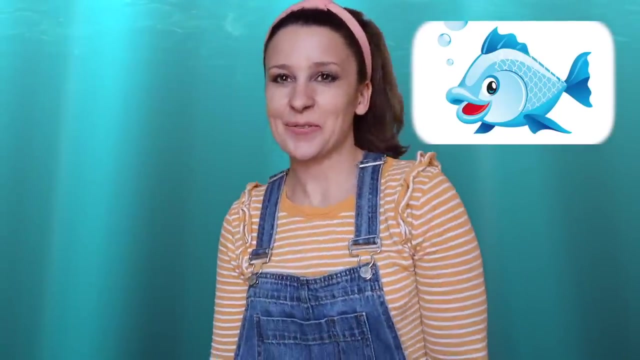 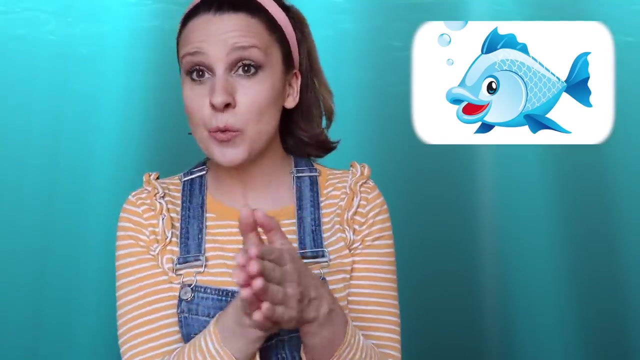 We did it. We made a fishing pole and a fish. Let's get out one little blue fish. Are you ready? One little blue fish swimming in the water. One little blue fish swimming in the water. One little blue fish swimming in the water. 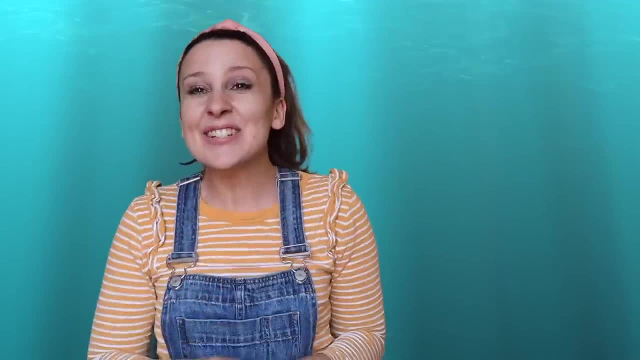 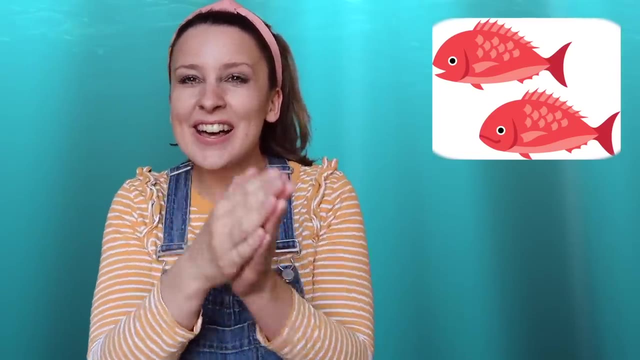 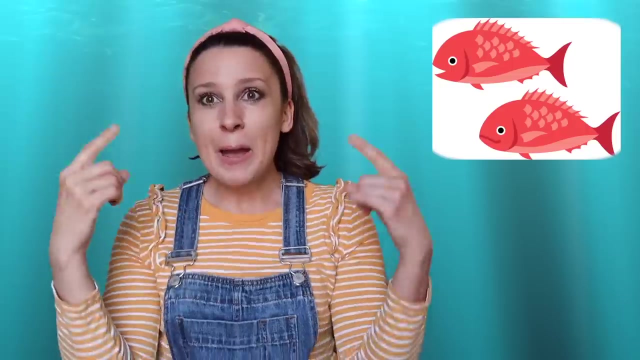 Bubble, bubble, bubble, bubble pop. That was fun. Let's get out two little red fish. Two little red fish swimming in the water. Two little red fish swimming in the water. Two little red fish swimming in the water. Bubble, bubble, bubble, bubble pop. 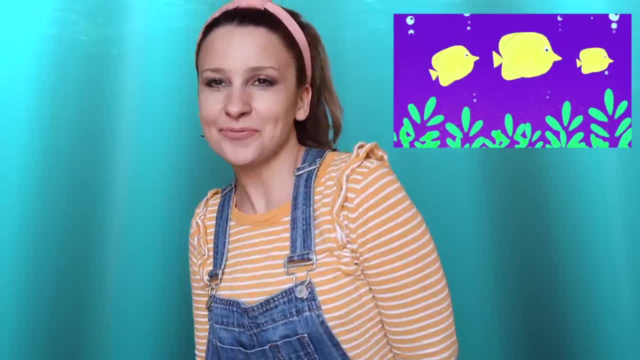 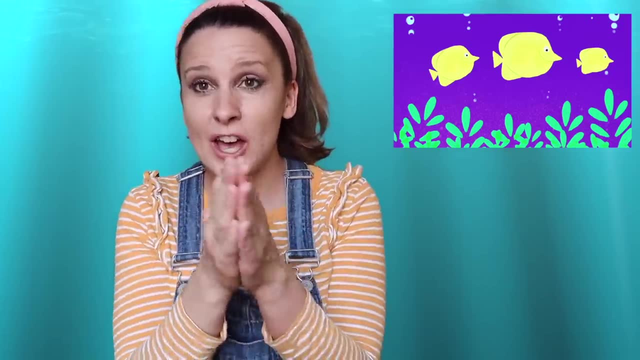 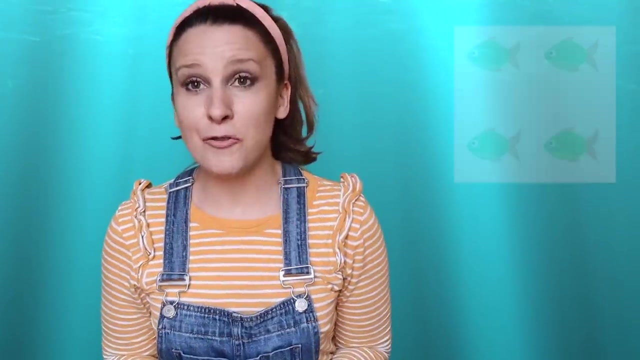 Wow, Let's get three yellow fish. Three little yellow fish swimming in the water. Three little yellow fish swimming in the water. Three little yellow fish swimming in the water, Bubble, bubble, bubble, bubble pop. How about four green fish? 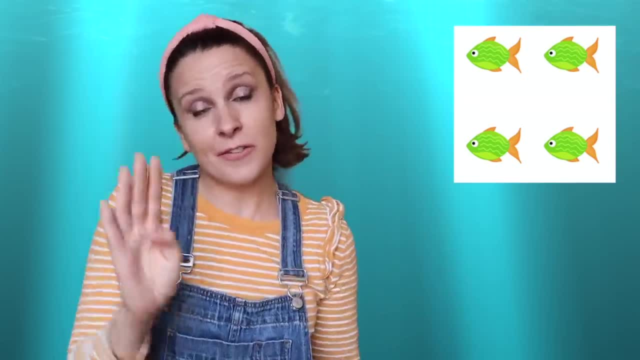 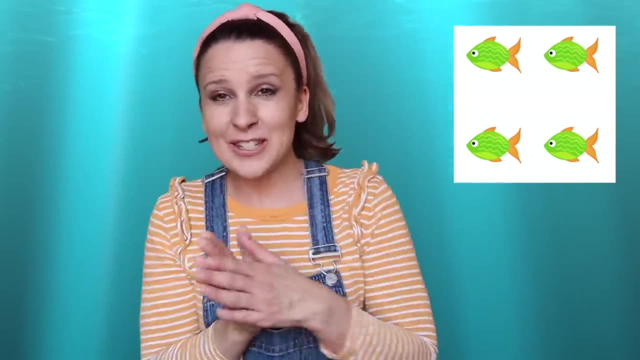 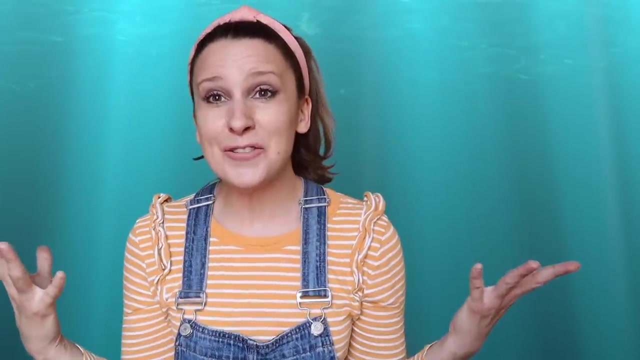 I'm excited. Four little green fish swimming in the water. Four little green fish swimming in the water. Four little green fish swimming in the water, Bubble, bubble, bubble, bubble pop. Now let's do five rainbow fish. Five little rainbow fish swimming in the water. 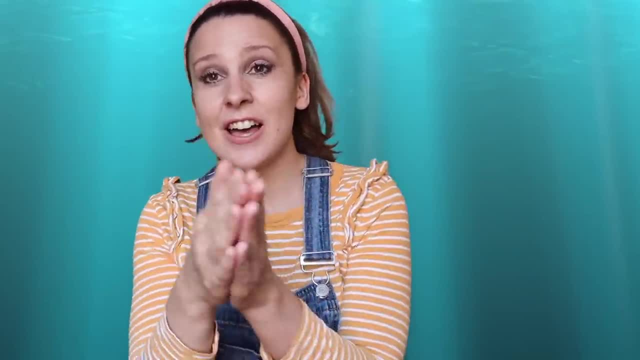 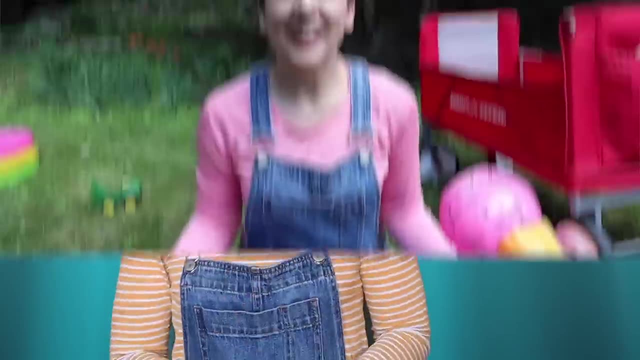 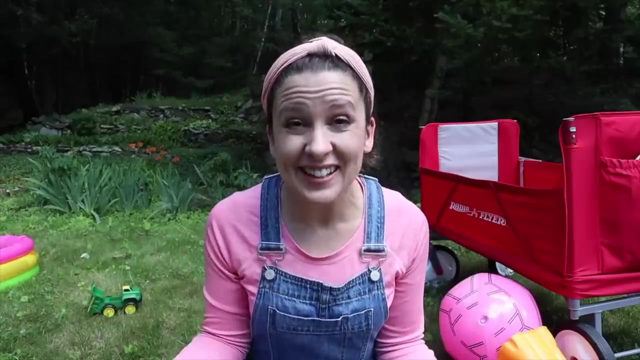 Five little rainbow fish swimming in the water. Five little rainbow fish swimming in the water: Bubble, bubble, bubble, bubble pop. Let's go see my friends Teresa and Rowan. They're going to help us count some seashells. 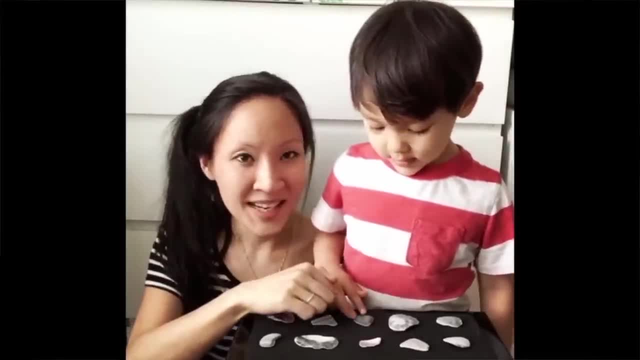 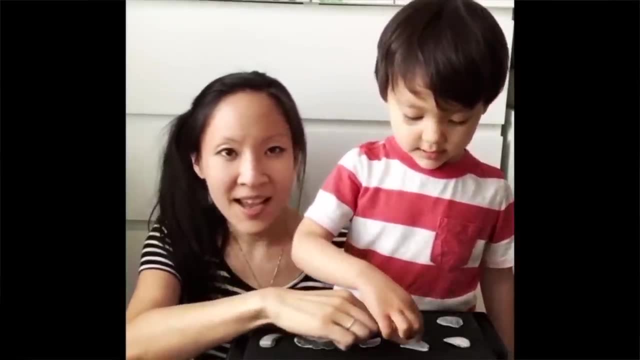 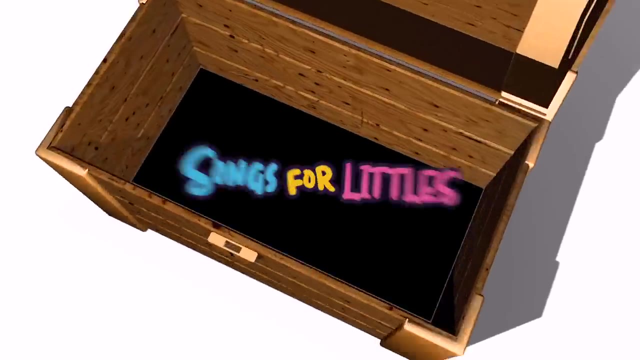 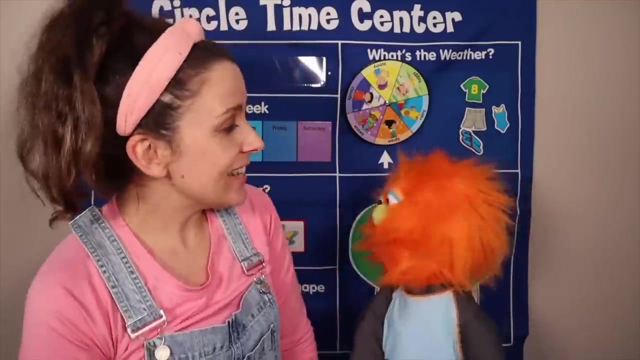 One, two, three seashells, Four, five, six seashells, Seven, eight, nine seashells. Now we count to ten. Our next call and echo song is a really fun game. Oh great, Yeah, it's like duck duck goose. 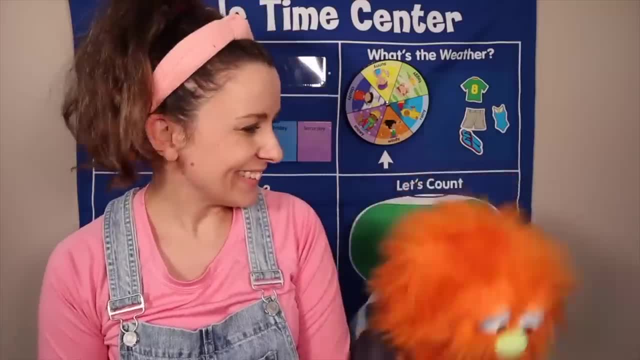 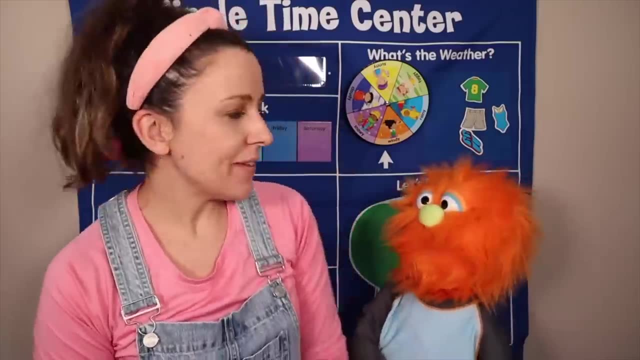 Oh, I love duck duck goose, Duck duck goose, Uh-huh. And then we run. Yeah, you're going to run after me, Oh, okay, Okay. so repeat after me. You repeat after me too, okay. 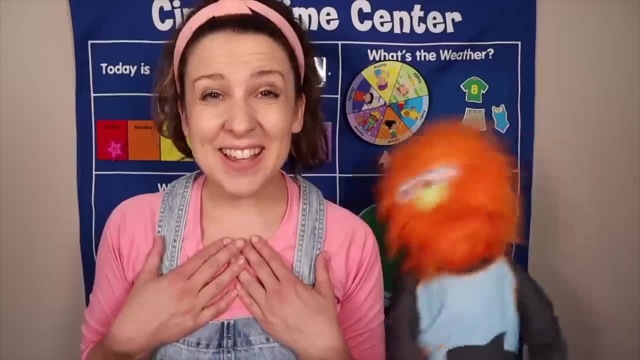 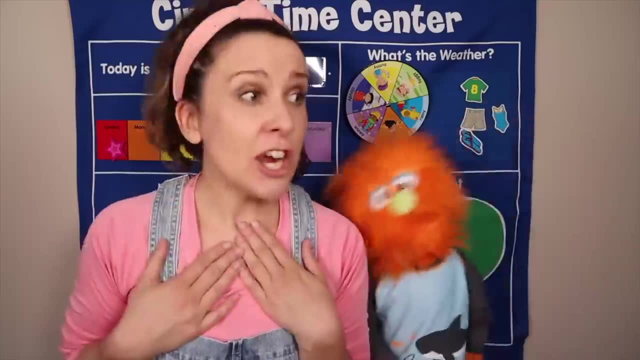 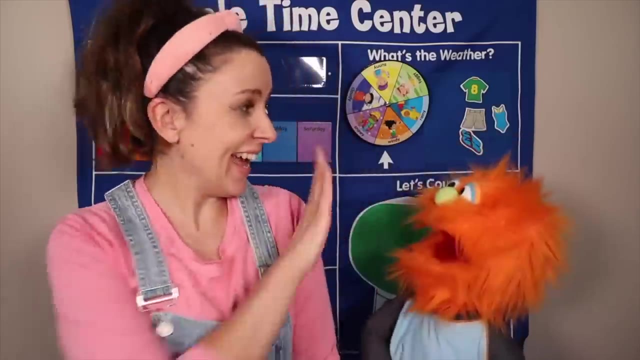 Okay, Charlie over the ocean, Charlie over the ocean, Charlie over the sea, Charlie over the sea. Charlie caught a big fish. Charlie caught a big fish. Can't catch me, Can't catch me. Tag. Now it's your turn and Herbie's turn. 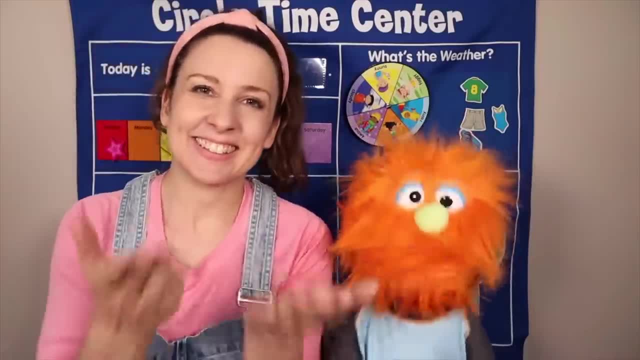 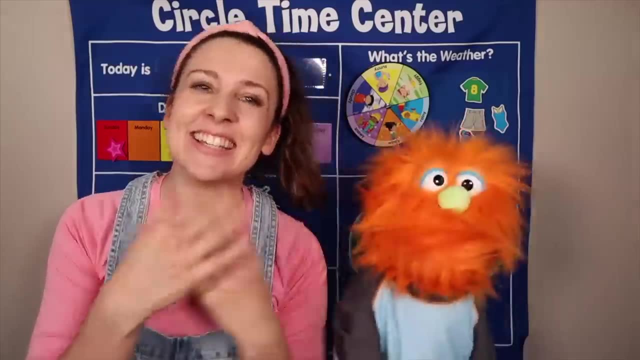 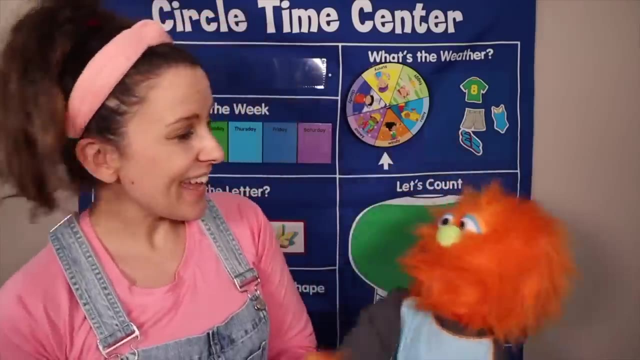 Okay, I'll try. Okay, Charlie over the ocean. Charlie over the ocean. Charlie over the sea. Charlie over the sea. Charlie caught a big fish. Charlie caught a big fish. Charlie can't catch me. Good job, can't catch me. 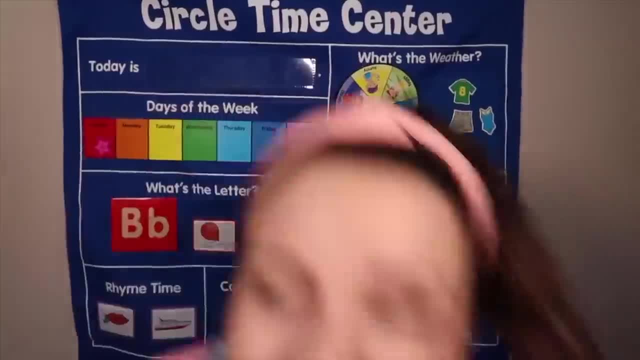 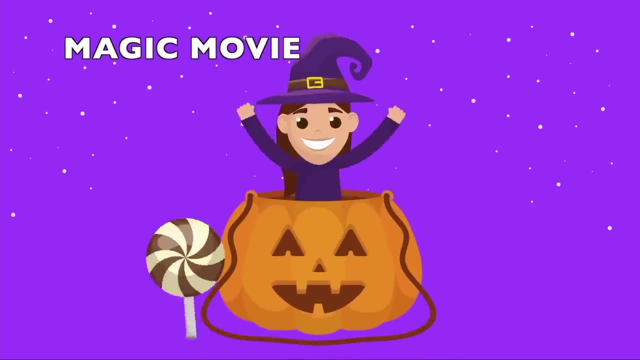 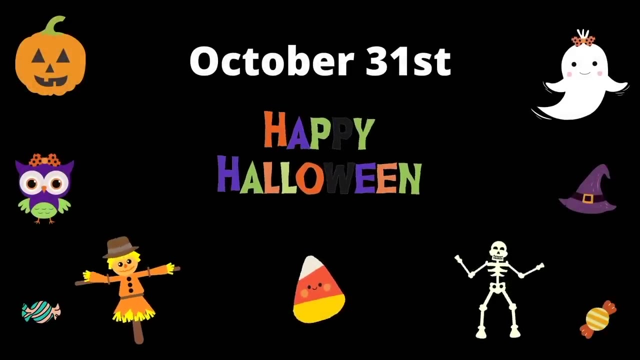 Tag, I couldn't catch you. You were too fast and I couldn't catch Herbie. Time for a magic movie. Let's learn about Halloween. Halloween is a fun holiday. It's celebrated every year on October 1st. Halloween is a fun holiday. 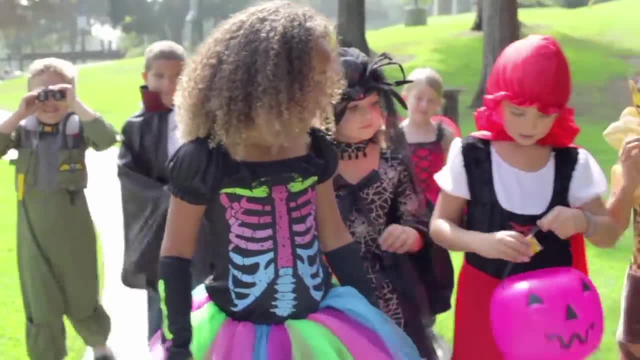 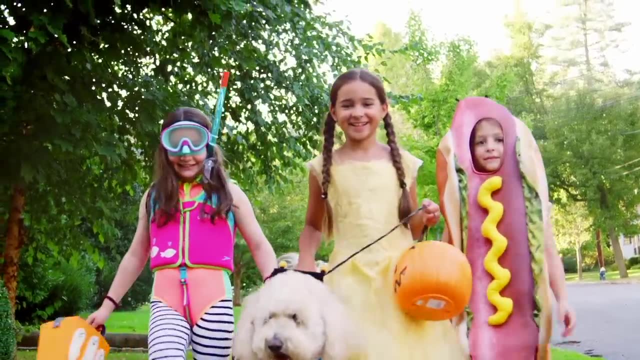 It's celebrated every year on October 31st. On Halloween, we can dress in fun costumes. On Halloween, we can dress in fun costumes. I see a hot dog, a princess and a swimmer. I see a hot dog, a princess and a swimmer. 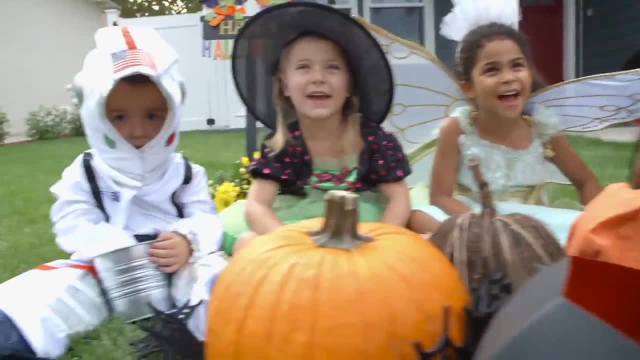 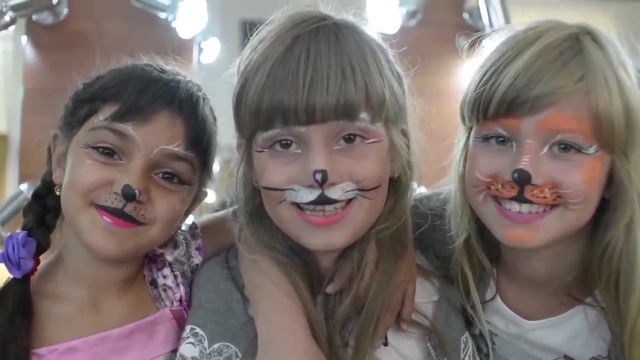 Even the dog is dressed up like a bumble Bee. Even the dog is dressed up like a bumble Bee. Now I see a witch, a fairy, another witch and an astronaut. Some people paint their faces on Halloween with face paint. What's your Halloween costume going to be? 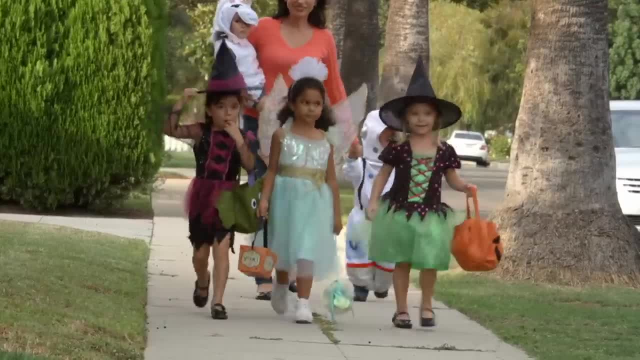 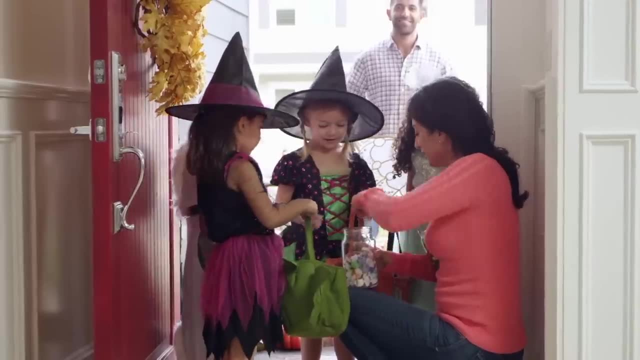 Some years we can go trick-or-treating. First we walk down the street with a grown-up, We knock on the door, knock, knock, knock. Then we say trick-or-treat and we get a treat. Can you say that? 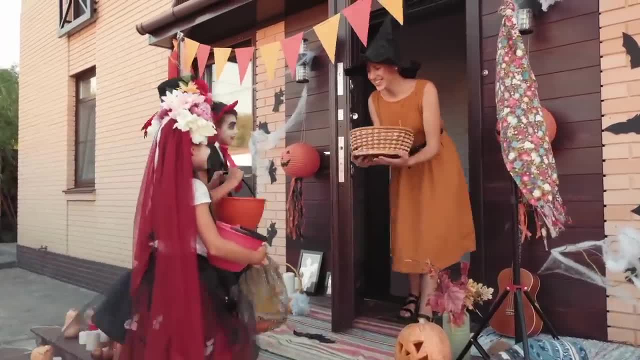 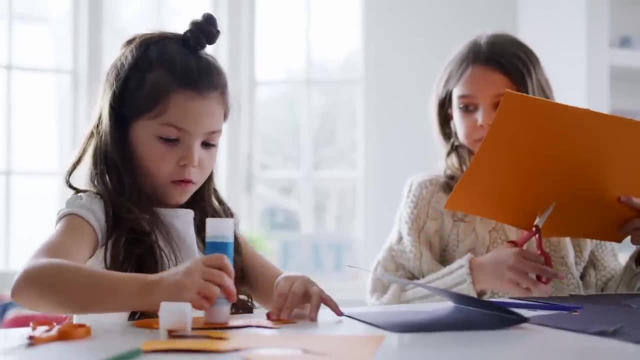 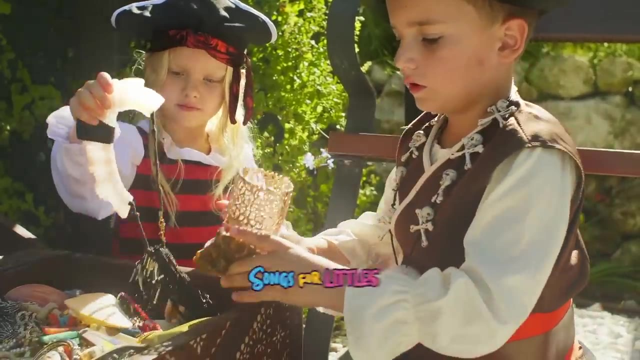 Trick-or-treat. Good job, We can do fun Halloween art projects like painting pumpkins, using glue to paste pumpkins on paper and drawing pumpkins. Halloween is a fun holiday. What should we pack for the beach? Can you think of anything? 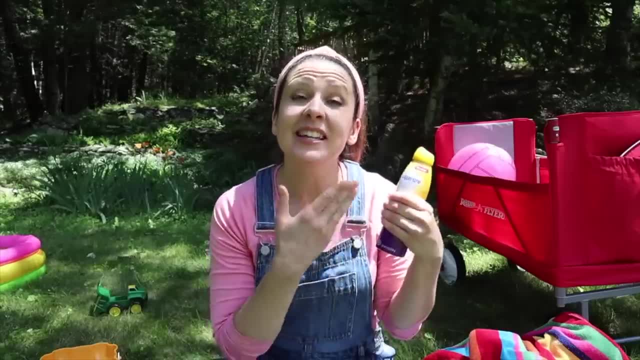 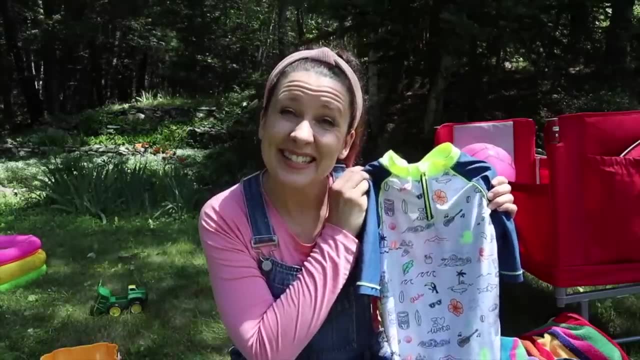 Great ideas. One of the most important things is sunscreen. Yeah, we don't want to get a sunburn. We have to wear lots of sunscreen. Do you know what this is? Yeah, it's a bathing suit. It's good to wear a swim shirt with long sleeves. 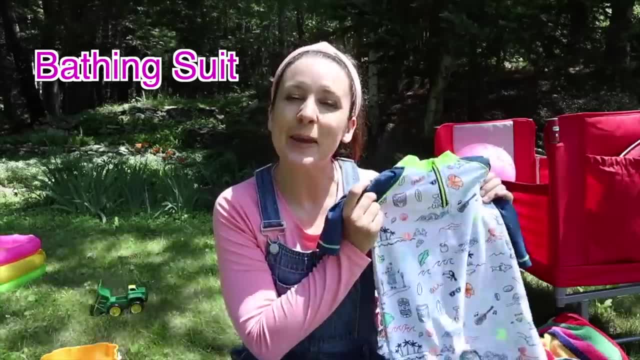 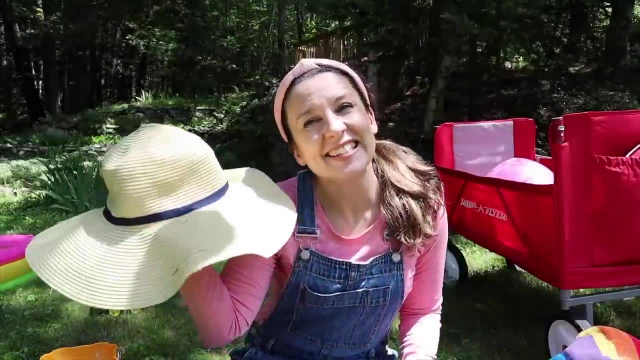 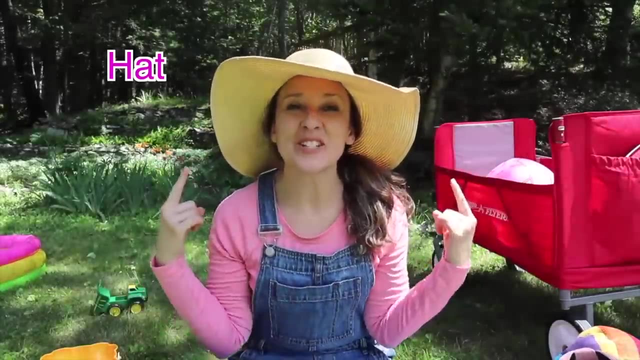 so you don't get burned by the sun. Yeah, this is a little bathing suit. Another great thing to bring to the beach is a what's this? Yeah, it's a hat. Put the hat on. Rachel is wearing the hat. 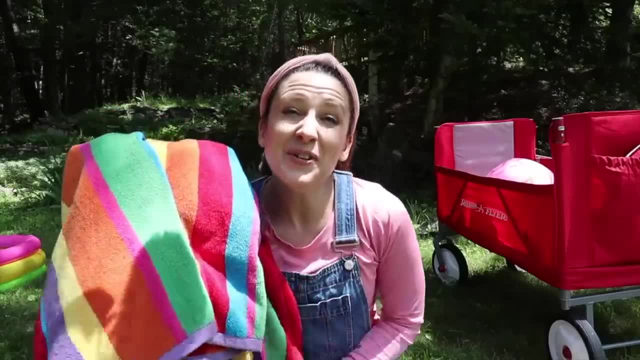 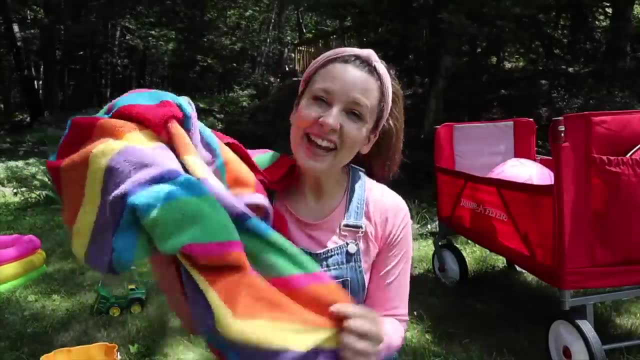 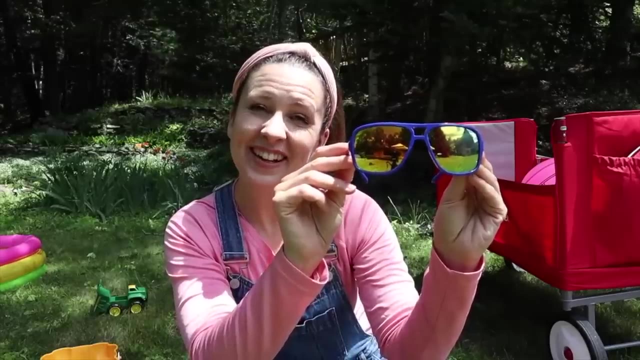 I like wearing my beach hat. Do you know what this is? You might use this when you get out of the bath. Yeah, It's a towel. It's good to bring towels to the beach so you can dry off. Do you know what these are? 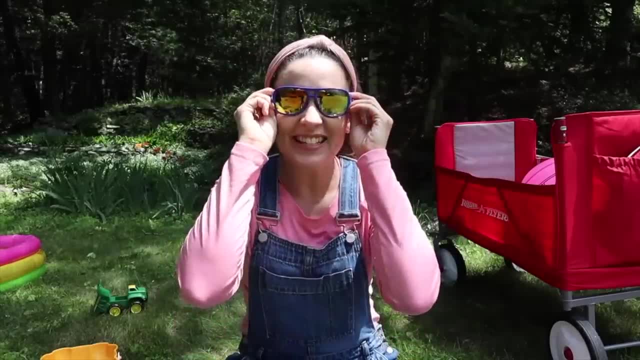 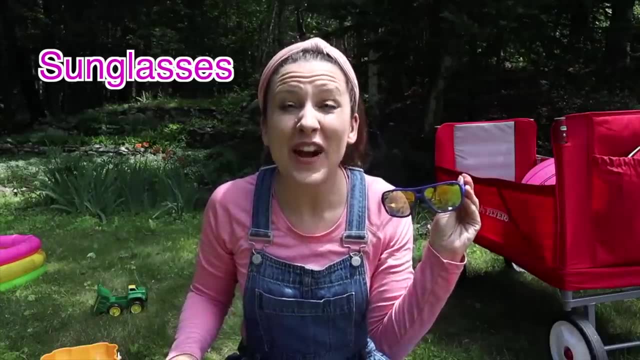 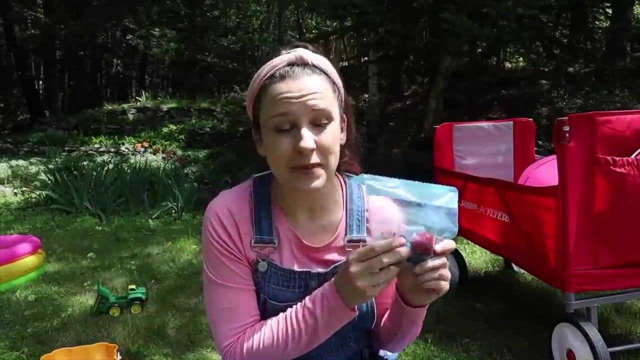 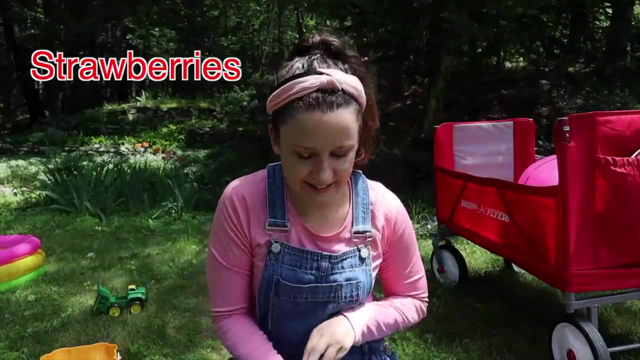 Sun glasses. Yeah, It's nice to wear sunglasses at the beach because the sun is so bright, But bright. The sun is so bright. I like bringing snacks to the beach. Guess what I packed for the beach: Strawberries And b-b-blueberries. 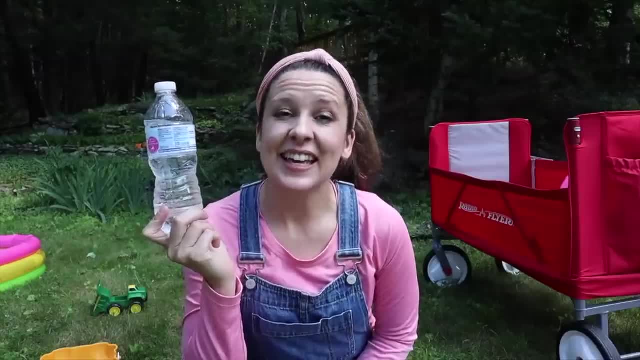 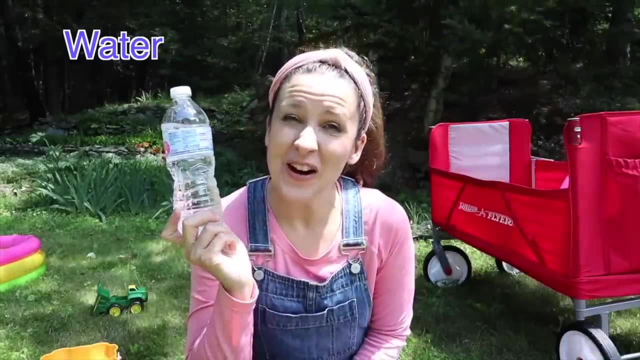 Wow, Do you know what this is? It's water. Yeah, This is another one of the most important things to bring to the beach: Some water, so you don't get dehydrated. Yeah, you drink a lot of water at the beach. 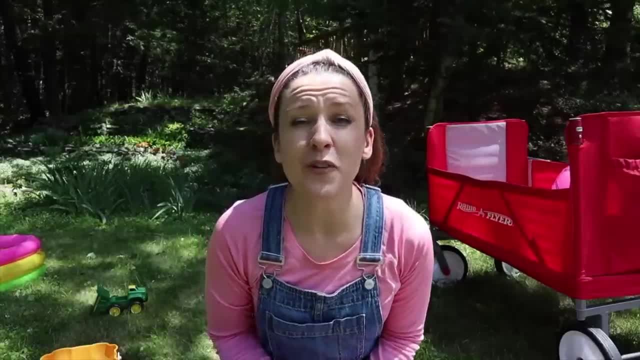 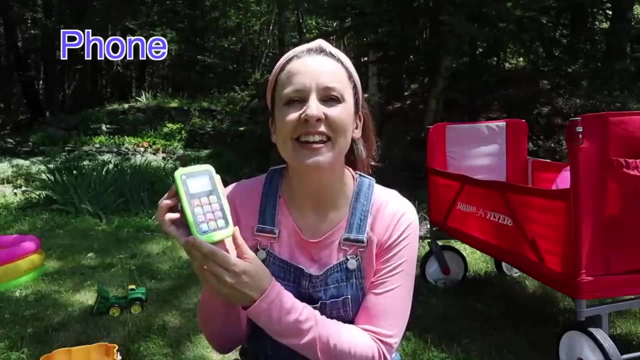 Water is so good for you, Maybe you should bring a phone to the beach. This is a toy phone, Turn it on. turn it on. turn it on. Hi, is Elmo there? Hi Elmo, What are you doing? 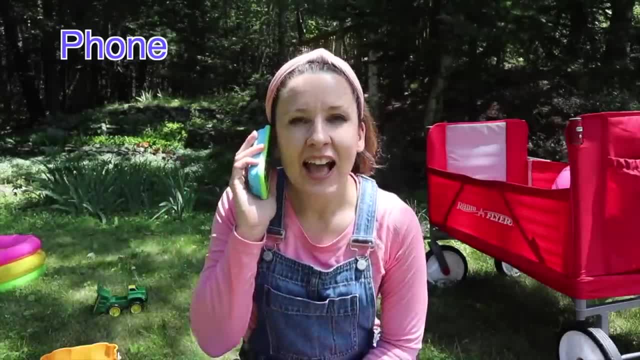 You're at the beach. Wow. Do you know what this is? It's a b-b-b-bucket. What letter do you think bucket starts with B-b-b-bucket. The letter starts with B- B-b-b-b-bucket. 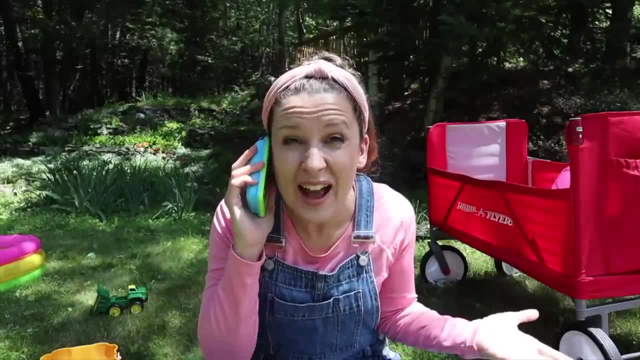 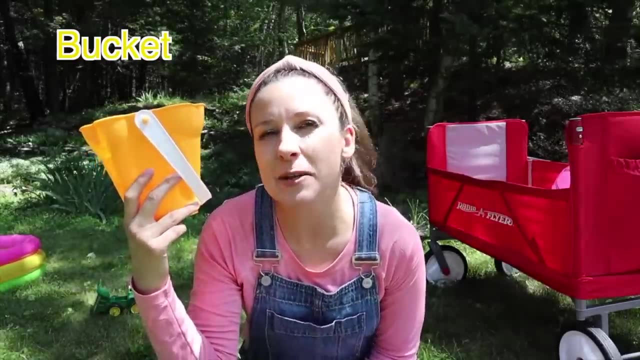 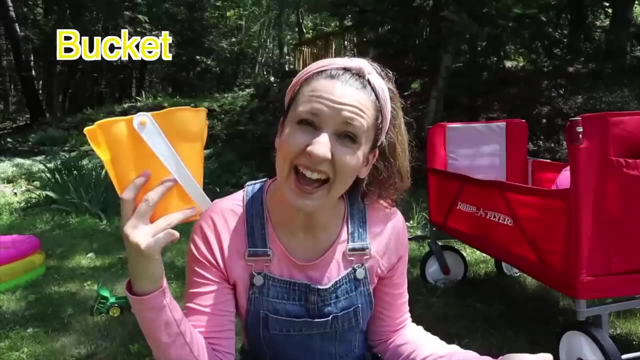 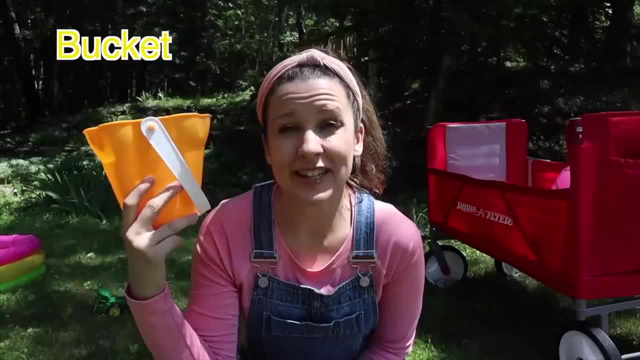 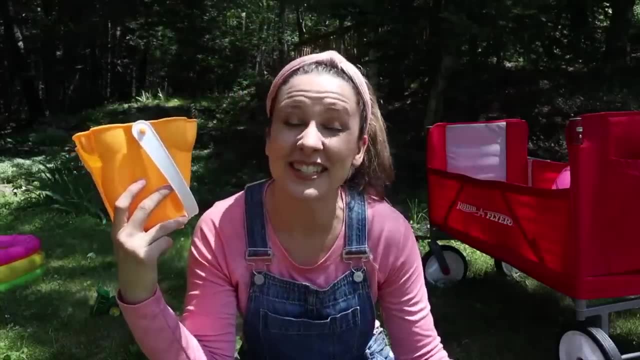 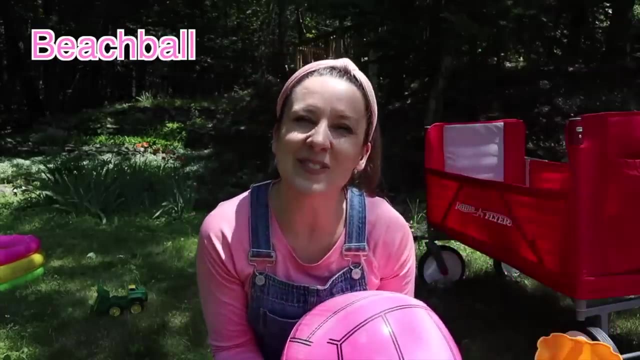 Wow, You can make sand castles with buckets. Some other fun things to bring to the beach are sand toys like shovels and rakes. Yeah, It's fun to dig in the sand. Dig, dig, dig. It's fun to bring a beach ball to the beach to throw and catch and play games with.